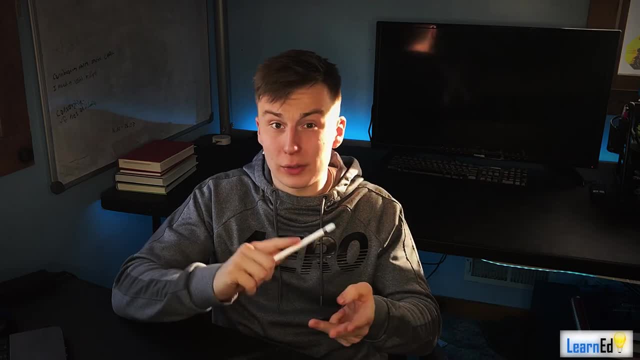 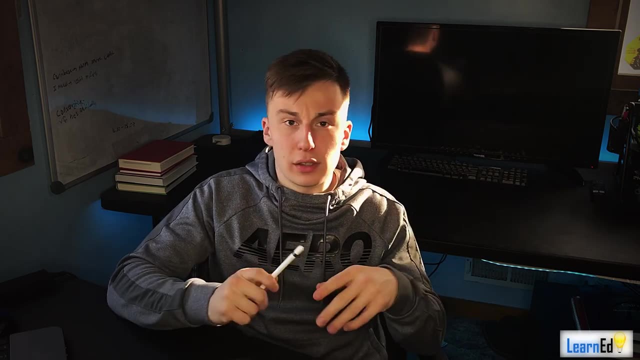 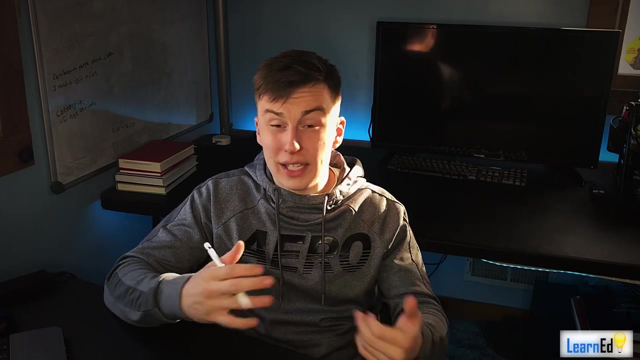 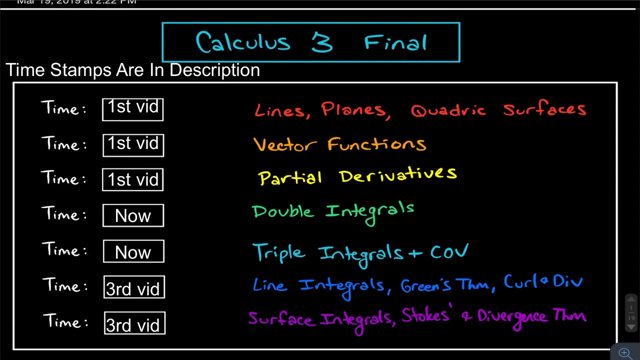 In this video, that being, you know so, double integrals, triple integrals and change of variables. And in the next video we'll be doing all the vector calculus stuff which is going to be, you know, Green's theorem, Stokes' theorem, line integrals, surface integrals, all that stuff. And you know, that way, this video will hopefully only be like an hour, an hour and a half long. Alright, so, without further ado, let's get into this video. So in the last video we did, you know, lines, planes, quadric, surfaces, we did vector functions. 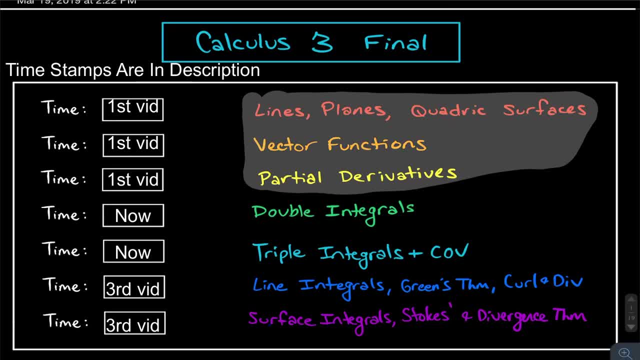 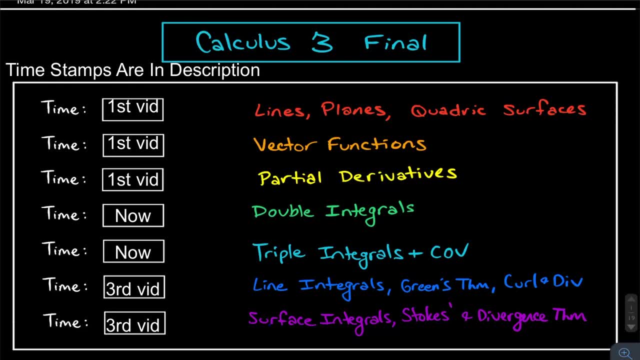 and partial derivatives. so Lagrange multipliers, we did max and mins, all that good stuff And that was kind of all the derivative stuff. Now we're going to get into the integrals. So we're going to do double integrals and triple integrals with change of variables technique Okay. So we're going to do all that stuff in this video. So we'll go through spherical, we'll go through cylindrical, we'll go through polar and then hopefully you guys will have a really, really good understanding of multiple integrals. 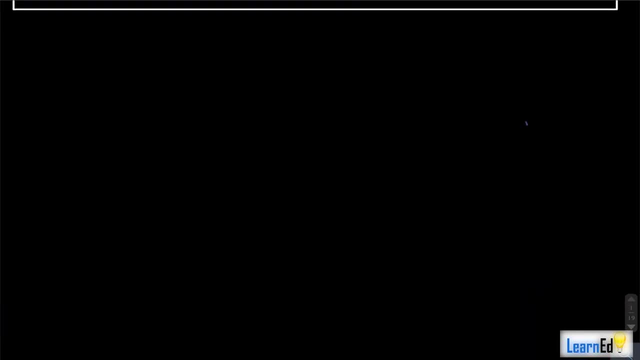 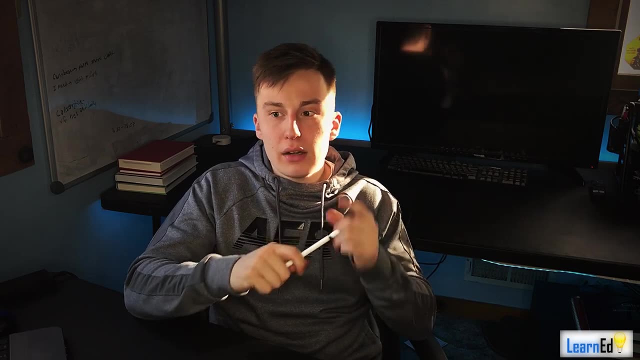 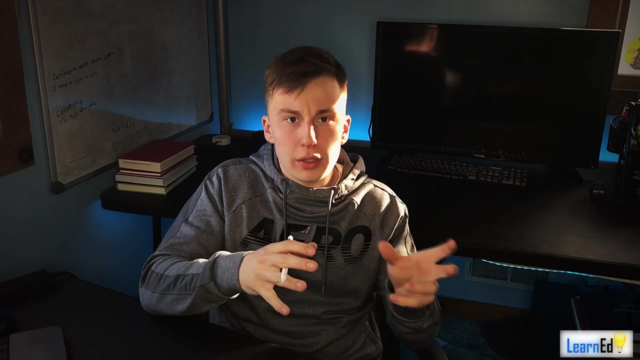 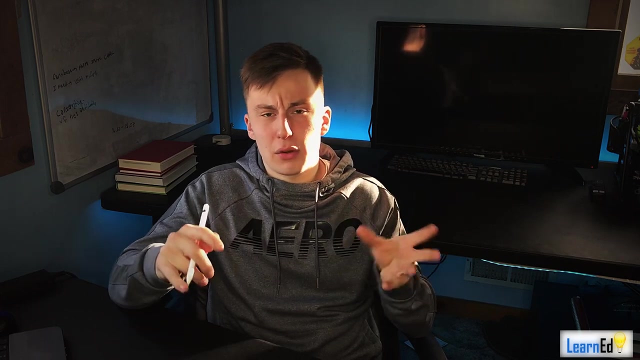 Okay, So before we actually get into our first problem, I want to talk to you about something that I really had trouble with doing- multiple integrals- And that was that I didn't understand. you know, sometimes we could use a double integral to find area or volume, and I couldn't understand. you know, what was a double integral meant to find. Was it volume, Was it area? And you know, was a triple integral finding the volume, Or was it finding this thing that my calculator professor called a hyper volume And that really, really confused me. 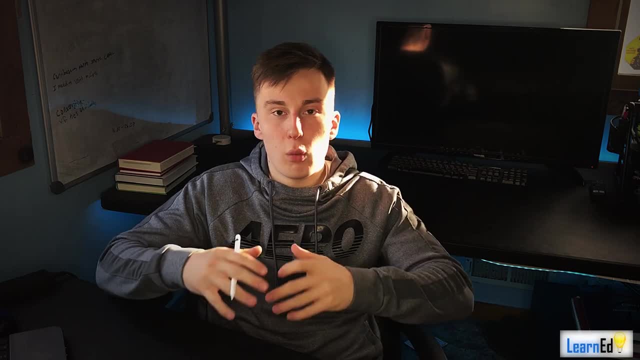 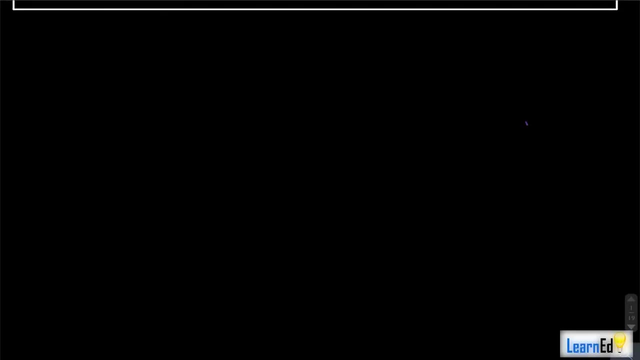 So I want to go through quick and just kind of talk about what a double integral actually would tell you and what a triple integral will actually tell you. Okay, so to give you an idea about what these things actually do, First off, when you have a double integral, a double integral finds the volume. Okay, it does, because a single integral finds the area. 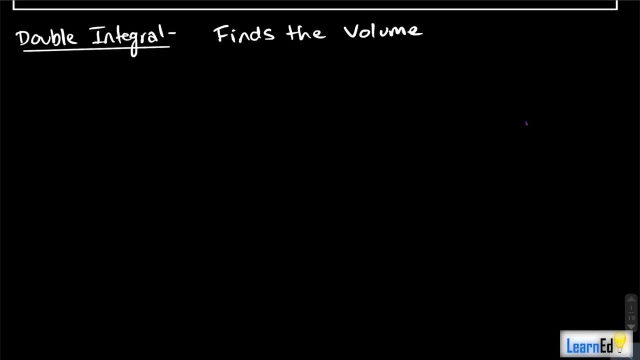 Okay, but here is the key thing that you need to understand: If you were to do a double integral and your surface, the top of your surface- is what your integrand is. So, whatever your surface is- x, y, z, whatever your surface is or whatever is on top of here- and you're integrating that over maybe some rectangle in the x- y plane. 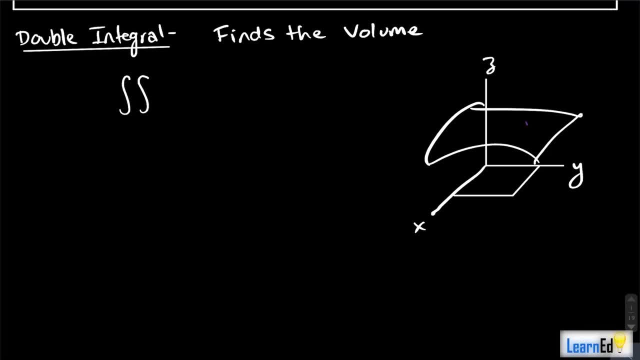 Okay, this surface, whatever function, z as a function of x and y, that is what goes right here in your integrand. Okay. but if we make this integrand one, okay, so we just make it one and we have to add a da on the other, on the end there. 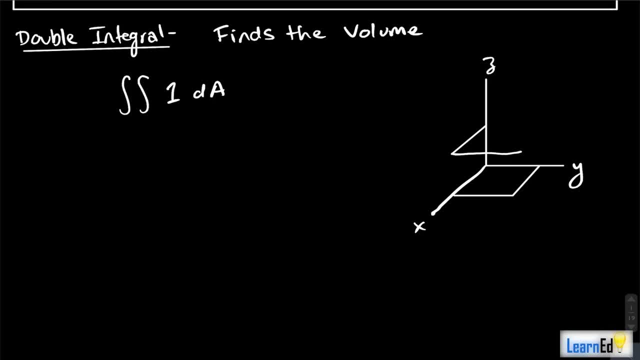 You just get a box right In this case because we, like I said, we're integrating over, like this rectangle, in the x- y plane. Okay, you are basically finding the volume of this box. Here's the thing, though: This box has a height of one. We know that volume equals length times width times height, And if height is one, we just get a box. 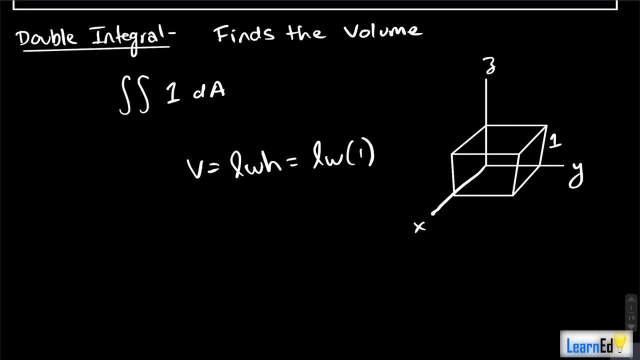 Well, length times width, in this case, right when height's one. So that's the area That's going to represent. what we find here is going to be the same exact thing as the area in the x- y plane. Okay, when we have a, our surface is just one. Okay, and you can actually kind of draw a parallel to two single integrals when talking about this. 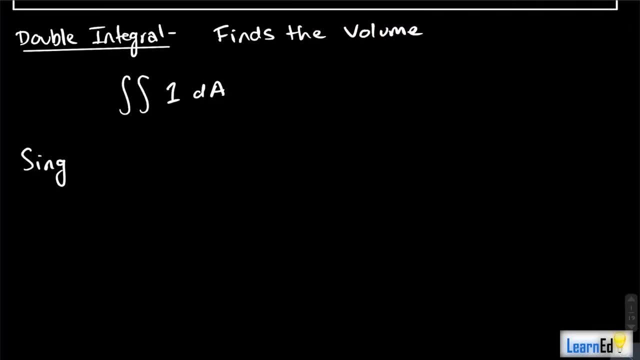 If we you know the job of a single integral and kind of going a little bit out of order here, next stop is triple integrals. A single integral finds the area- Right, It finds the area. But if you have like, so let's say, you have the single integral of like x squared dx, right, Whereas that x squared, like with double integrals, that's your surface, Okay, But in with a single integral, this is your curve that you're integrating under Okay. 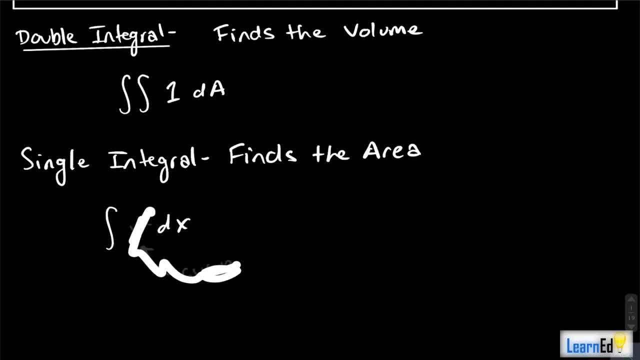 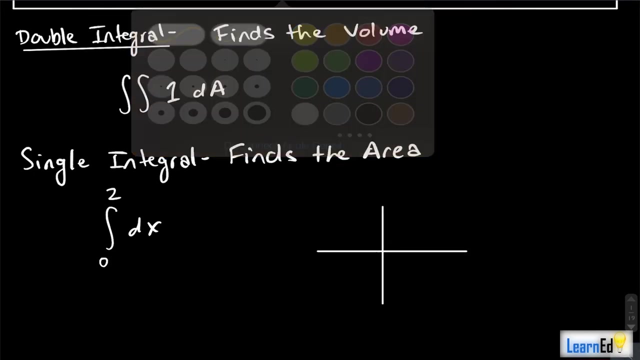 Now take that curve away. What are you integrating under? Well, that's just so. let's say you're going from zero to two, Okay, If you just have dx. okay, and sorry, that's a three-dimensional thing. I'm talking about two dimensions here. Okay, We just have dx. That's a line with height one, Right. 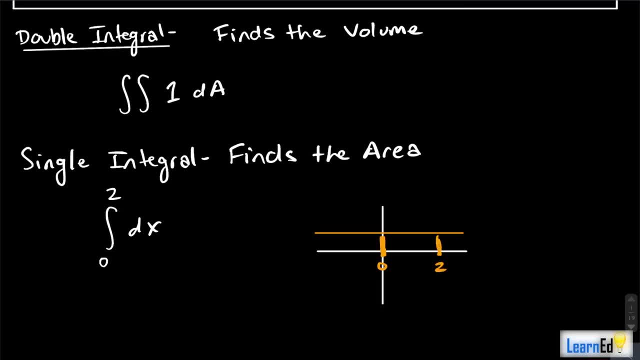 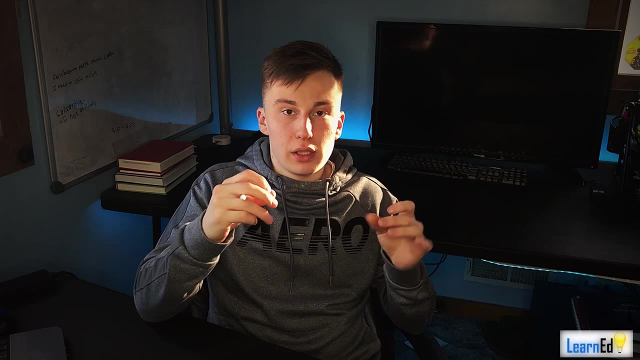 And if we're going from zero to two, all that's finding is, I mean, essentially, the length of this line, which is two, Right? So it's going for finding this kind of this one-dimensional measurement, right? So just this length of the line to an area in two dimensions, when we just have an integrand of dA. 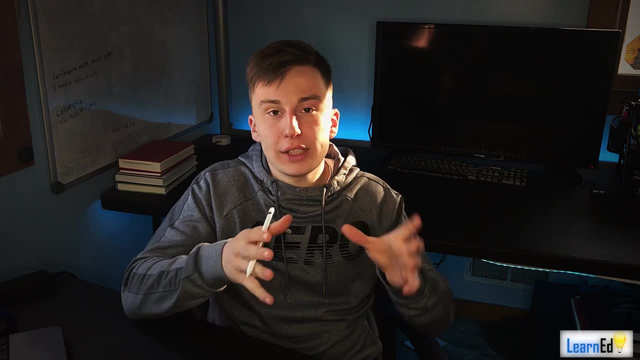 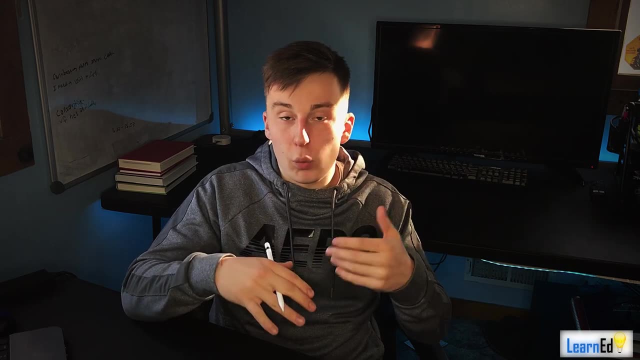 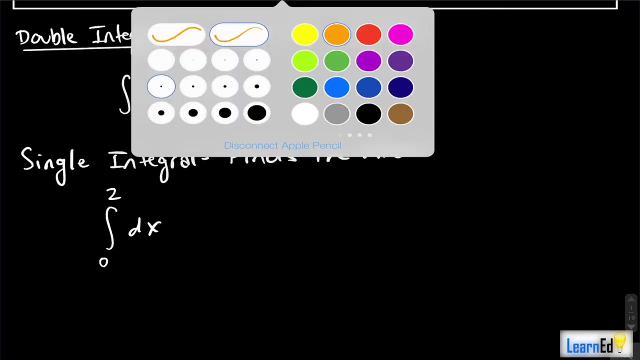 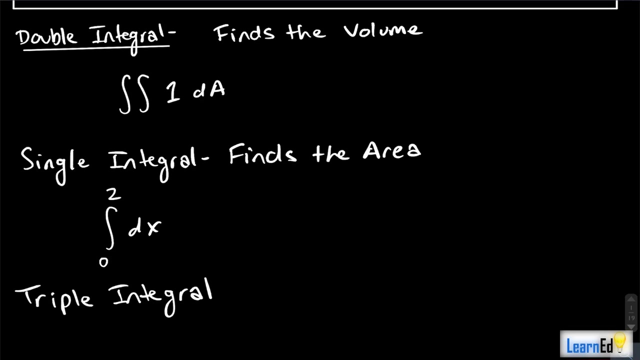 And similarly with a triple integral. if we just have our integrand dv, you can think of it as the same exact thing. So we're, in a sense, we can find the volume that way. Let me show you what I mean. Okay, So think about this in the same way that we just talked about our triple integral and our single integral. Or, sorry, think about the triple integral in the same way we just talked about our double integral and our single integral. Okay, 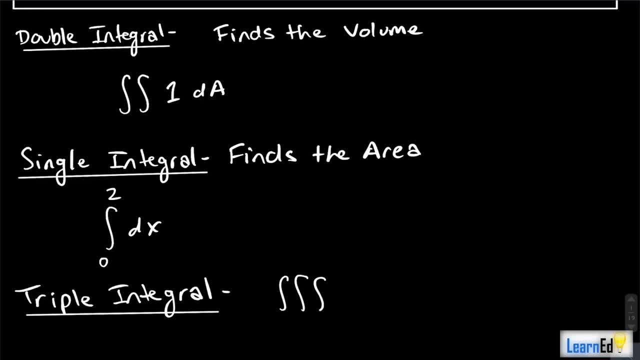 For our triple integral generally, what we have is: we're integrating. I think they like to use, like E as the solid that you're integrating over. If you have some function of x, y and z here, Okay, 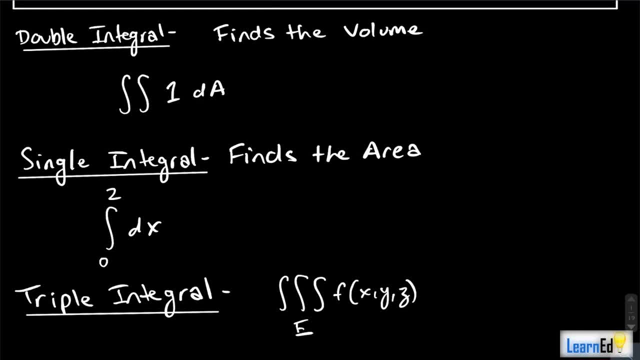 This is some four-dimensional- I guess you could call it a surface, I don't. I don't, I mean four-dimensional thing. Okay, That you're, that you're going to be integrating over, Okay That's, that's kind of like. 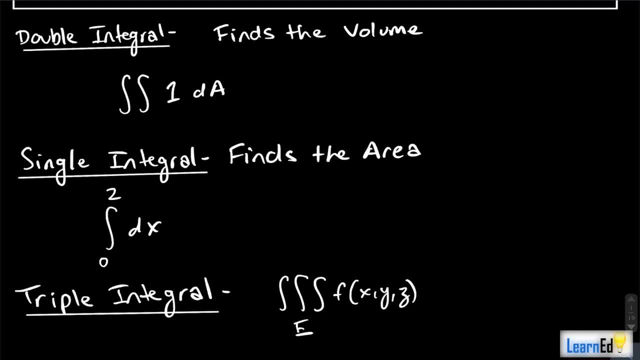 it's it's not, you're not going to be able to visualize it Right And your integrand is dv. So here, when you actually do this integral, what you get is a hypervolume. Okay, Because the job of the triple integral is to find the hypervolume. 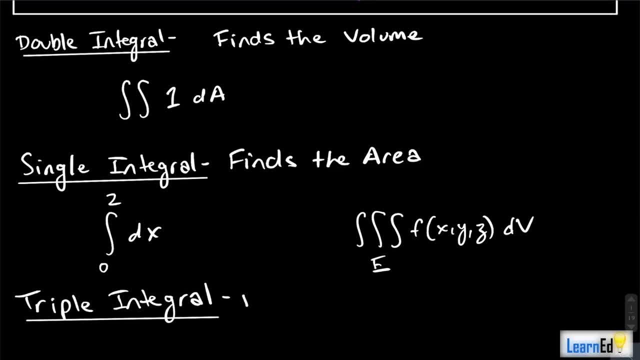 And that has applications like you're. like what's a hypervolume? It has other applications And I believe you know you could do some things like density measurements or something like that. My teacher always referred to it as hypervolume. 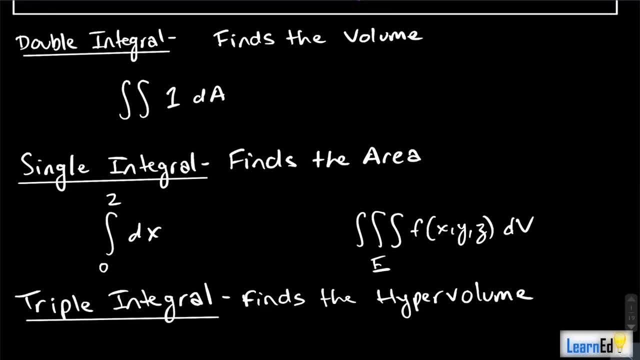 But you know it's really not. I mean, you're not going to have to know any of that, But what you will have to what, what, what will kind of make more sense to you is when you take away this function. 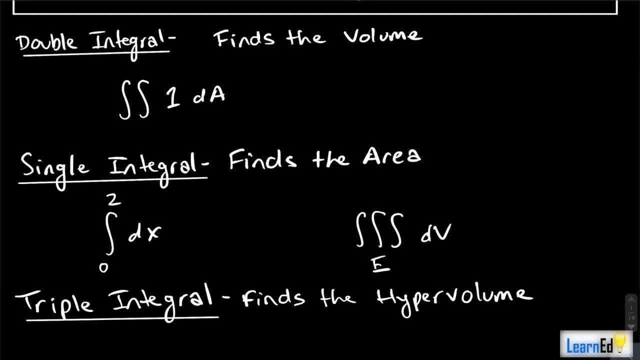 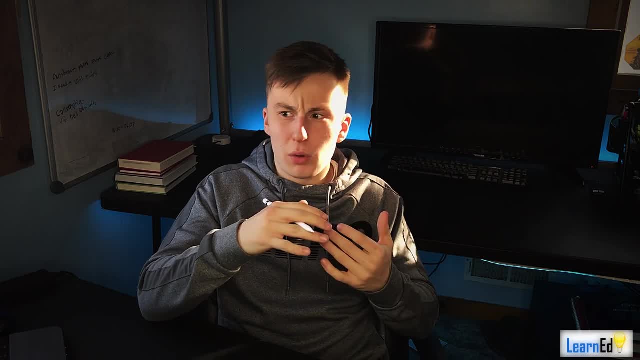 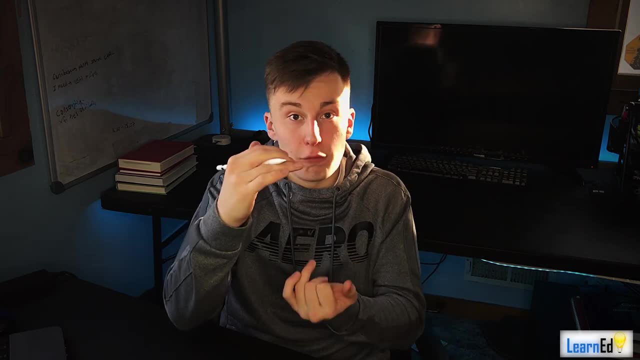 and you're just integrating over dv. now you're just finding the volume, Because that kind of extrusion into the- if that's a word, I don't know if that, that expansion into the fourth dimension, is only a length of one. 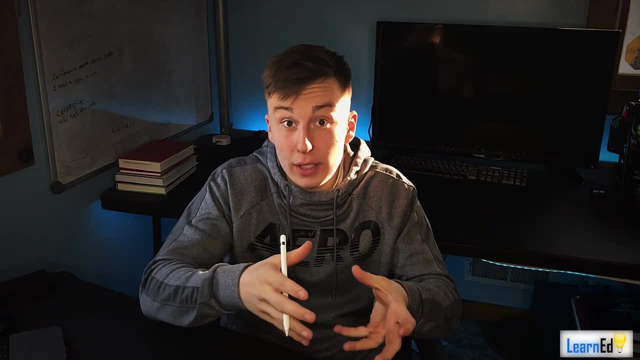 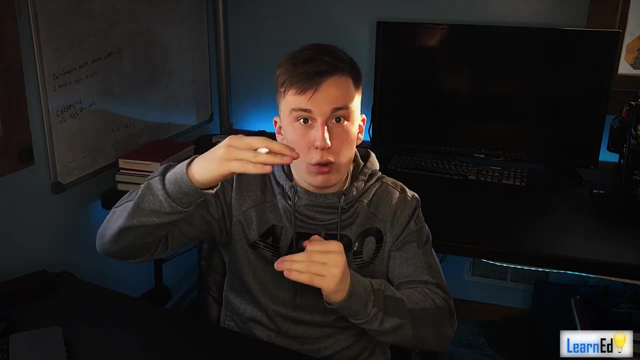 Right, So that means you're just essentially finding the volume, Like with a double integral, your, your extra dimension, right into the third dimension. your height was one, So you were just finding the area, Because volume equals length times width, times height. 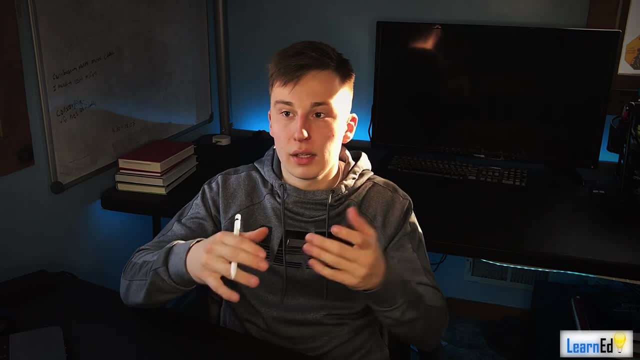 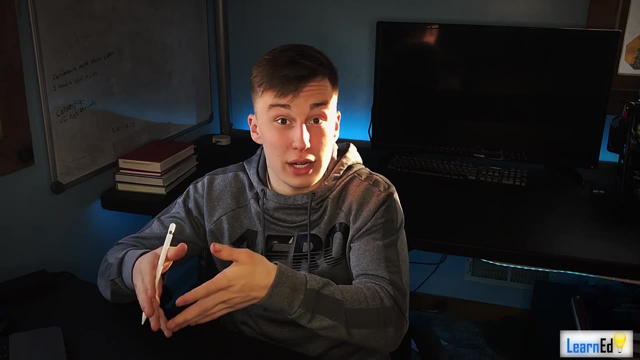 Right, It's the same thing. Let's say, our hypervolume equals length times, width times, height times another dimension which we'll call x. Okay, When we expand into that fourth dimension, but we just have an integrand of dv. 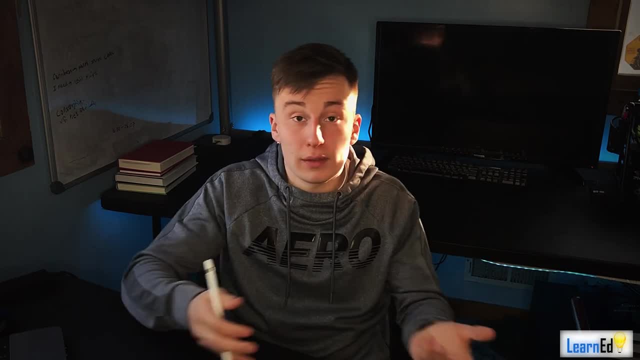 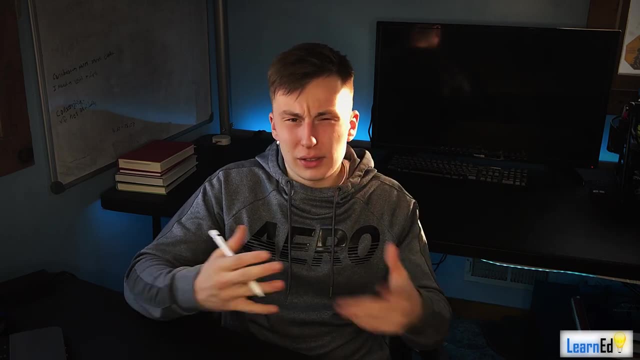 well, that's just one, x is one, So we get a volume, Length times, width times, height. Okay, Hopefully that makes sense. I didn't want to go over that too quick, So you know, hopefully you were able to kind of stay with me here. 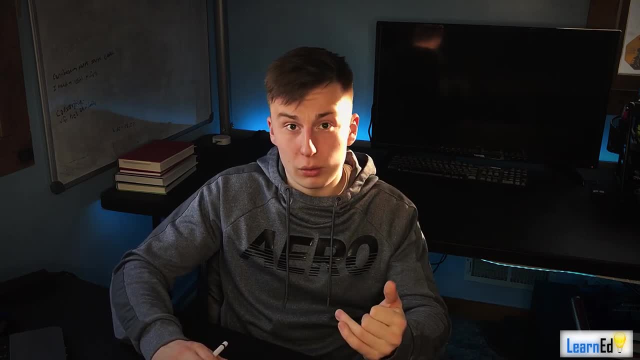 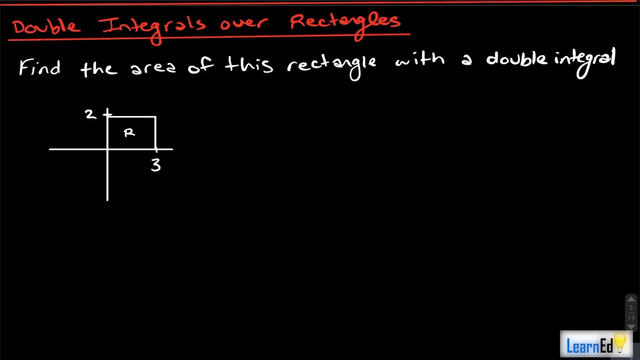 But I'm going to be reinforcing this in the problems that we're about to do, So stay tuned for that. So let's- yeah, let's- get into this here, The first thing. we're just going to start off easy here. 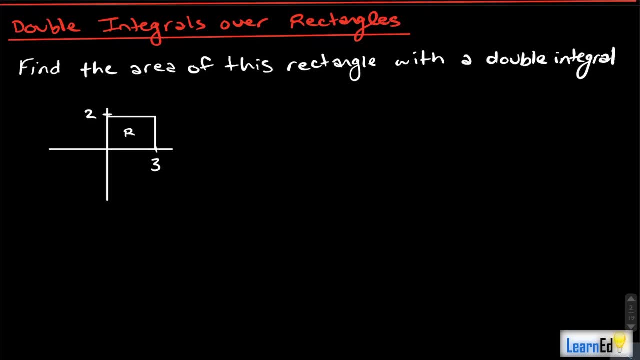 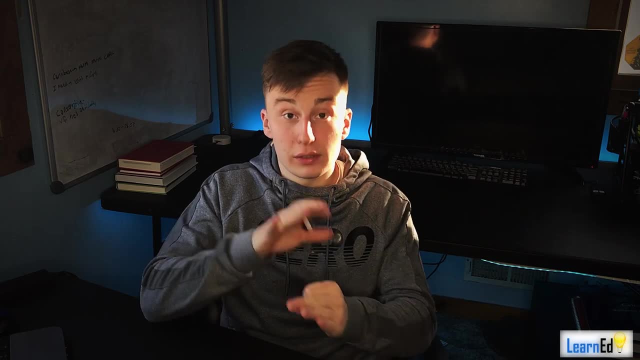 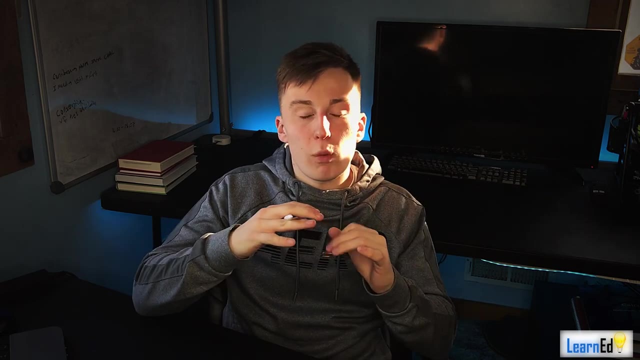 Okay, We're going to talk about double integrals over rectangles. Okay, So we're going to find the area of this rectangle with a double integral. Now, remember double integrals, they find the volume. Okay, So it's going to be equivalent to finding the area if our integrand is just dA. 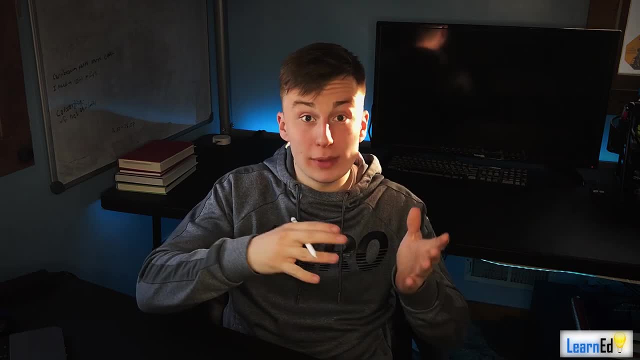 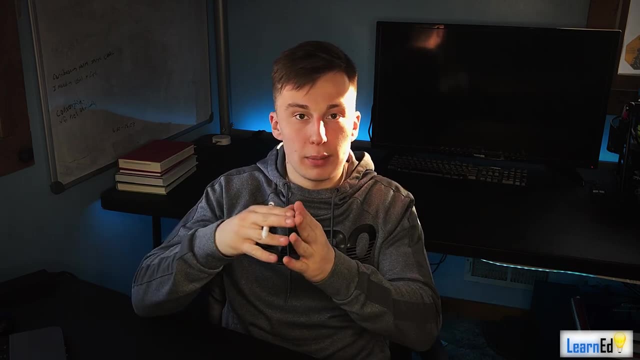 Okay, Because that means that one of our so volume is length times, width times, height. Our height here, if our integrand is dA, is just going to be one Right One, dA, So the height is just one. 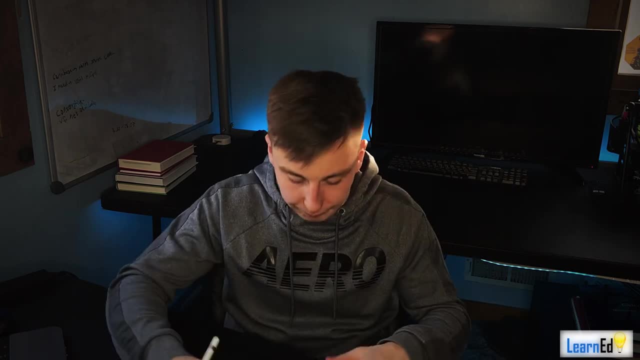 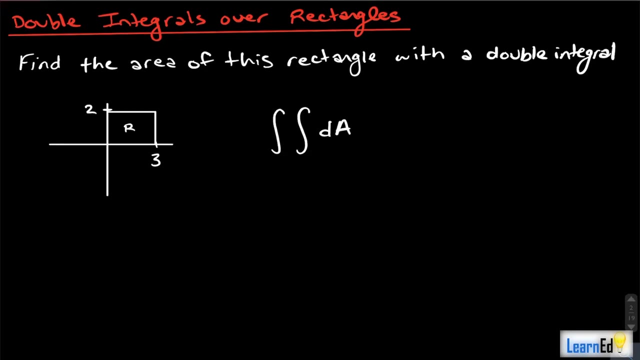 Okay, Because that's our, that's our surface, as I talked about before. Okay, So we're going to have the double integral of dA. Okay, Over this region R. Now, what are our bounds? Okay, Well, our bounds are really nice here. 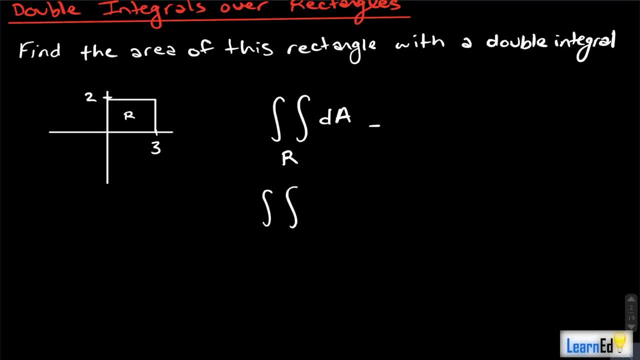 Okay, On the dA right, this can be rewritten as dxdy. Okay, So our inter, our inner integral, is going to have bounds of x. So on the x-axis we go from zero to three, And these are straight lines going up and down. 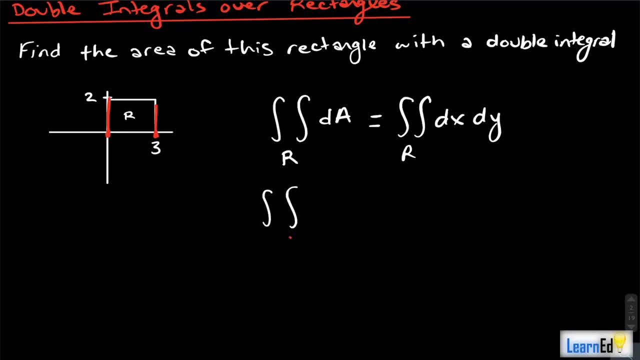 So we don't need to worry about any curves or anything like that. Okay, So we have zero to three. Okay, Of dxdy. Okay, So those are our x-bounds. Okay, We know that because that's our inter, our inner integral, and we have a dx there. 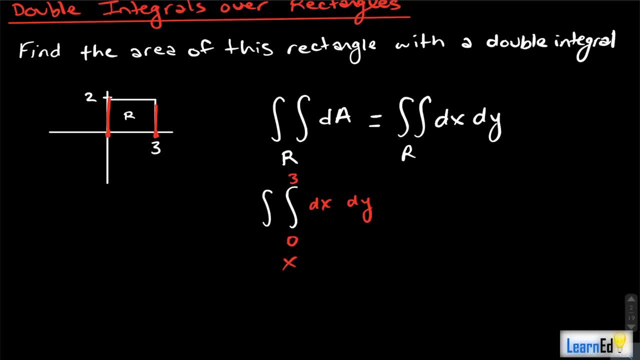 So I know some people like to put like an x under here or something like that. I don't really care for it, just because it's extra work. But you know, here we go. We have zero to two as our y. 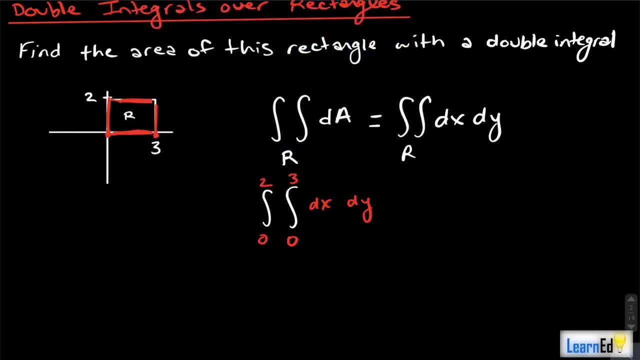 Okay, So now we just evaluate this right, So we can first do our. I mean, we can separate these two integrals. actually, We can take this integral and do this thing separately, because this dx and dy are being multiplied together and these bounds are not dependent on each other at all. 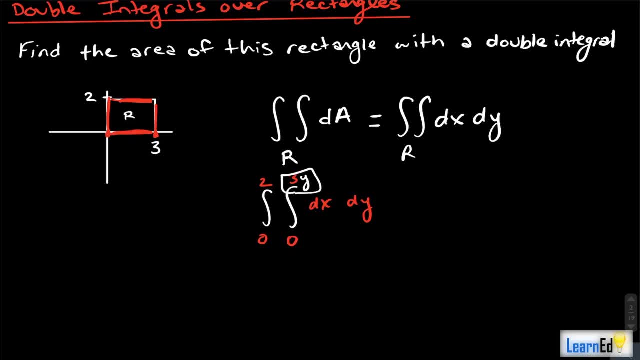 Like. this isn't like three y where you need to integrate this thing to get Yeah, To do your second integral right. That's not how this works, So you know. you may remember this from your Calc III class. This is the same thing as saying the integral from zero to two times the integral from zero. 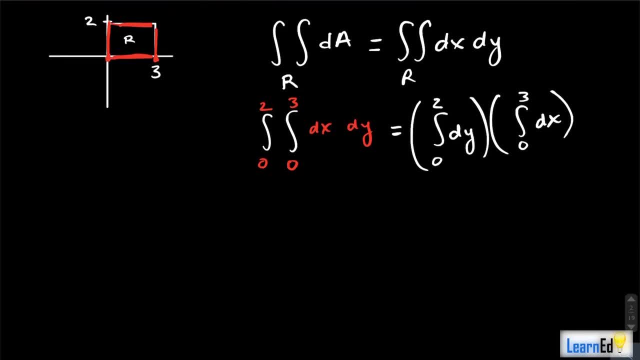 to three of dx. Okay, Same thing. So if we actually do this integral here, we get y evaluated from zero to two times x evaluated from zero to three. Okay, Okay, Okay, Good, All right, Perfect, All right. 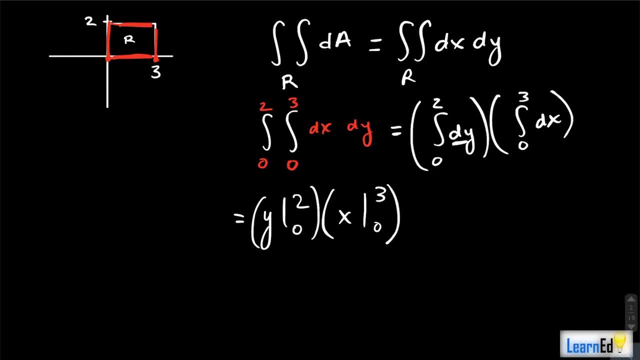 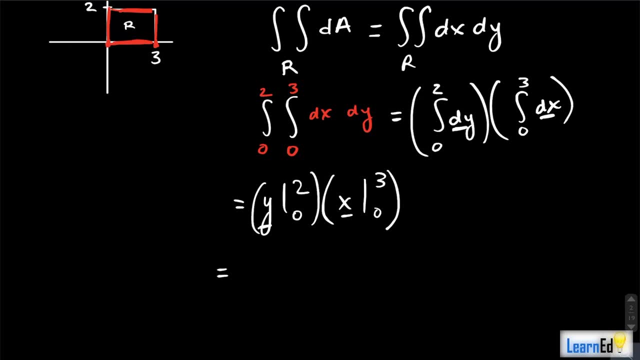 Good job, Thank you. Thank you All right, All right, Thank you All right, Okay, Okay, All right. right. the antiderivative of dy is just y and the antiderivative of DX is just X. okay, we're evaluating it from 0, or from 0 to 2. this is just 2 minus 0, and then 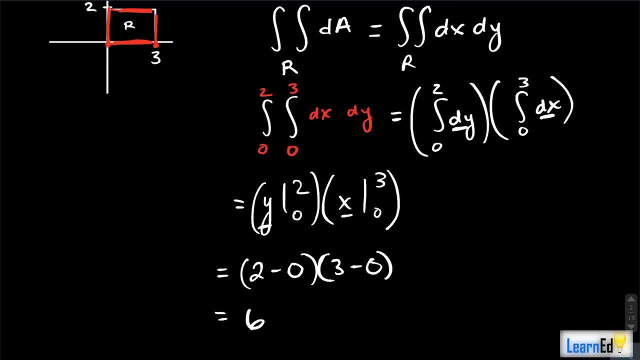 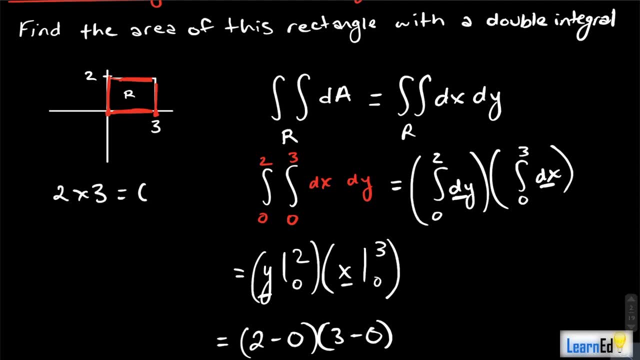 the X is just 3 minus 0, and that's just 2 times 3, which is 6, so you get an area of 6 which we can conclude. that's exactly what that is: 2 times 3 is 6, right? so that is probably the most complicated way that you'll ever find. 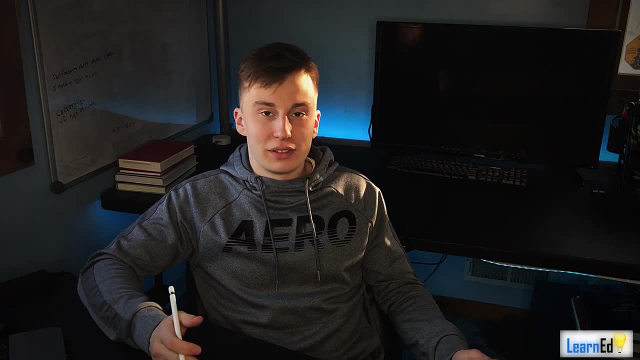 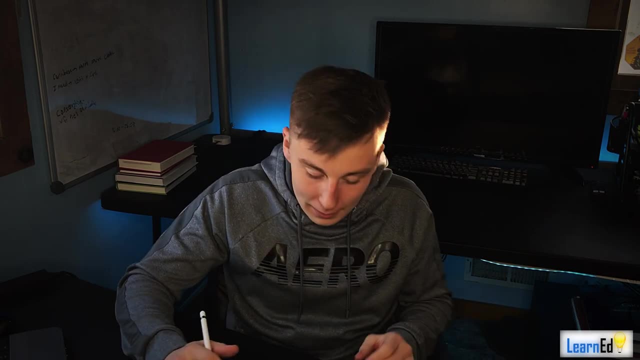 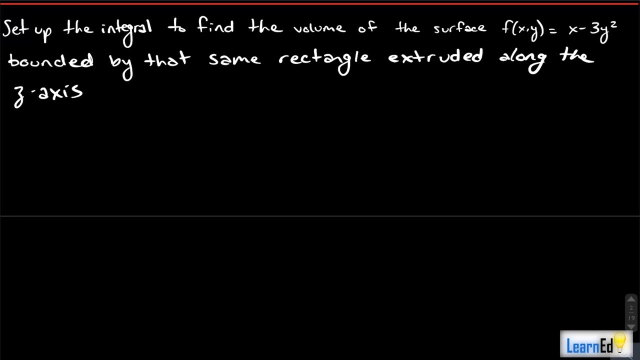 the area of a square, of a rectangle. but you know it, hope it, I hope it's helping you understand double integrals. at least that would be great if that this helps, right, I don't know. moving on, so let's next set up the integral, not now we're. 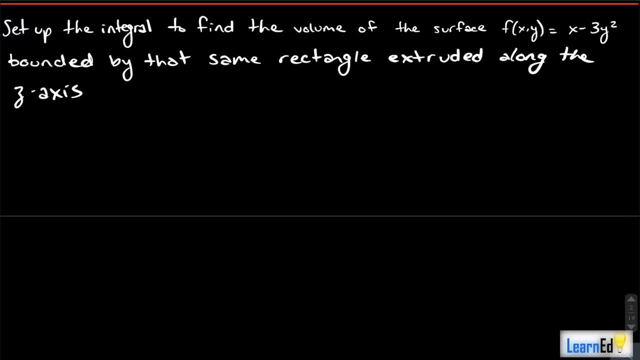 not gonna evaluate it because we're gonna be evaluating some tougher in the girls below and I just want to get the concept across of setting up an integral. so we're gonna set up the integral to find the volume of the surface. we have a surface F of X and Y equals X minus 3y squared bounded by that same. 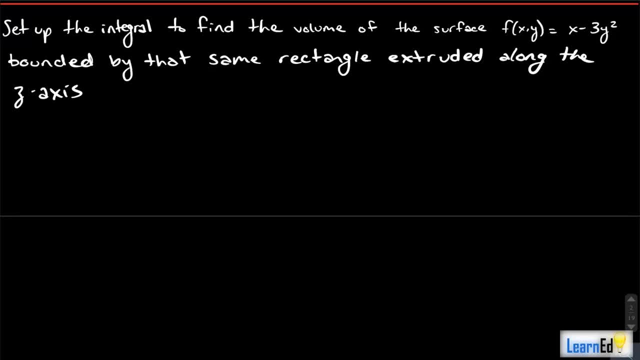 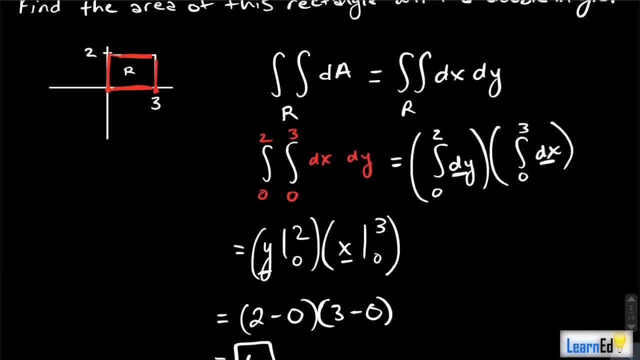 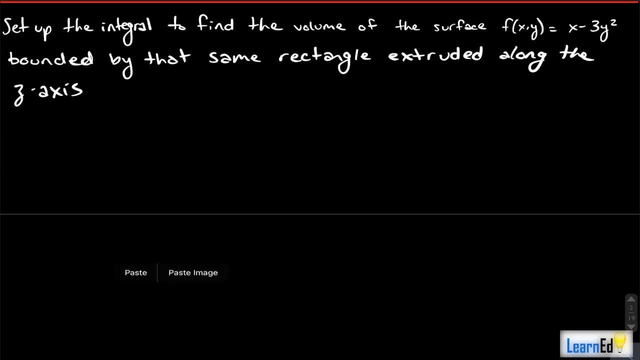 rectangle extruded along the z-axis. okay, so we have that same rectangle, right? so it's this guy, so we can actually. let's just copy this down. oh yeah, you guys aren't drawing on an iPad. that sucks, sorry, but what I'm gonna do. so this is: 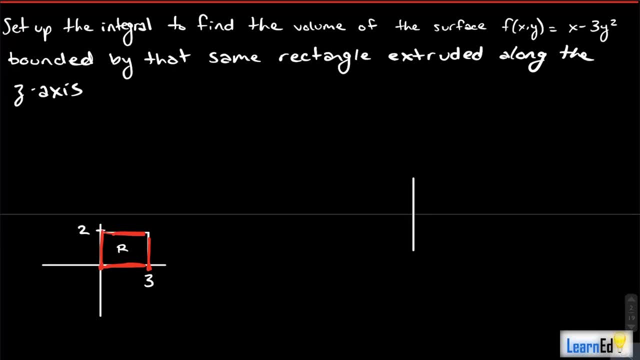 our visual. you guys probably aren't drawing on such a small screen, though, like or on such a small surface, so it's so hopefully be alright for you still. so we've X, Y & Z, and on X we're going over 3. actually, I'm going to draw this in red, yeah, so we've. 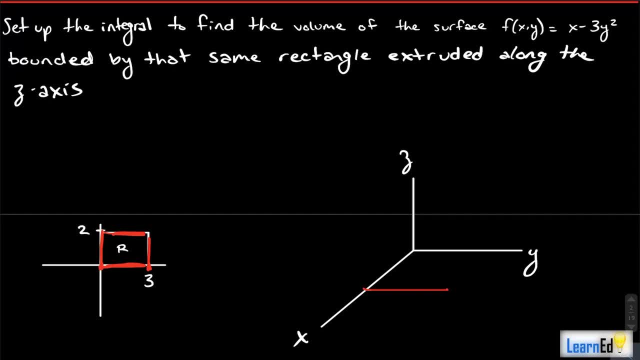 got 3 and here we got 2. okay, so this is 3, this is 2, and now we're gonna have some surface. I have no idea what X minus 3y squared looks like. if I look up I, if I examine them enough, I could probably figure it. 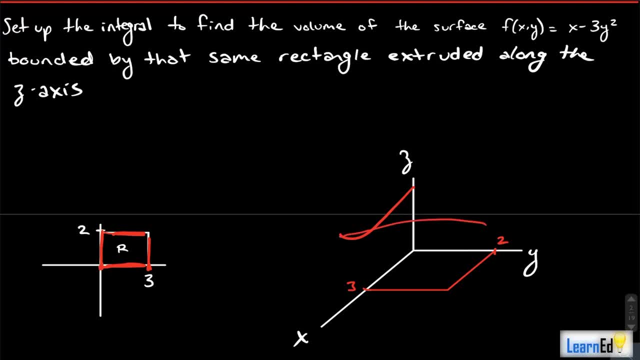 out, but it doesn't matter, really, I don't care. okay, we have some volume, what some? or some surface? let's say that this is F of X, Y, okay, and we can just still have the same bounds here, okay, but now, instead of finding an area, we're finding a volume. so you know, what we're gonna do is because our 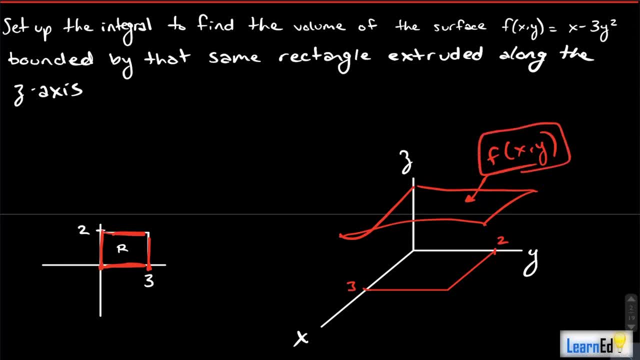 surface is no longer one. it's a function now. okay, if it was. if it was one, then we'd essentially just be finding the area right, like we did in the last problem, but now we're finding a volume. we have a surface that's not just one. 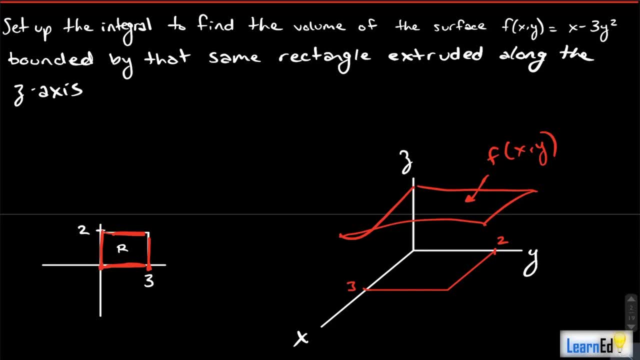 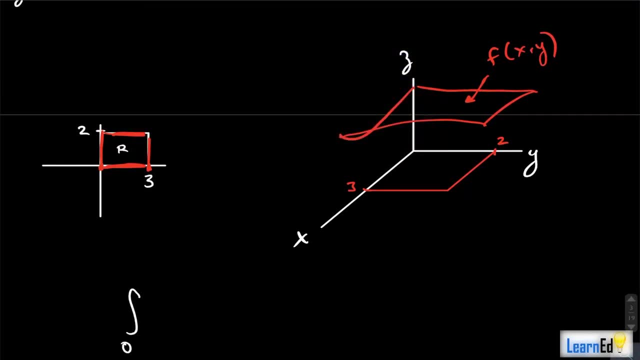 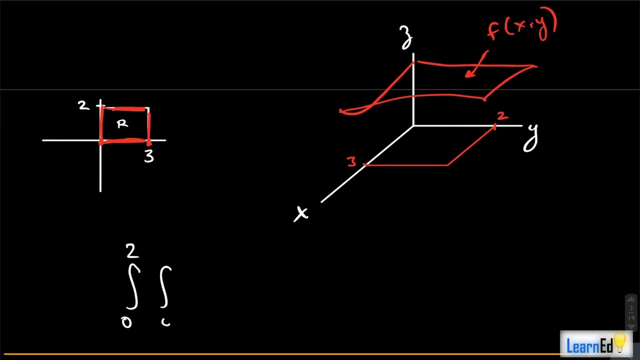 okay, so we have this guy and we can still. I mean, our bounds are gonna stay the same. we have an integral from 0 to. what did I use before I did my Y first? okay, so 0 to 2 and then 0 to 3, and 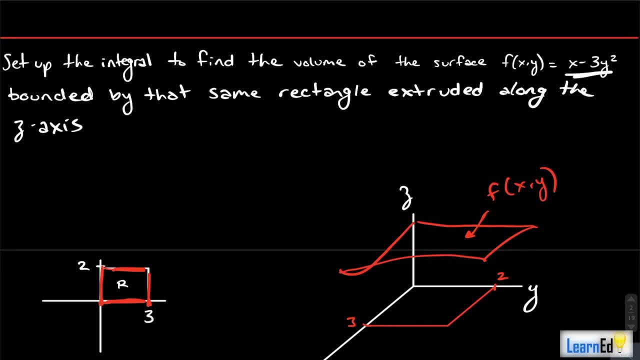 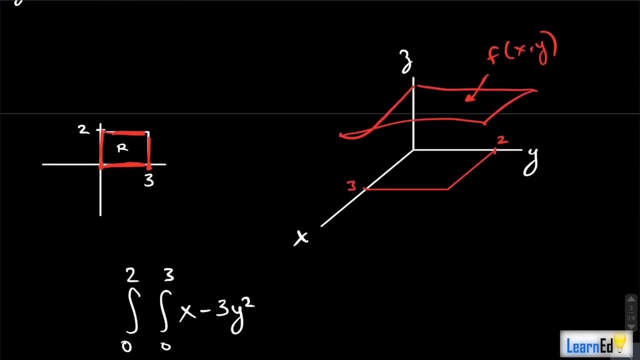 now we just insert our integrand, which is the surface right X minus 3y squared D, our inner integral, 0 to 3, that's our X bounds, so we have DX there. and then our outer bounds, 0 to 2, are our dy. okay so, 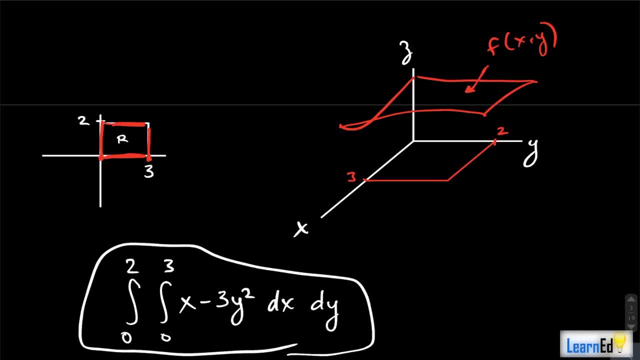 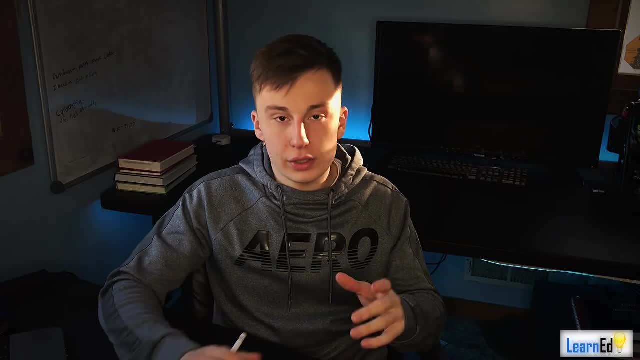 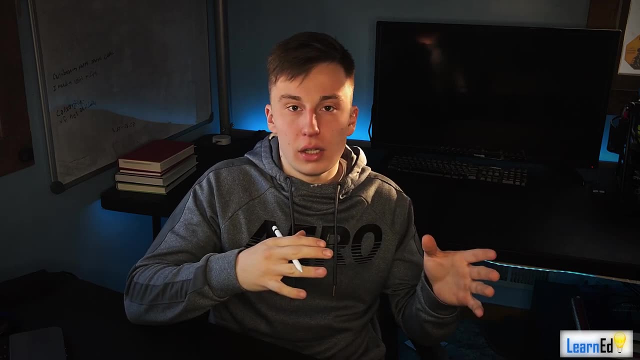 that's your integral, right there. okay, so it's. it's not the hardest thing in the world to just set up, if you just understand the concept of what a double integral actually does. right, let me rephrase that one more time. so, because if you're still lost, I don't, you know, I don't want you to stay lost for the 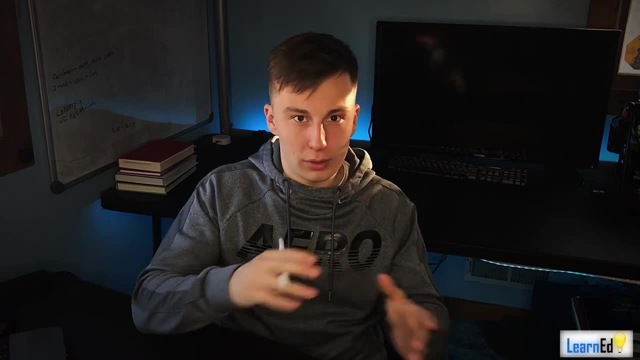 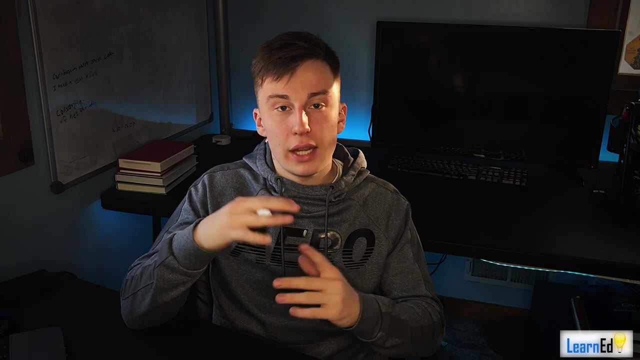 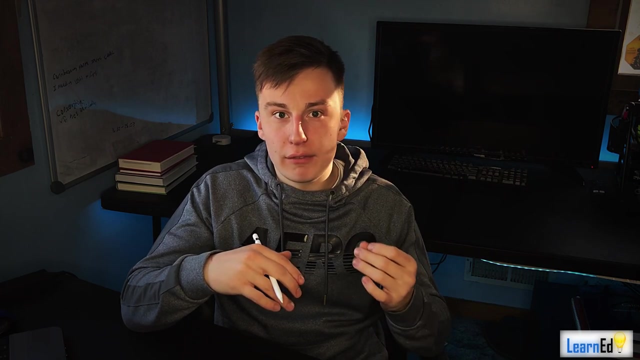 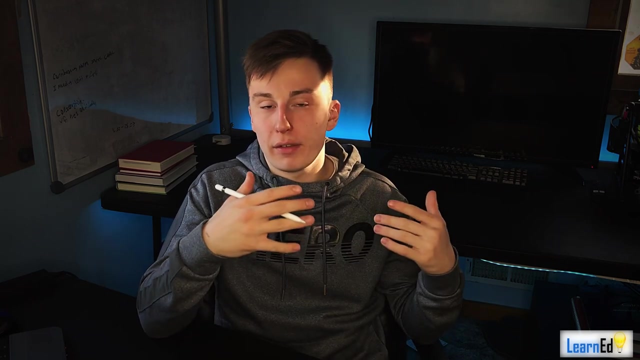 entire video. so so let's go over this once more. a double integral gives you the volume, okay, but if your surface is just one, it's tierra right. if the surface that you are integrating over is just one, that essentially is going to give you an area, because think of volume. 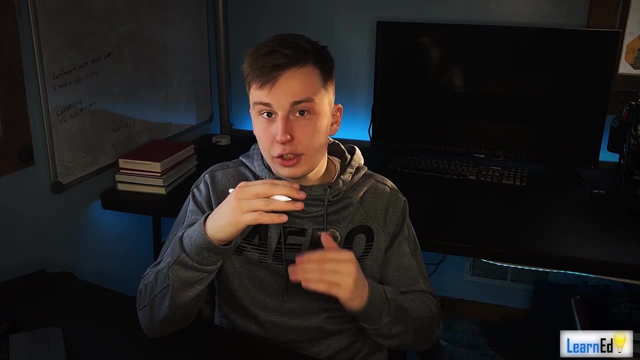 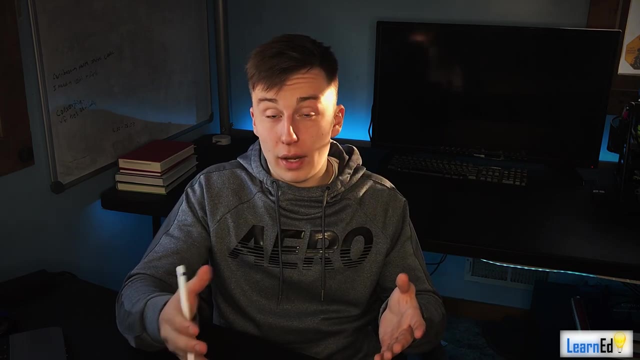 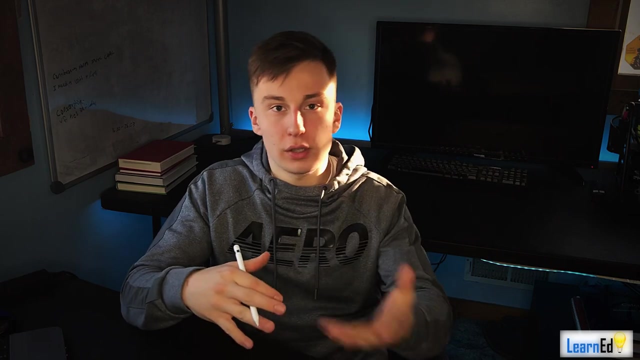 as just length times with times height, right, if your height is just one, you have a length times a width, right, which is an area? okay, that's an area. so if one which you know, you add the da on the end. that's why i was talking about da earlier. 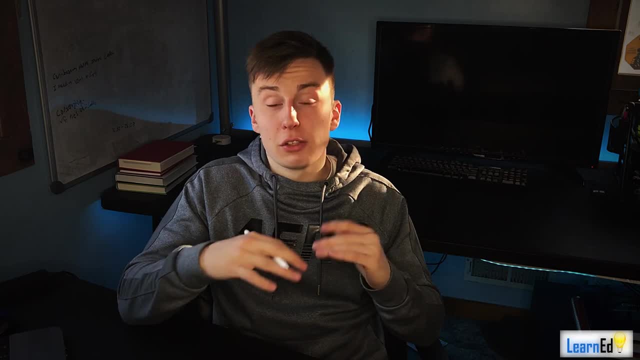 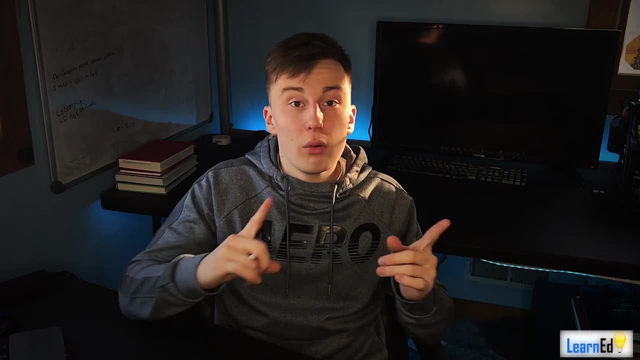 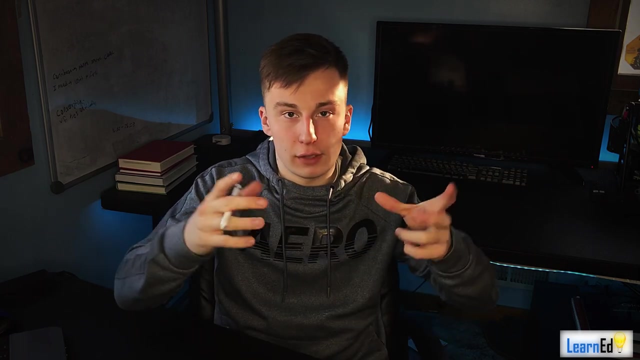 then you just are finding an area. okay, so that's what we did before when using a double integral to just find the area of that rectangle. now we're using it to find the volume under a surface, but, you know, still bounded by that same rectangle. so we're cutting that surface off, you know, with that, 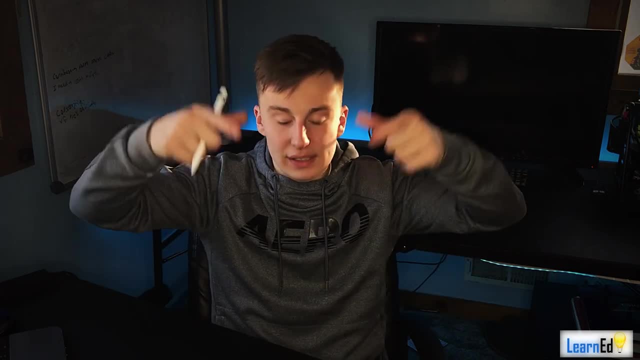 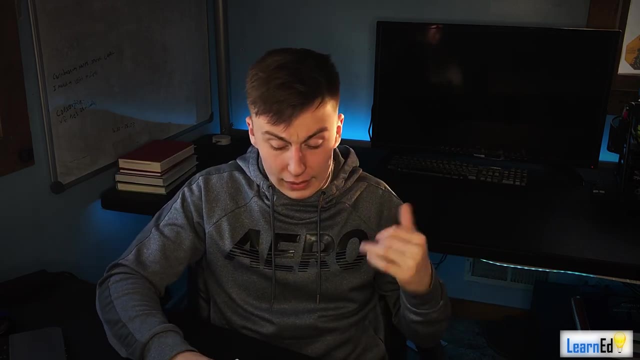 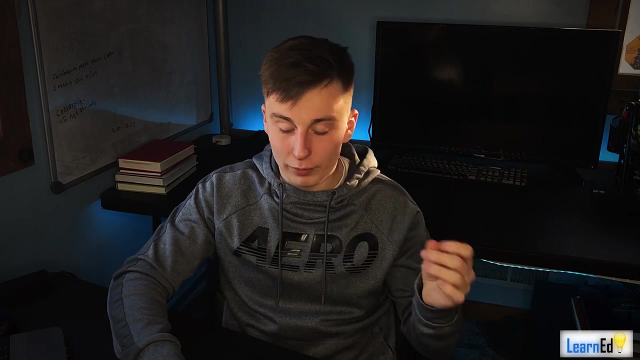 rectangle going up right where we can extrude that up into the in the z direction. okay, that's kind of what i meant by the that in the problem. if you got confused by that wording at all, okay, and you know that was really all we did there. so that's the idea with double integrals. okay, hopefully. 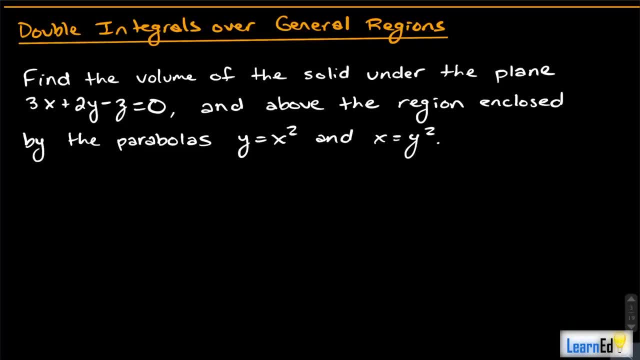 that makes sense. let's move on to the next problem now: double integrals over general region. so we're not gonna always have like rectangles, it's not always going to be really really nice. so you know, we're going to have some more general regions. so here we're, being asked to find the volume of the 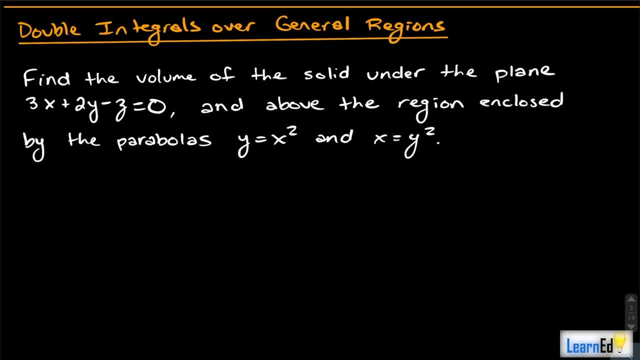 solid under the plane theta and we're going to have that volume of the solid under the plane theta. three X plus two, Y minus Z equals zero, And above the region enclosed by the parabolas, Y equals X squared and X equals Y squared. 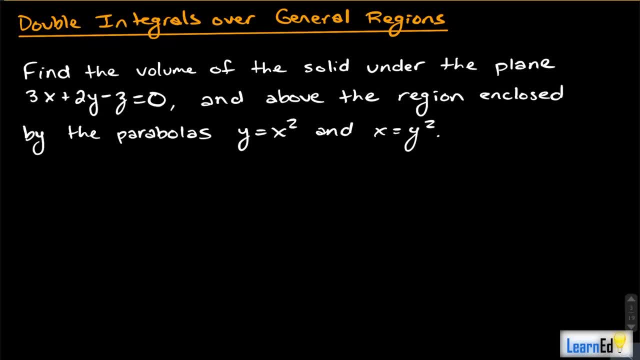 Okay. so first off, let's look at the two dimensional figure here. Okay, because like these are our bounds in the XY plane. Okay, so let's just draw out some axes. Okay, we have our X axis and our Y axis. 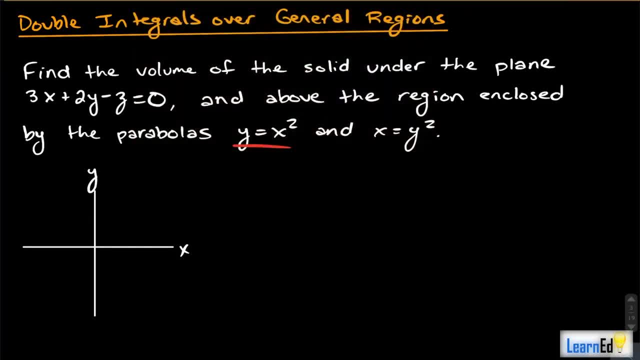 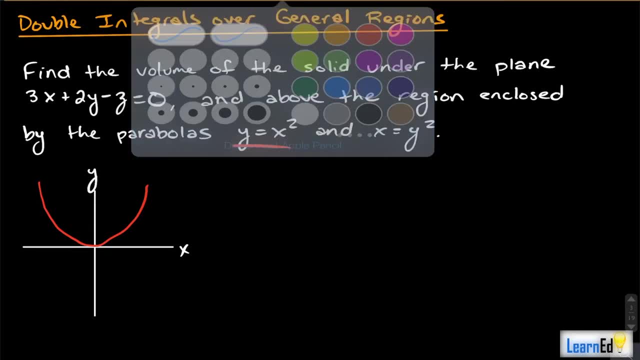 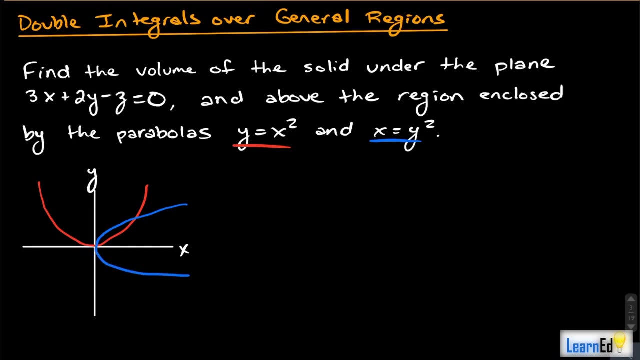 and we have two curves here. We have Y equals X squared, So we just have this guy here, Okay, and we have X equals Y squared, So it's gonna be that guy right here, Okay, the surface that we are, the, yeah, the. 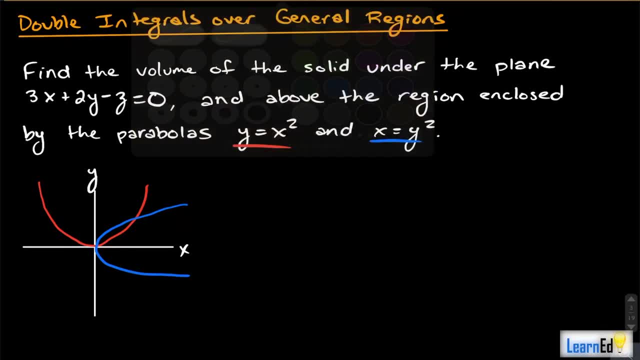 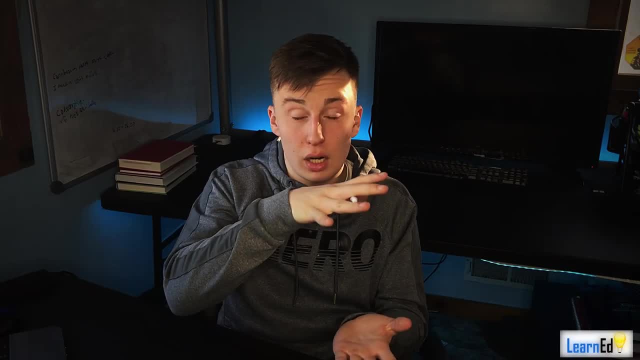 the region. that's the word that we are going to be extruding upwards. that's gonna be our bounds, right, That's what's gonna come into contact with our surface. our plane that's above, that is going to be that intersection, right there, okay. 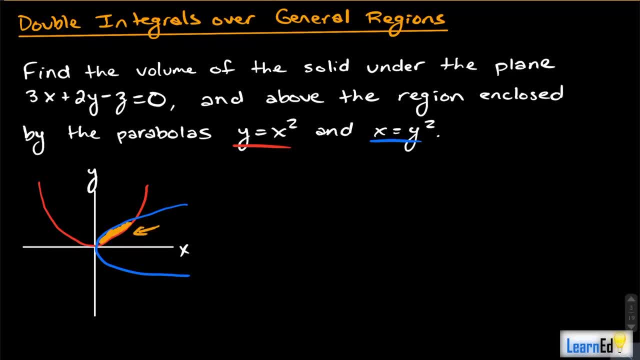 So that's this intersection right here. That is our region R, That's what we're integrating over, okay, So that's gonna determine our bounds, right, Because, remember, we set up a double integral. that's over R, right. 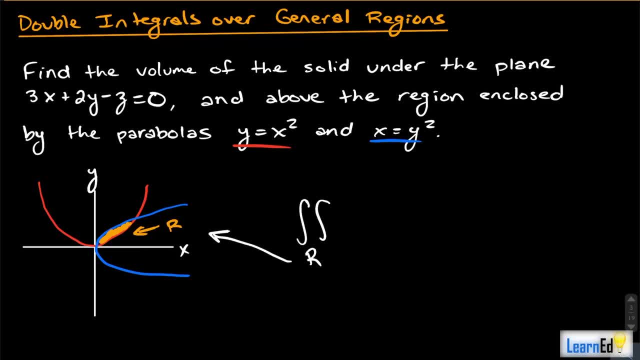 That's over our region, R, and right there you can see that R is this guy. Okay, so that's gonna set up our bounds, And then all we gotta do is just throw in our plane. okay, And remember that in a double integral. 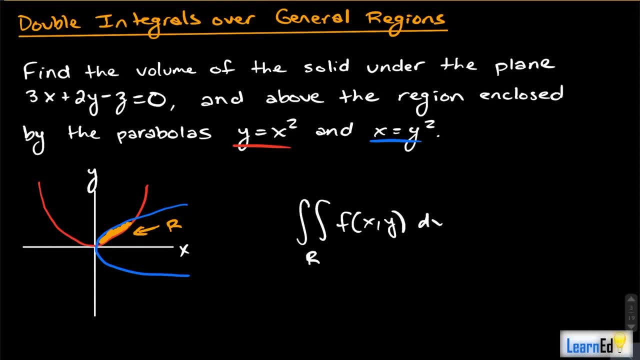 we have a function of X and Y, okay, And then you have, you know, DX, DY, whatever, DA. So what we need, I'll write DA first. I'll write DA for now, because I don't know which one we're gonna do first. 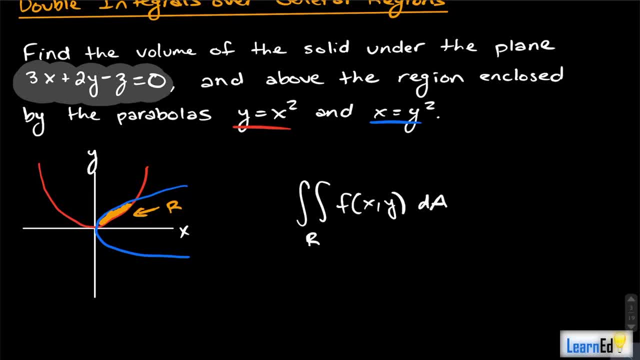 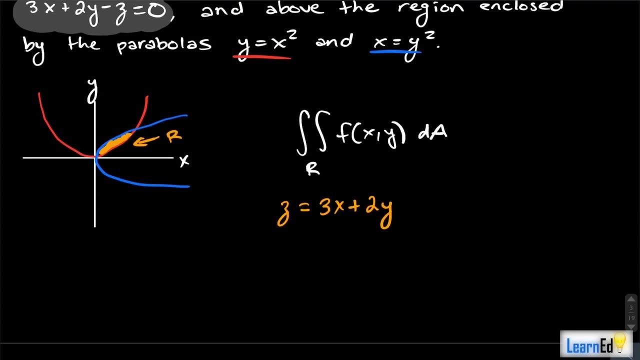 We need to express this plane as a function of just X and Y, So all we have to do here is just add Z over to the other side. So Z equals three X plus two Y. And there you go. Now you have your function that you can plug in, okay. 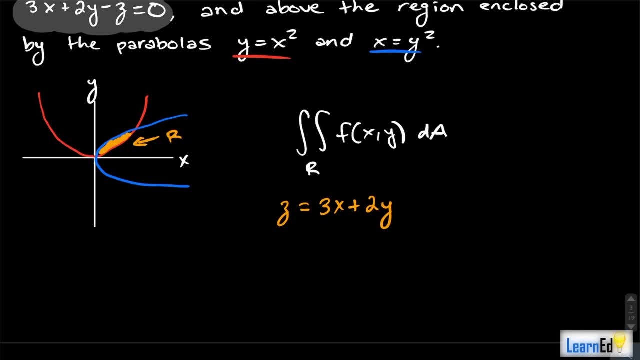 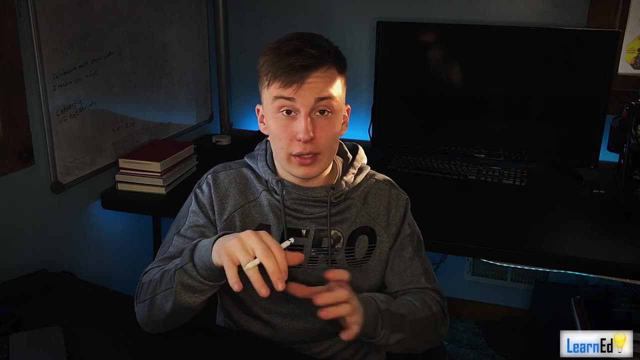 So while we're on the topic of figuring out what's gonna go in this integral, we might as well just figure out the bounds, okay? So, first off, what are our X bounds and what are our Y bounds? Now, remember, when you're setting up a iterated integral, 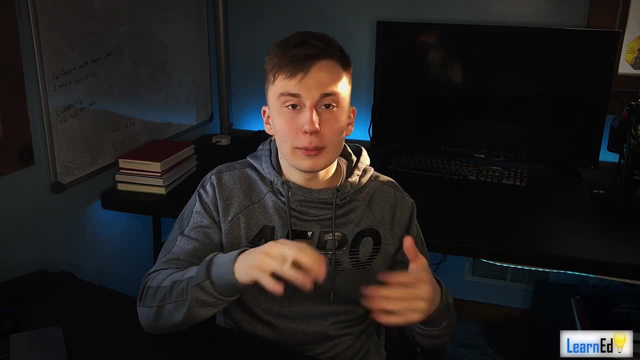 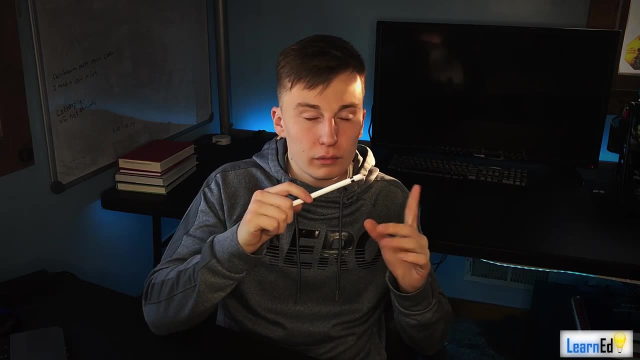 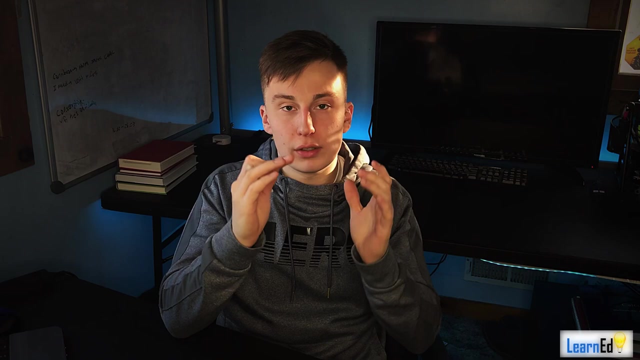 so you have, you know, multiple pieces or multiple integrals to take. you can have variables that'll, you know, come up again in your inner integrals. So let's say that your outer integral is with respect to Y, Your inner integral is with respect to Y. 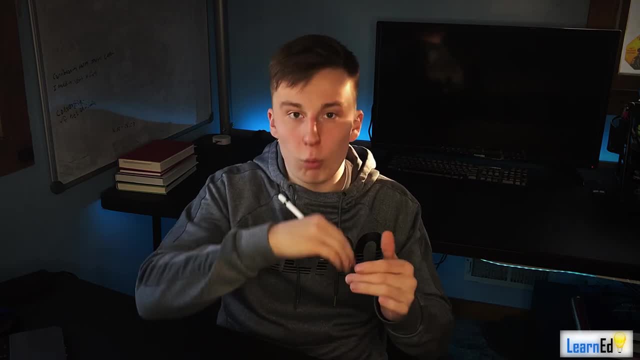 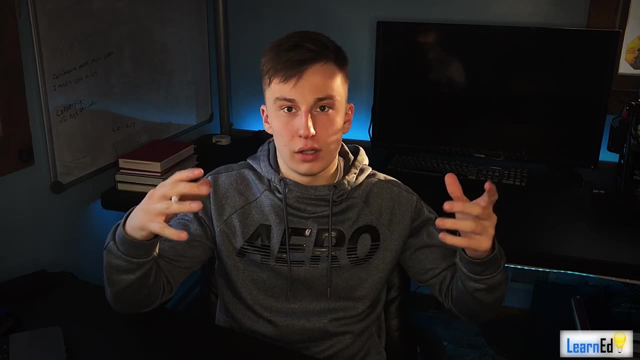 Your inner integral is with respect to X. Your inner integral can have bounds of Y- okay, Because that's just gonna get taken care of with your outer integral- But your outer integral can't have bounds of, you know, X or anything like that, or well, that doesn't make. 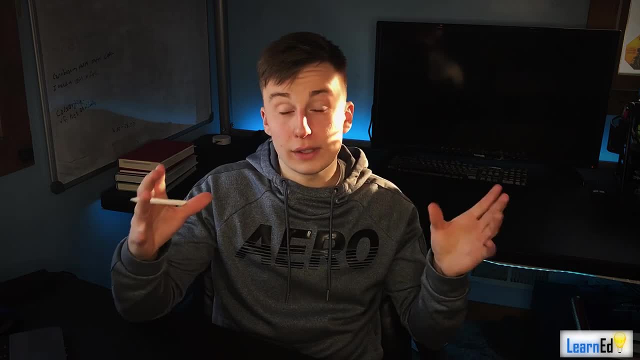 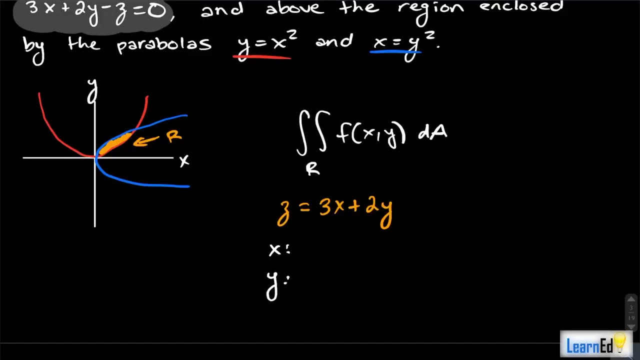 yeah, I mean whatever, But you get the point. Your outer integral can't have variables. Your inner integral can, if they get taken care of later. Okay, so we're gonna use that to our advantage here. okay, So our X bounds, let's actually write this: 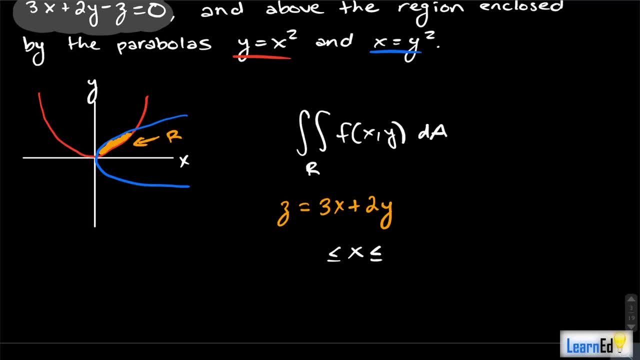 a little bit differently. So what is X between here? Well, if we wanna just put it simply, I mean we kind of can understand that that intersection point is at one one right? So the max and min values of X and Y are both zero to one. 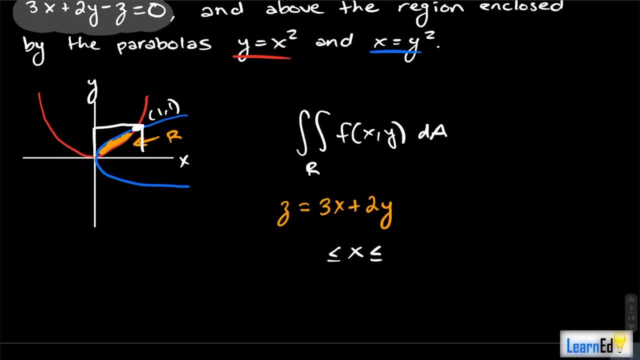 But we need to take into account the fact that we're not integrating this whole. we're not integrating over this whole square. Our region is just this parabola. So what I'm gonna have X do is I'll have X go from zero to one. 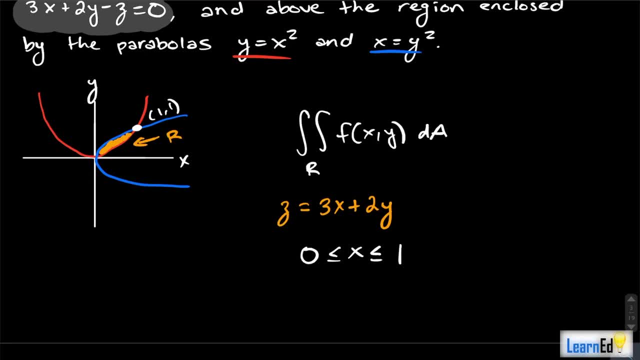 So what I'm gonna have X do is I'll have X go from zero to one. So what I'm gonna have X do is I'll have X go from zero to one. Okay, because that'll be our outside integral, But then our inner integral will be Y. 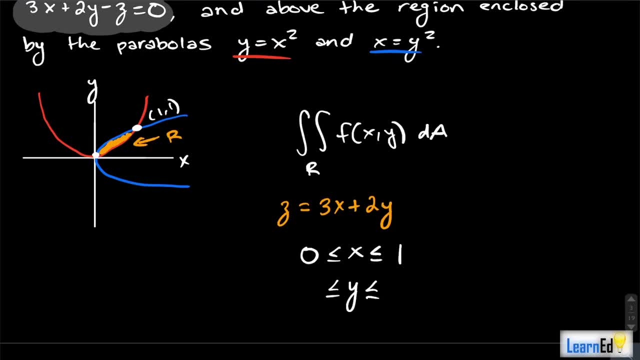 and it'll take care of these two curves, okay, So the bottom of our Y is this curve right here. That's Y equals X squared. So it's at the bottom of Y is X squared. The top of Y is X equals Y squared. 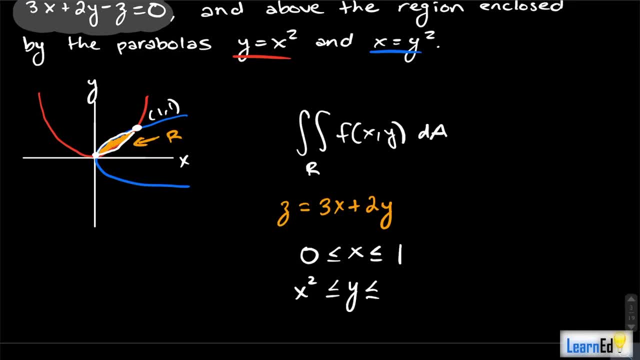 In other words, Y equals rad X, not negative rad X. In other words, Y equals rad X, not negative rad X, because it's not going below this curve. We're not dealing with any of this, so no, So just rad X. 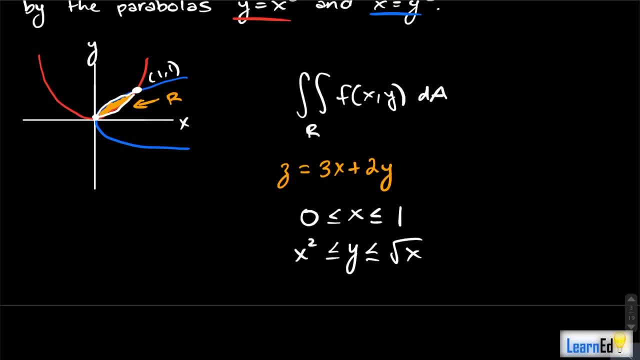 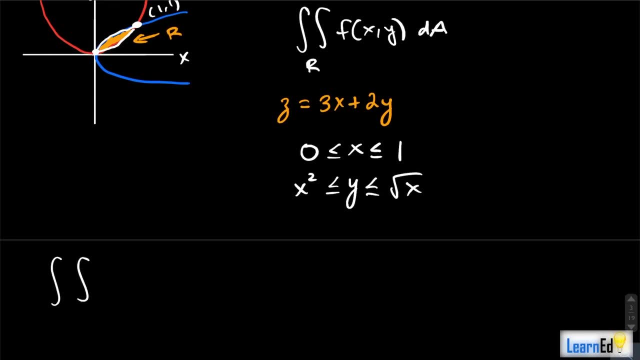 Okay, so let's set up this integral, and then I'm gonna help you understand this even more. Okay, Our region, We know that our inner integral is gonna be have bounds of X squared to rad X, and our outer integral is gonna be from zero to one. 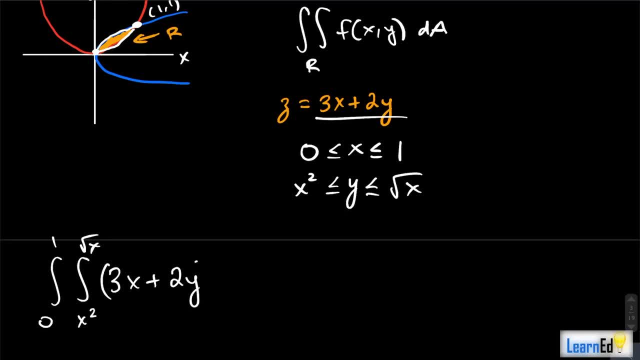 Our integrand is gonna be three X plus two Y, And remember that our inner integral is DY And then our outer integral is DX. So what happens here, okay, Is that that inner integral, Okay, That takes care of those two curves. 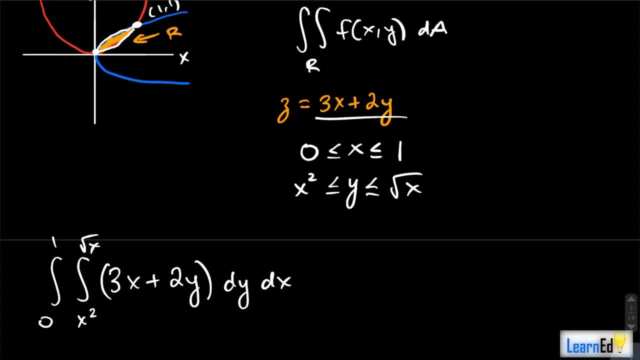 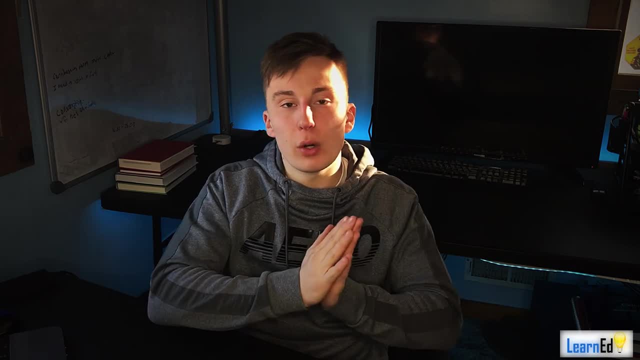 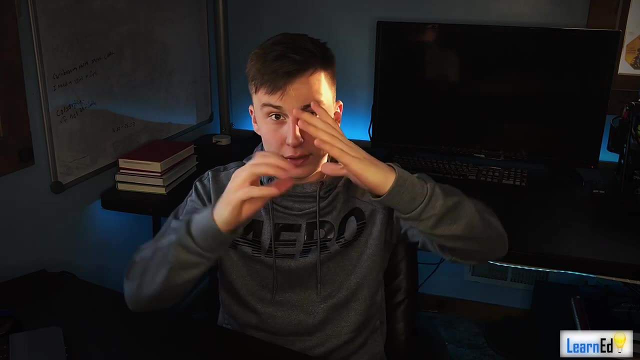 Okay, So that's defining exactly where your region will be as you integrate over it. okay, But you now need to integrate over it on X, right? You need to give it. give it some some width, okay, because it already has it. already is the length figured out, right? 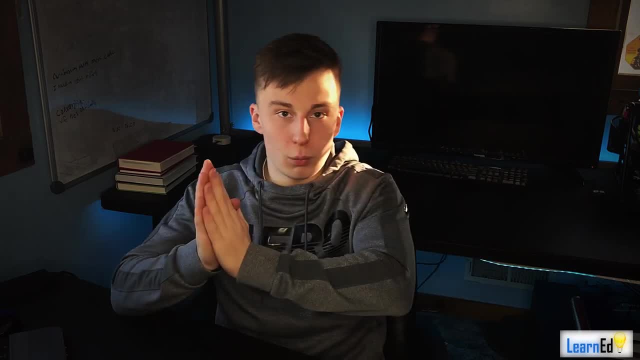 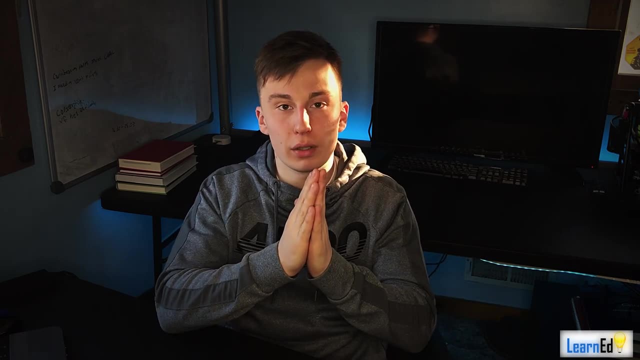 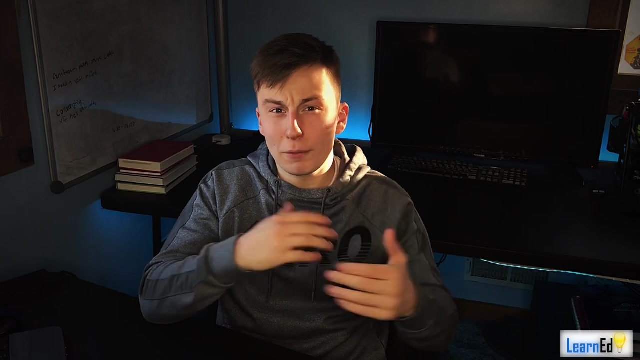 the spacing in between those two curves, but you don't need to give it the width. okay, since we already took care of those. the placement of those two curves we can now integrate over- and actually maybe this is the way you would look at it- from zero to one, okay, so hopefully that makes more. 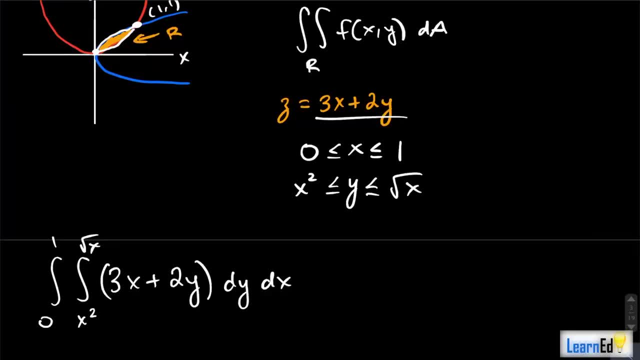 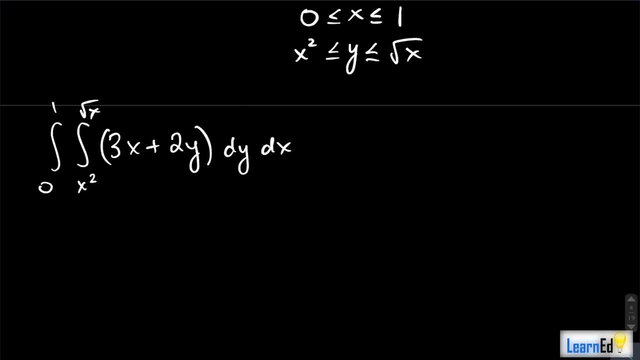 sense okay, so let's, let's just, uh, did i say okay, we are going to integrate this, so what i'm going to do first is just integrate with respect to y, so we get the integral from 0 to 1, right of, we're going to take care of this inner integral first, so we get a 3xy plus a y squared. 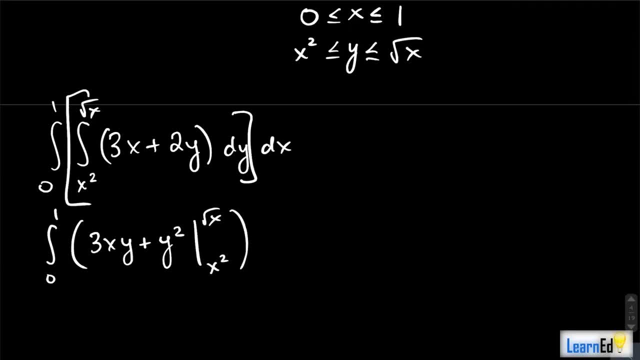 and that's going to be 4, 3x, y and that's going to be the oriented loss. all right, so we're going to do this integral to be evaluated from x squared to rad x, dx. okay, because that's our outside integral is dx, so we 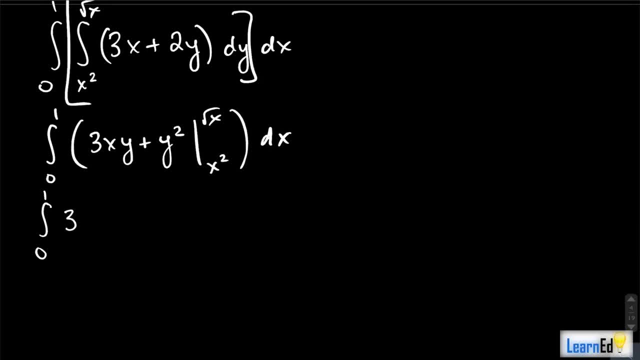 have the integral from 0 to 1 of a 3. see if you could follow me here. uh, i don't want to go too fast, but i don't want this video to be hours long. so we have a radix we're plugging into y, so we're. 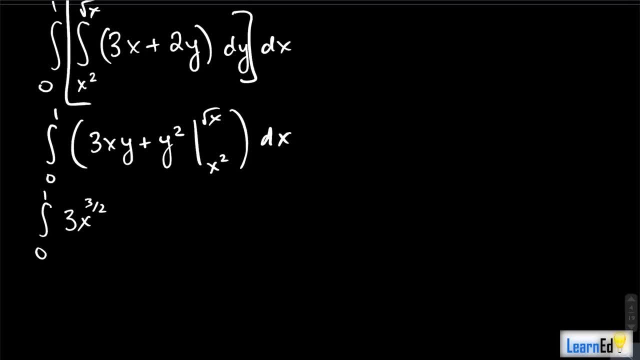 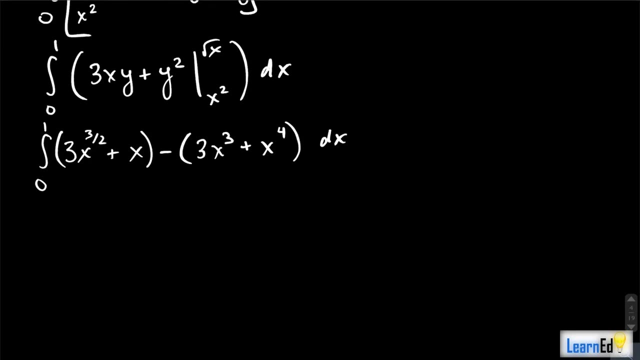 going to have a 3x to the 3 halves. we're going to have plus a rad x, squared is x, and that's going to be minus a 3x to the third plus x to the fourth. okay, and then we have a dx there. 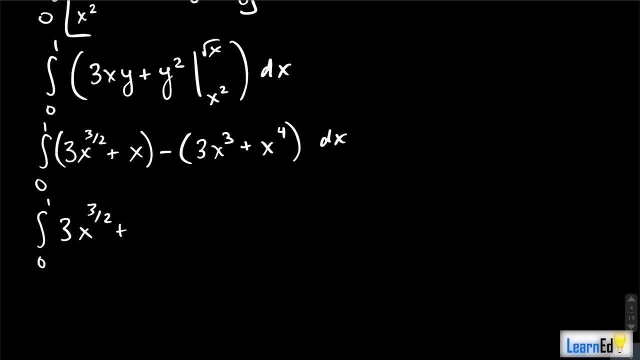 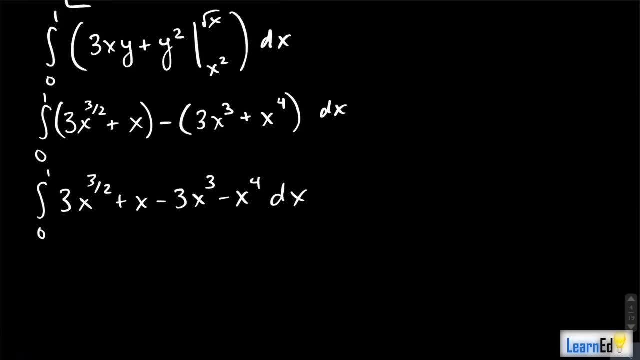 all right, distributing that negative, we have 3x to the three halves plus x minus 3x to the third, minus x to the fourth dx, and we can integrate this to be: we have a two fifths times three x to the five halves plus x squared over two minus three x to the fourth over. 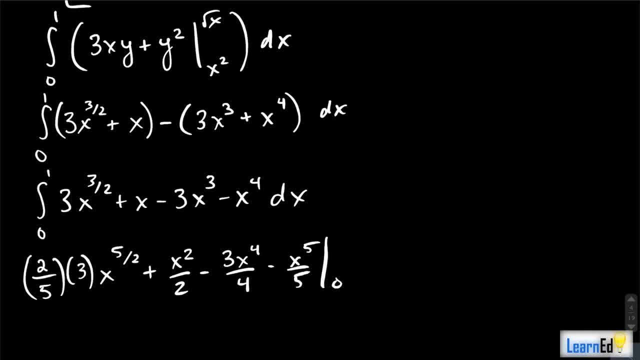 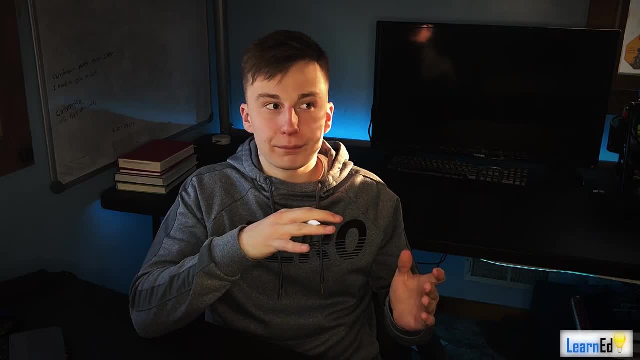 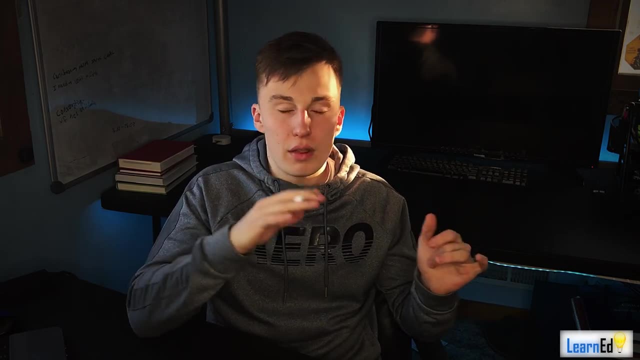 four minus x to the fifth, over five, evaluated from zero to one. i really like when you uh integrate from zero to one, because and you just have like a polynomial uh with, like you know, no exponentials, it's just like a straight polynomial. all the x's go like first off, the zeros don't matter. 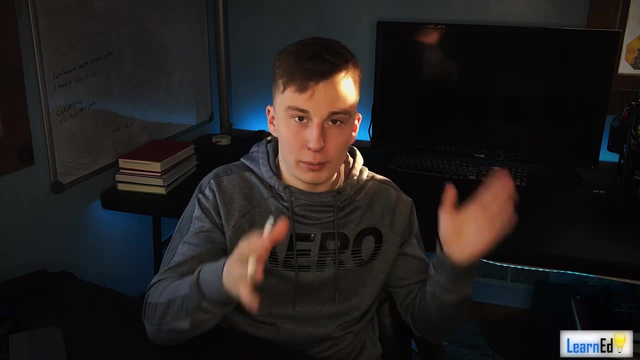 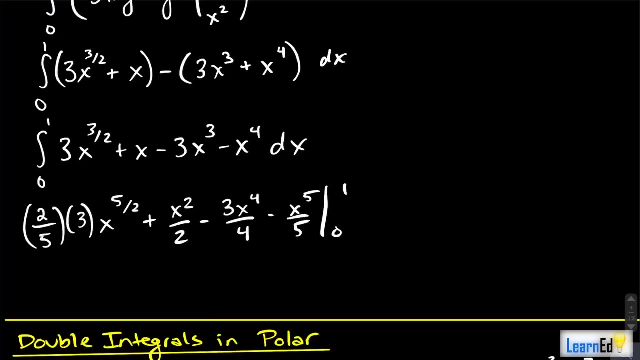 and then all the x's just go away. it doesn't matter what power is on them, it's just one, right? so you kind of just go by the coefficient. so it's really nice when that happens. but yeah, c of two fifths times three plus one half minus three over four minus one fifth, and i'll just uh. 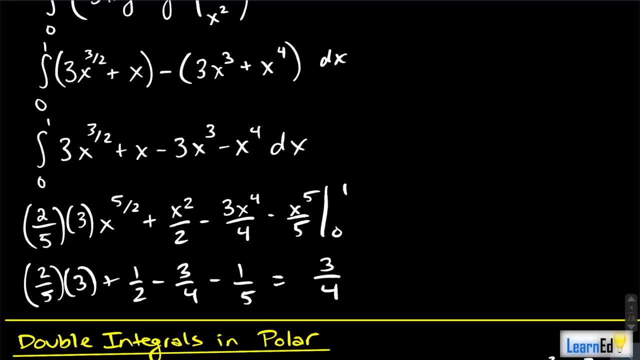 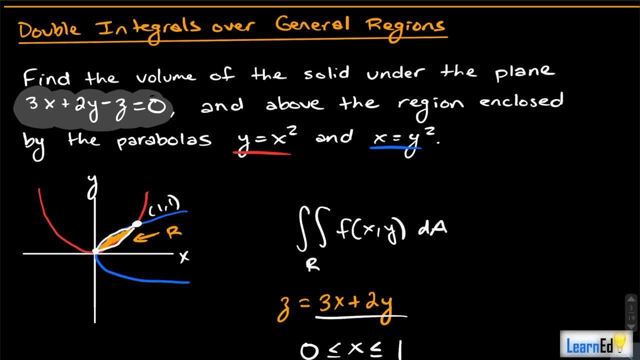 simplify this for you guys, because there's no need to worry about any of that stuff. that's just three fourths, okay. so just to recap right. the original question was finding the volume of the solid under the plane. 3x plus 2y minus z equals 0 and above that. 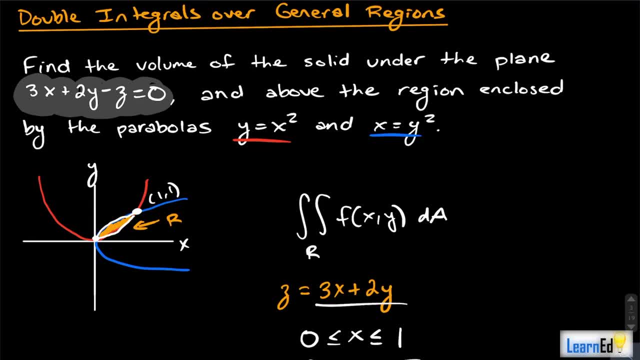 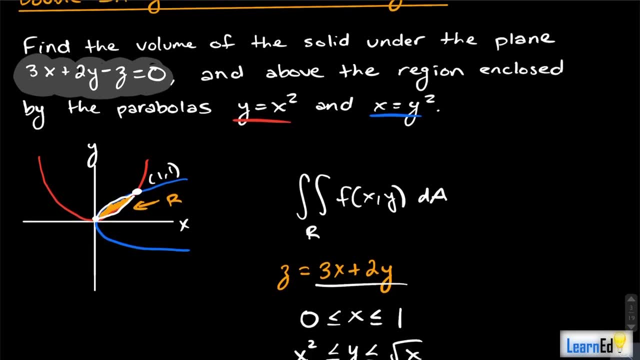 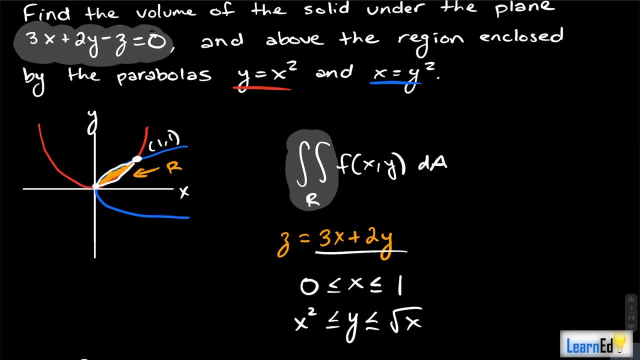 region enclosed by the parabolas y equals x squared and x equals y squared. okay, we found that region in the xy plane. okay, and you know that was half of the battle. finding that region r is the region. r means we find our bounds. okay, the only other thing we need to do is remember the the. 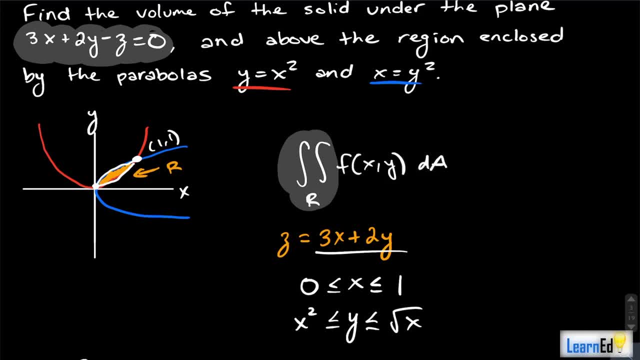 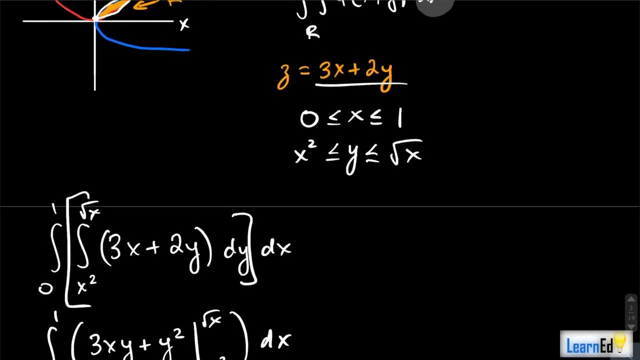 integrand right, that's going to be our surface, which is our, which is that plane that i have highlighted over here. right, we put in our da we plug in our bounds. right, making sure that our outer integral does not have any variables in the bounds, but our inner integral can. 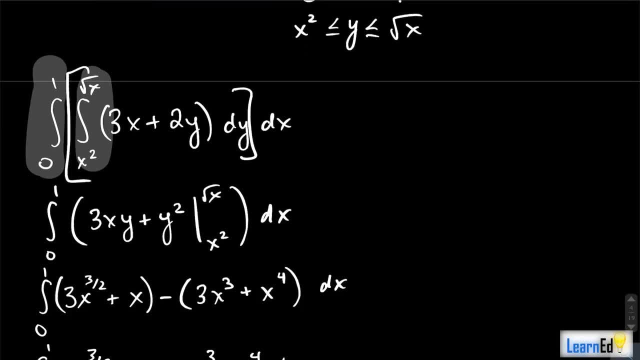 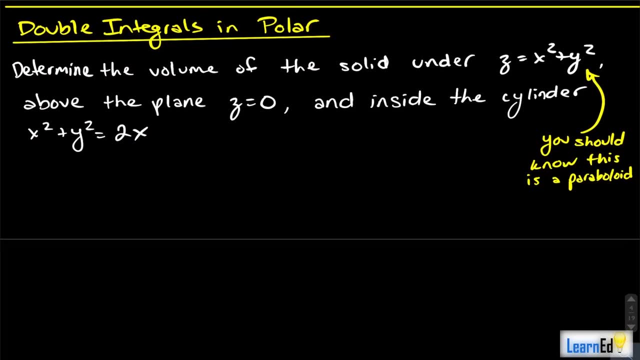 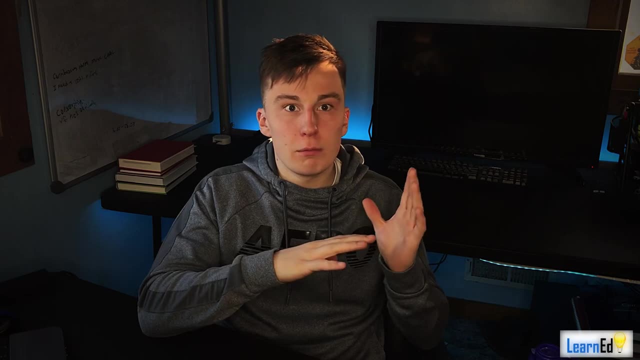 okay, and you know, voila, a nice iterated integral that you can go out and do, and it's not really that big of a deal, okay, so next we're going to be looking at double integrals in polar coordinates. okay, because, you know, not always are you going to want to have. 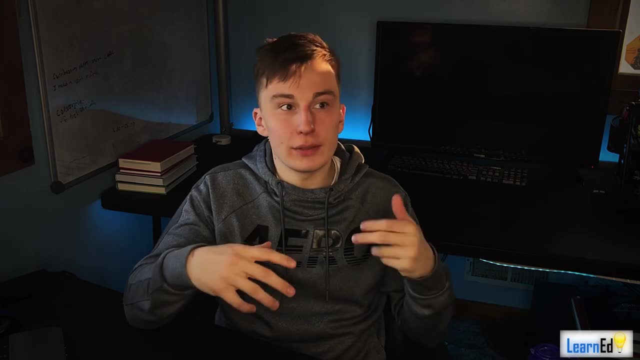 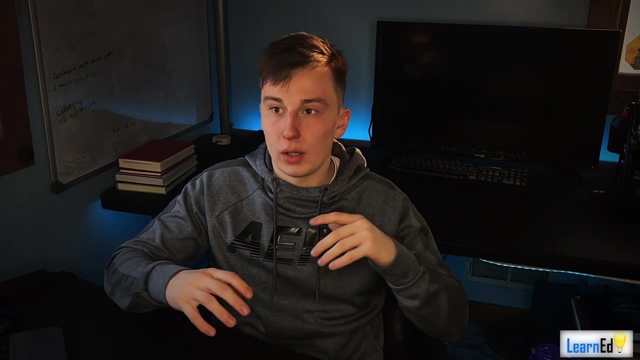 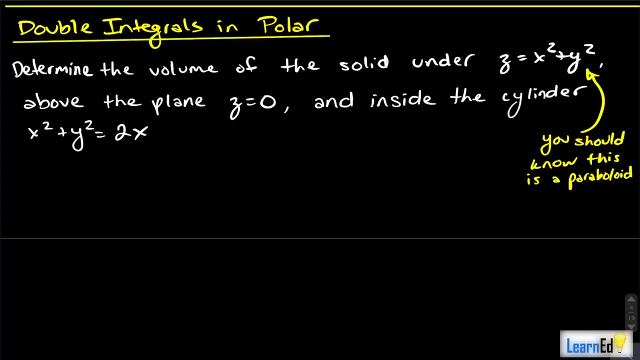 your double integral in regular cartesian coordinates, because your bounds are going to be really, really gross and they're going to be much easier to deal with if you have them in a different set of coordinates. the only other one that we learn that we use is polar. okay, so let's do a problem with with that. 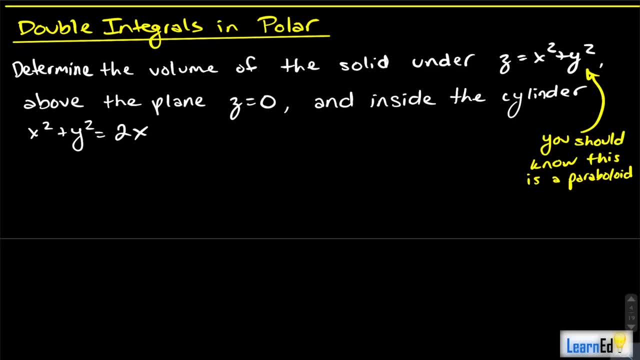 so determine the volume of the solid under: z equals x squared plus y squared. above the plane, z equals zero and inside the cylinder, x squared plus y squared equals 2x. okay, so you know, this is going to be a little more, it's going to be more difficult than the. 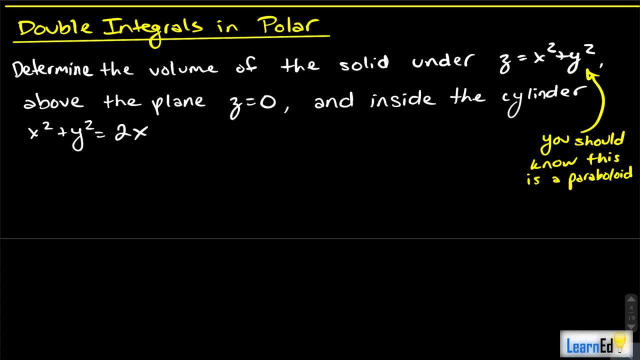 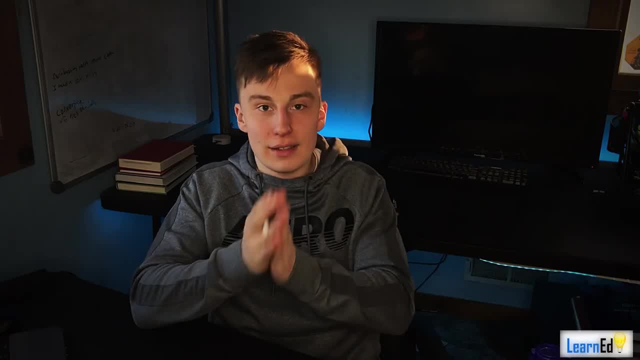 last problem, because you know, we got to first graph this, we got to understand what this looks like, and the reason why i have this noted here- you should know this is a paraboloid- is because i didn't in calc 3. okay, i had no idea what that was, honestly, and that's why i struggled. 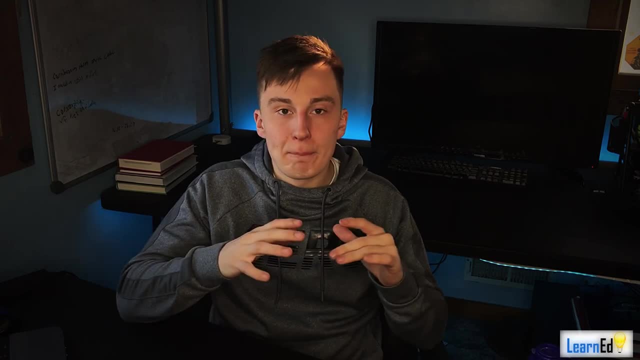 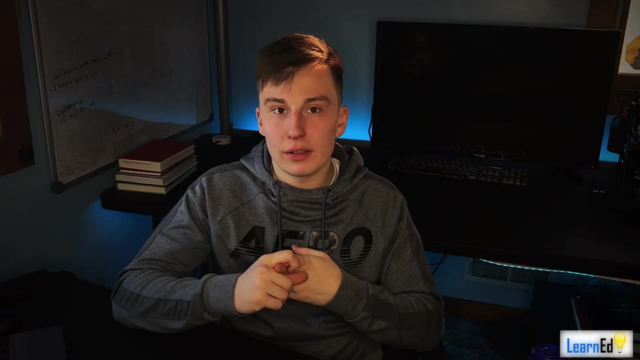 so much with multiple integrals. that's why i struggled so much with vector calculus. i couldn't visualize this stuff in three dimensions because i didn't know my quadric surfaces. okay, i honestly didn't understand how to graph a plane. i think until i started. uh, i think until i 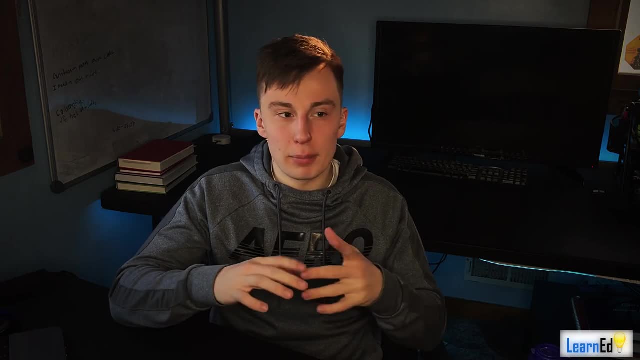 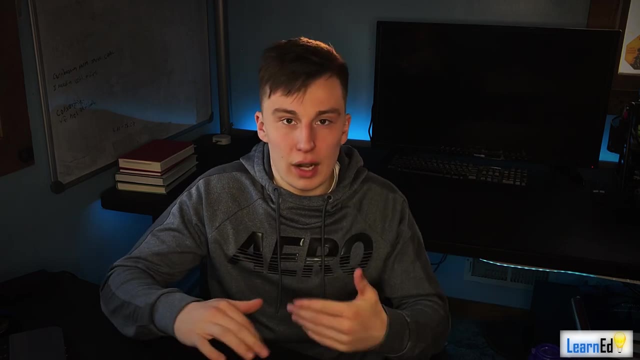 started like multiple integrals, like like double integrals and stuff. because you know, and i know it's probably a pretty common sense thing to most of you, but it wasn't to me and you know, i eventually figured it out on my own but i was like you know, i i couldn't graph in three dimensions. i. 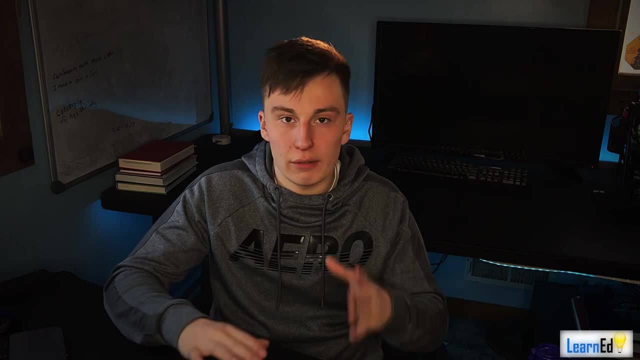 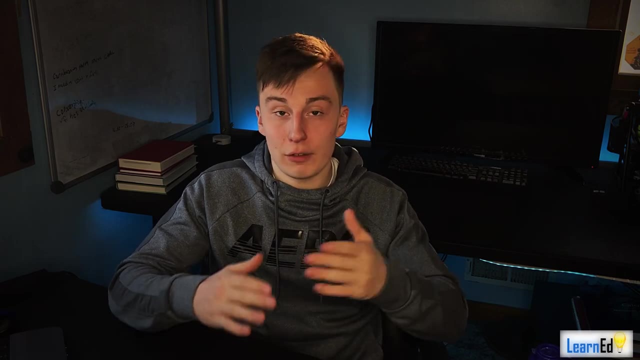 went over quadric surfaces, i went over planes, i went over all that stuff. i figured it out and that's why now i'm able to do these problems a lot easier and that's why i really, you know, push that off to you guys- make sure you know how to graph in three dimensions. okay, go over quadric surfaces. 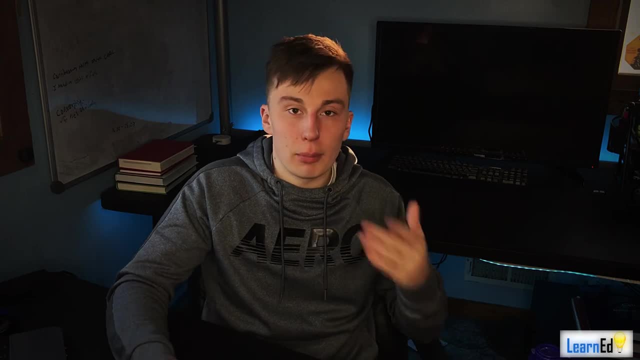 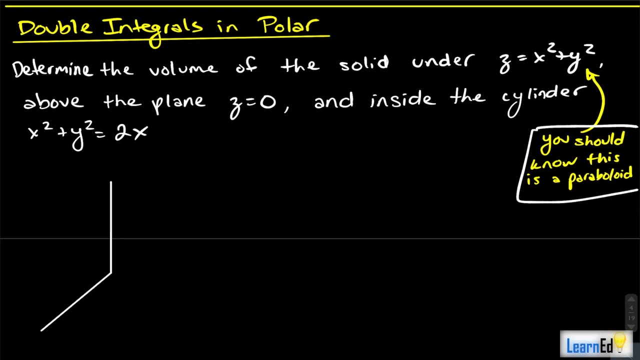 go all that stuff, go over all that stuff, because it's really really important for problems like this. getting into the problem, we're going to first graph this, okay, and if you know this is a paraboloid, you know what it probably looks like. remember that this is kind of just like an extension of a parabola into three dimensions. 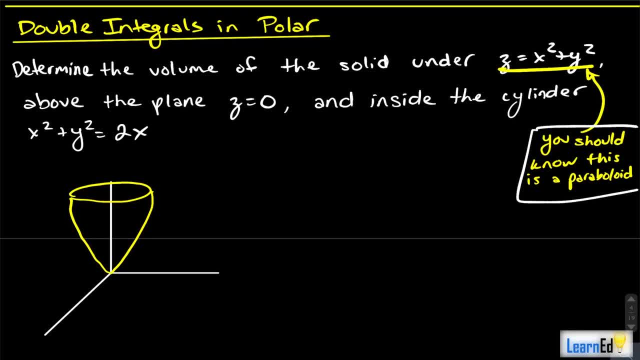 okay, so there's your paraboloid, okay. next, we're going to graph our cylinder. now our cylinder. well, that that looks a little gross right now. right, x squared plus y squared equals 2x. how does that a cylinder? well, what we can do is complete the square here. so we're going to move that 2x over. 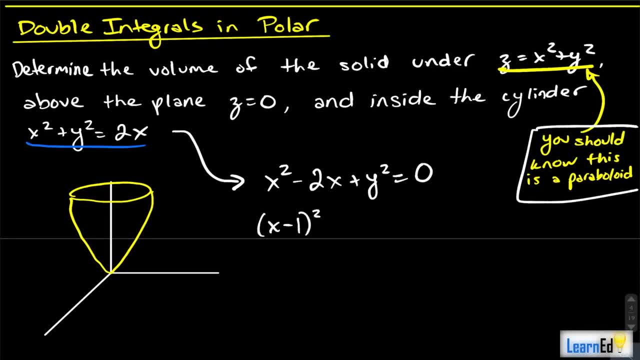 okay, and then we complete the square, and i'll just go ahead and do that quick: x minus y, one quantity squared plus y squared. and then we have to move a one over to the other side and we get one that tells us that, well, our cylinder is going to have a base with the, since this is the x, this is the y, this is the z. 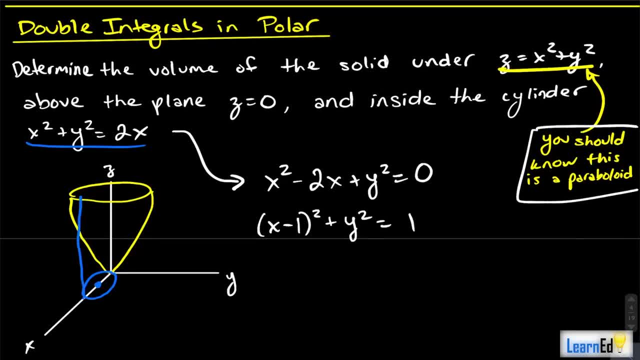 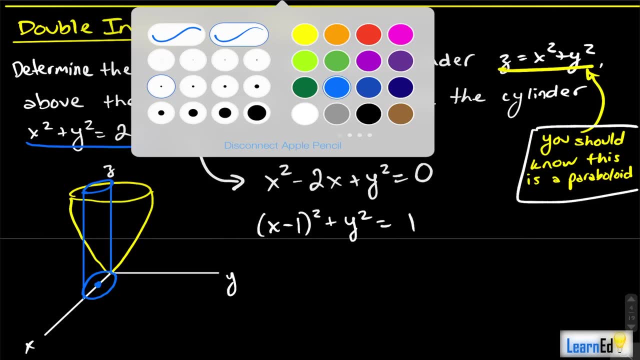 our cylinder has a center of x equals one, and a uh and y equals uh- zero. okay, so there you go. that's our cylinder. like i said, yeah, i i'm not very good with with the drawing. i've gotten a lot better with these visuals. i'm not really utilizing what's going on, but my drawing still sucks. 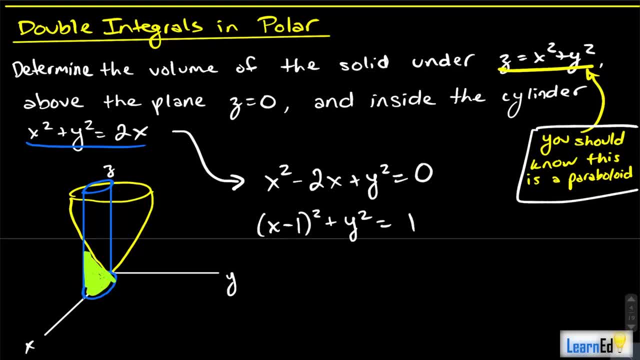 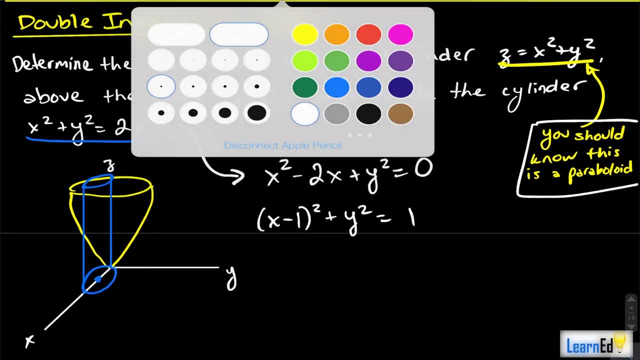 anyways, this is what we're finding here. is the volume of this solid? okay, but here's the thing: we need to still look at this in two dimensions to find our balance, because let's go ahead and set up our integral here, that's going to be the integral over that. 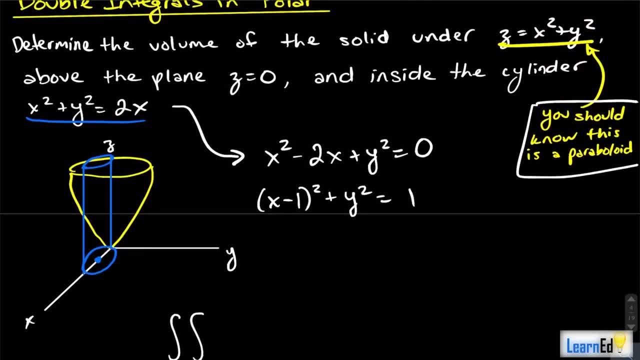 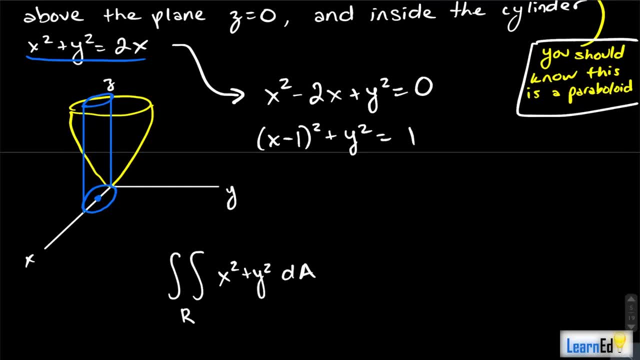 region r, which is going to be in the xy plane. okay, we know our integrand is going to be x squared plus y squared and we have a da here. but we still have to find our, our region r, and that's going to be really, really gross to do with cartesian coordinates. okay, 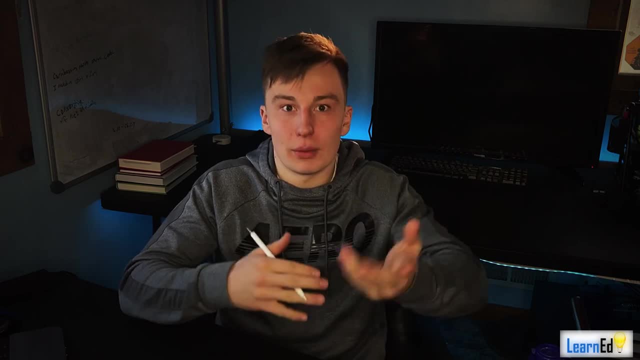 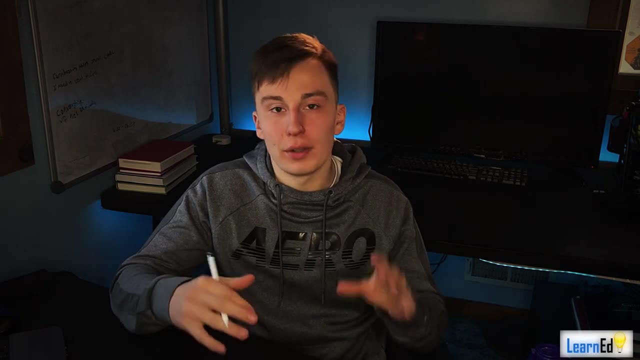 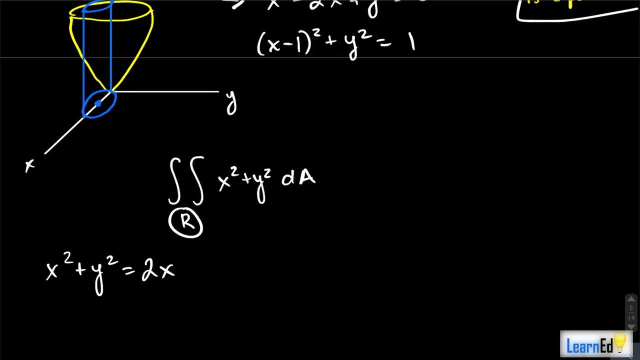 it's a circle, but you know, and that's what makes it bad for cartesian, that's screaming polar at you. and even the integrand x squared plus y squared is screaming polar, okay. so what we're going to do is, well, convert to polar our region. okay, is the the base of that cylinder? so let's figure out how to illustrate the base of that. 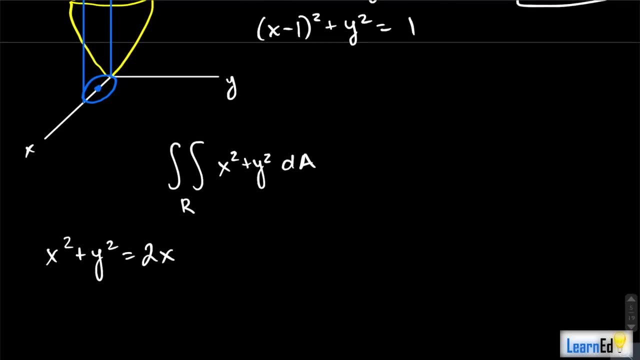 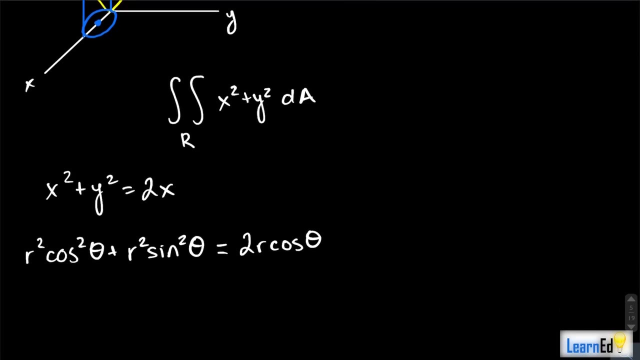 cylinder with polar. remember with polar that x equals r cosine theta. so this is r squared cosine squared theta, and y is our sine theta. so this is r squared sine squared theta and we have 2x to our cosine theta. okay, well, we know that we can take a r squared out here and that just becomes one on the inside right. 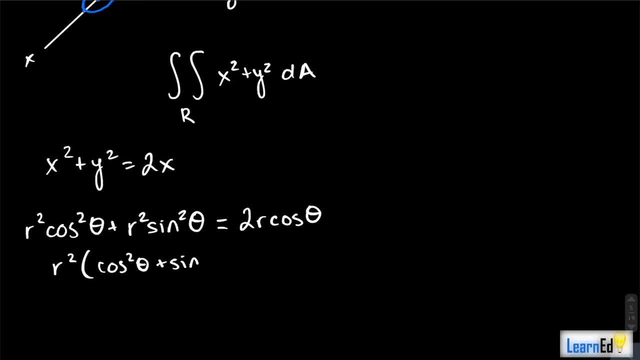 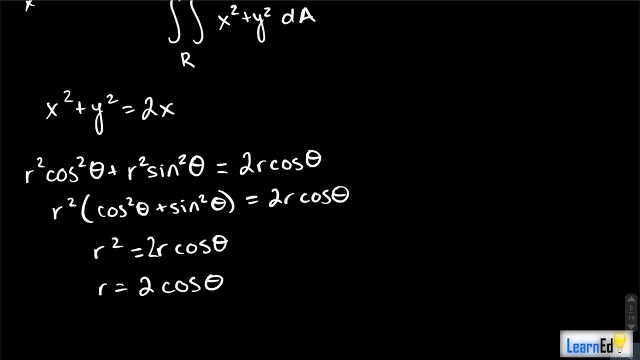 we have r squared times. cosine squared theta plus sine squared theta equals 2r cosine theta plus sine squared theta. so we just get an R squared equals our cosine theta- sorry, to our cosine theta, in which case that we just get R equals cosine of theta when we divide R on each. 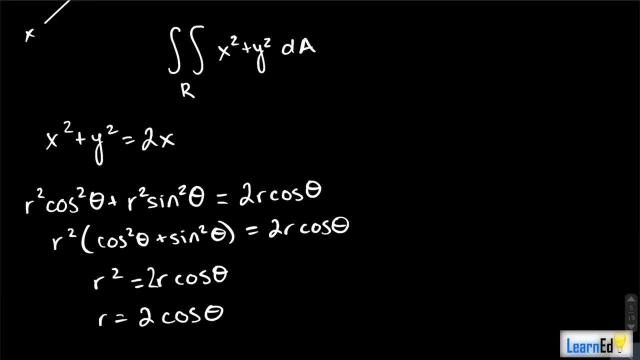 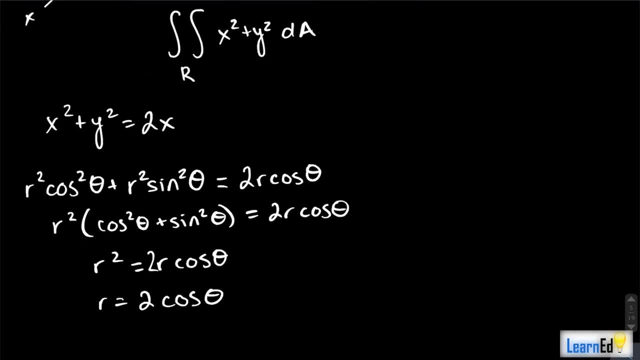 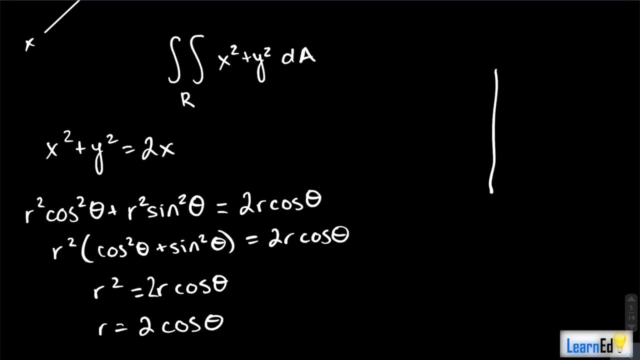 side. so you know, that is what our, our R goes out to. okay, so in and where our R starts out with: okay, let me draw this in two dimensions. okay, if our X is here and our Y is here, then our cylinder are the base of our cylinder, which is a. 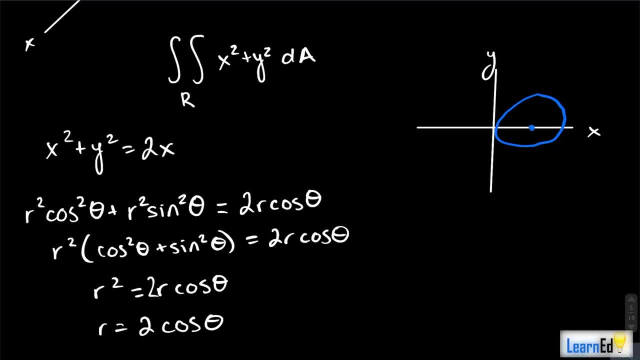 circle- that's an awful circle- is right here with our set, with its center here. okay, that R is gonna start from zero and it's gonna go out to as far as two cosine theta, which is anywhere on this circle. okay, now all that's left to do? 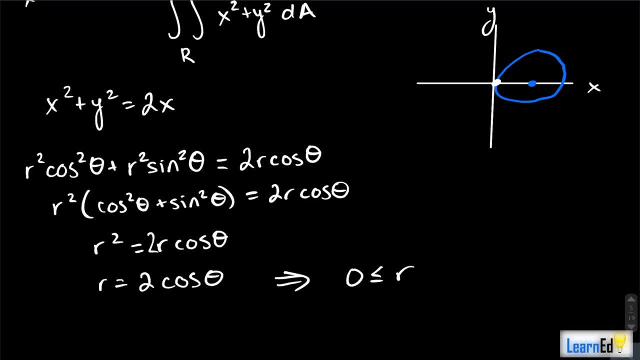 is so, now that we know that our R bounds are from zero to two, cosine theta, what's our? what's our theta gonna be? well, that's gonna stretch as far down as negative pi over two and go up to pi over two. okay, and now we have our region. 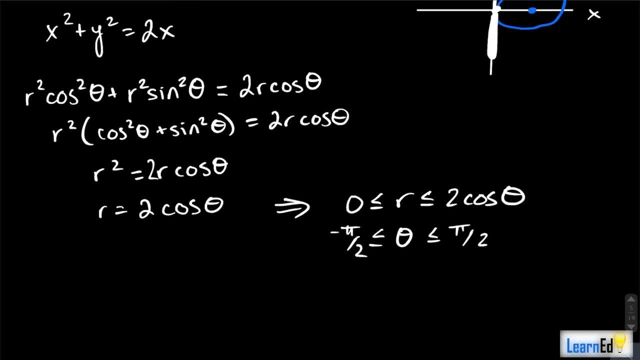 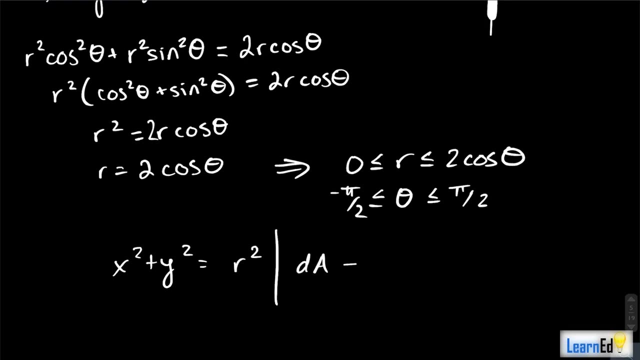 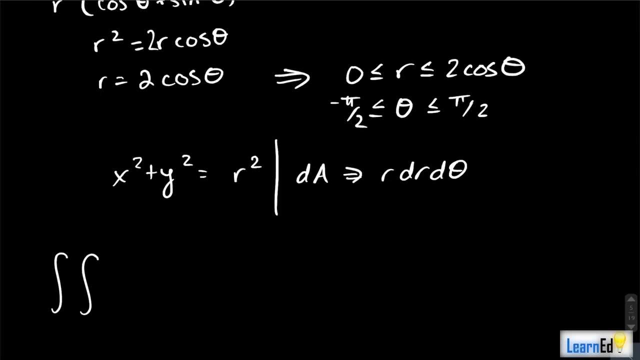 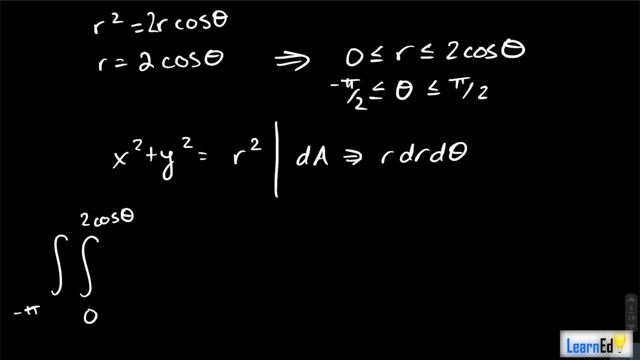 and all that's left to do is just convert our integrand to polar. remember our integrand. x squared plus y squared just becomes you R squared and remember that. da becomes R dr d theta. okay, so really we're gonna have the double integral from 0 to 2 cosine theta and then from negative pi. 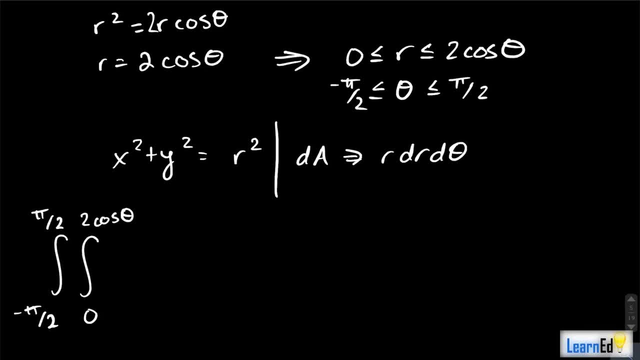 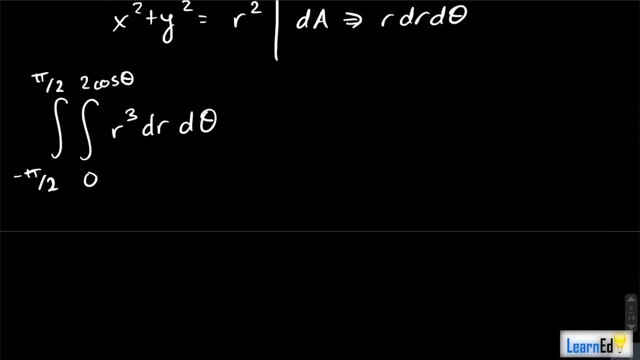 over 2 to pi over 2, our integrand is going to be R squared times R, which is R cubed, and then we have a dr d theta theta. so we're actually not going to be able to split this integral up in, the reason for that being because, well, this, while this R cubed dr and these in this, 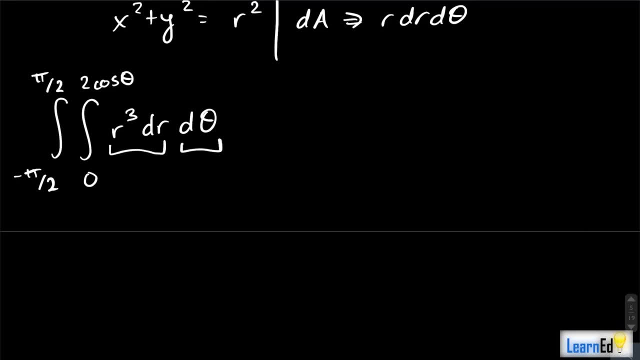 d theta there being multiplied together now, not being like add and subtract or anything like that. we do have this R bound that is dependent on theta, so we're not going to be able to split this integral up, okay. well, we're not going to get a numerical answer, okay. so moving on, guys, if you have a question, just drop in. now and everywhere. we want to have this. let's get this had to come back. okay, so do one or two X. if you have a question, you can reach the Q and then call us 67. let me know how much you want us to do and I don't care. so we're not gonna be able to. 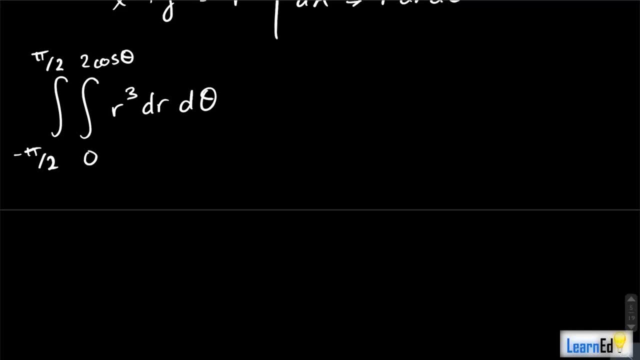 so move on to the next song. President thought is no, the black and white bar. so why is potential than theta and LGBTQ it? after Moving on, let's just do our inner integral first. okay, We're going to get a r to the fourth, over four times well, actually evaluated from. 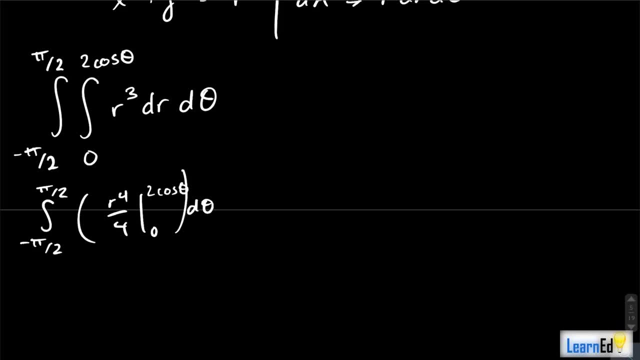 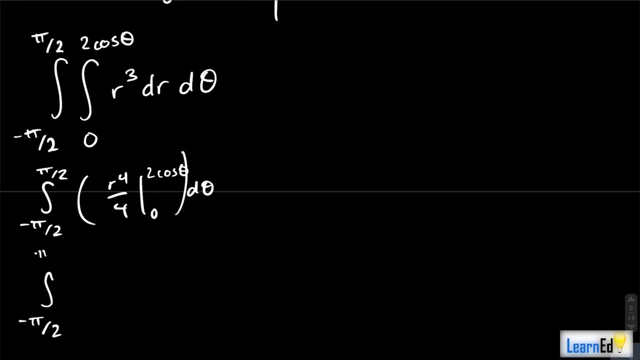 zero to two. cosine theta d theta is on the outside of that. so we're just going to end up with the negative integral or, sorry the man, the integral from negative pi over two to pi over two. of this will just be a two to the fourth times cosine fourth theta over. 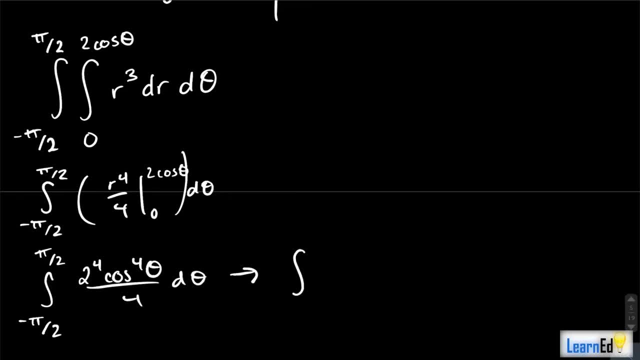 four d theta, which is just going to become the integral from negative pi over two to pi over two, of two to the fourth is sixteen. sixteen over four is four, so we're going to have four, the integral, of course, cosine to the fourth of theta. we can also make this: 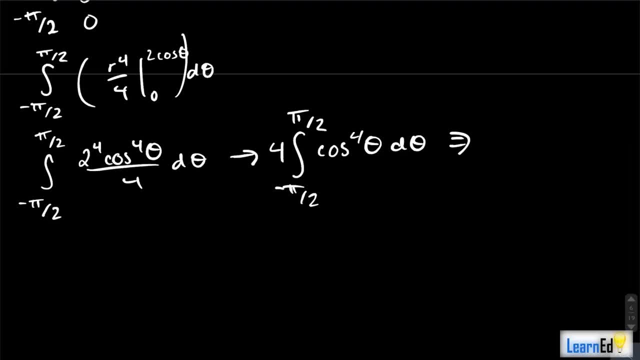 eight- we can just rewrite this again as eight. the integral four, From zero to pi, over two of cosine to the fourth of theta, and I've said this in my calc. two final review video, but I'm going to say it again, you know, if you're not sure. 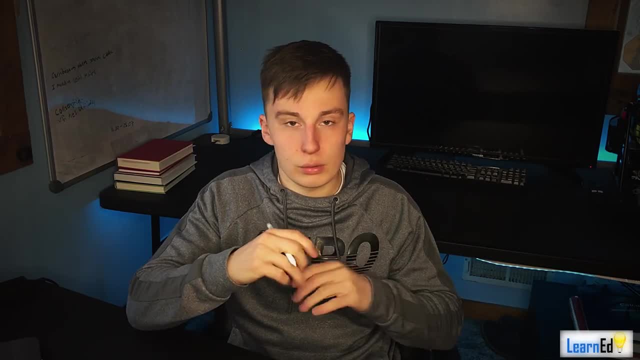 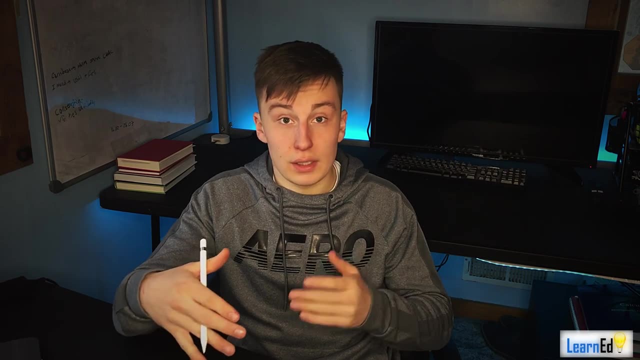 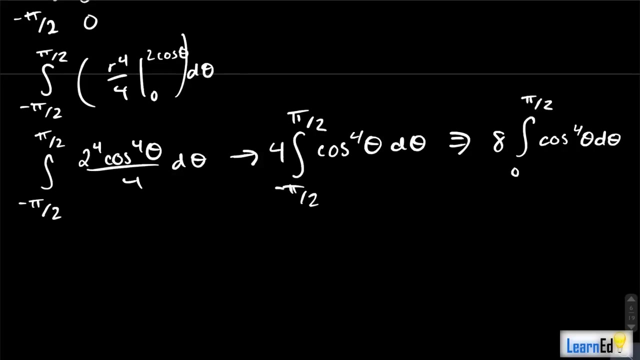 if a function is even or not. don't. don't double it like that. okay, just just evaluate it as is, because that's a safer bet. I know that cosine to the fourth of theta is even, so I can do that. but if you don't know that that's even you know, then take action as 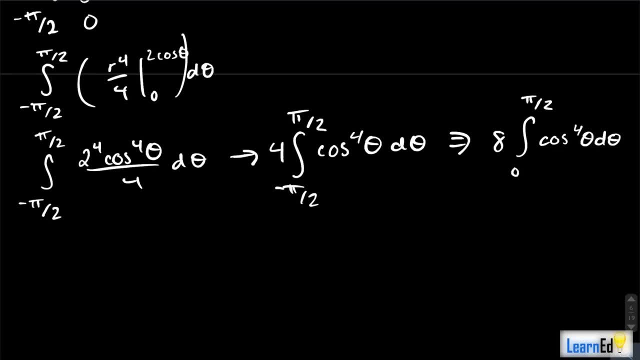 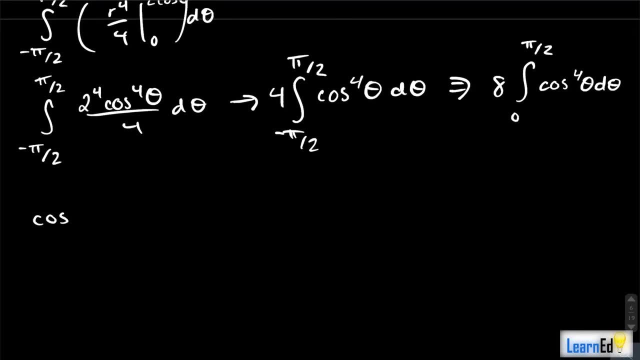 needed. okay, so Moving on. so how do we break up this cosine to the fourth of theta? okay, because it's going to be rough to integrate. well, what we're going to do is, first off, we're just 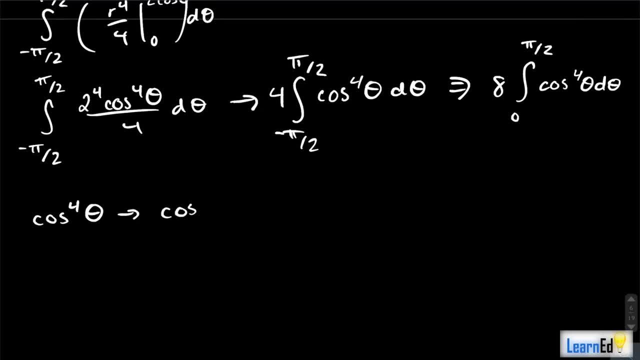 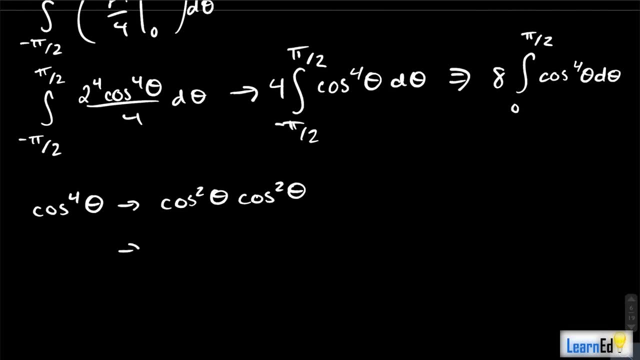 going to write this as cosine squared theta times. cosine squared theta. okay, and remember our, our, our half angle identity. I believe it's called. I believe it's the half angle identity. it's one plus cosine of two, theta over two. 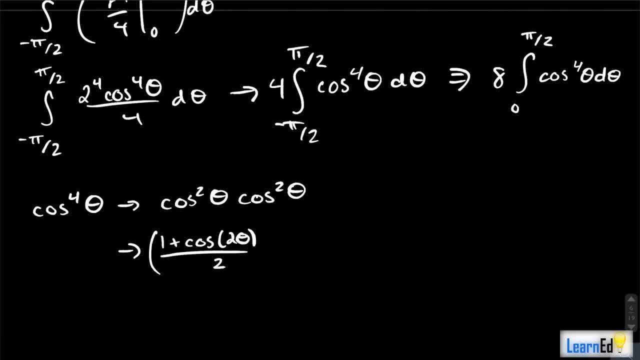 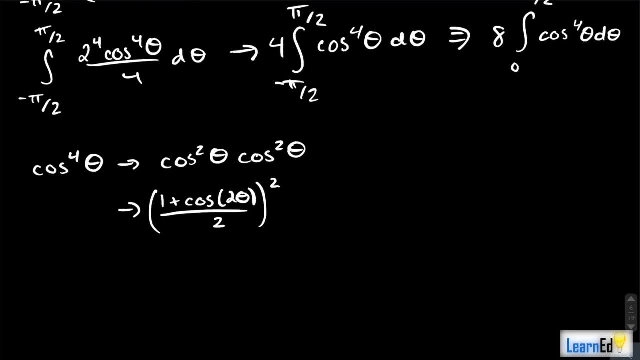 It's equal to cosine squared theta. so if we multiply this by itself- in other words we square it- we get cosine to the fourth of theta. okay, so our denominator just becomes four. right, but that's, that's. that's. you know, two squared. but then we have to actually 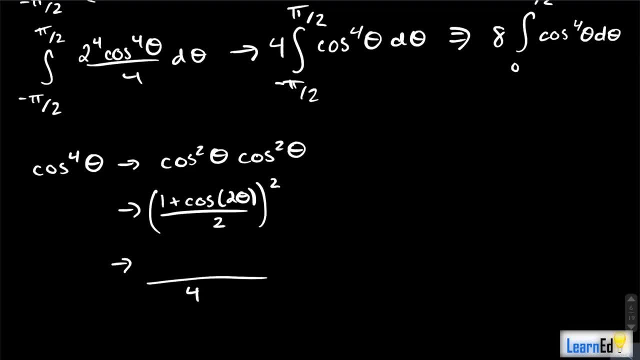 square the numerator, and well, we get one plus, We'll have, Okay, A two cosine of two theta, and then we'll have plus cosine squared of two theta, which we're going to have to apply that identity again to to get one plus two cosine of two. 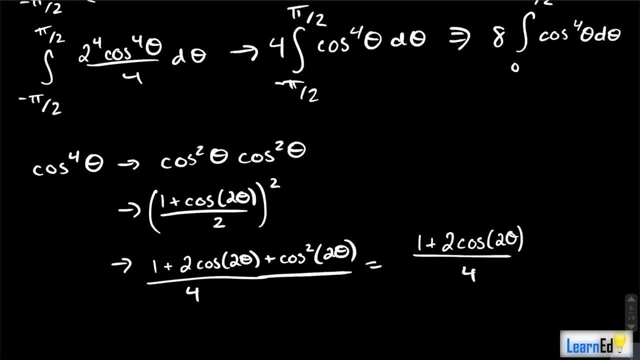 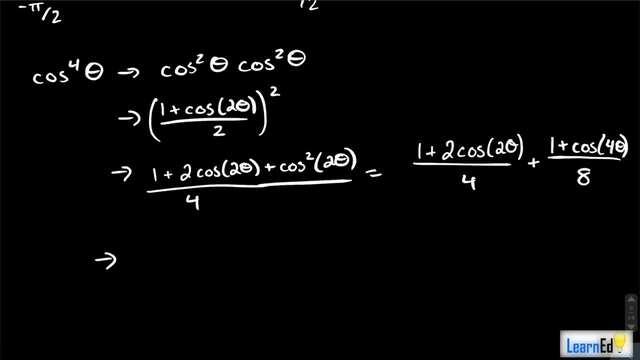 theta over four, and then we'll do plus one plus cosine of four theta over, and this will be over eight. okay, So, simplifying that down, we have one fourth plus two cosine of two theta over four, plus one eighth plus cosine of four theta over eight, which we can just write as we can. 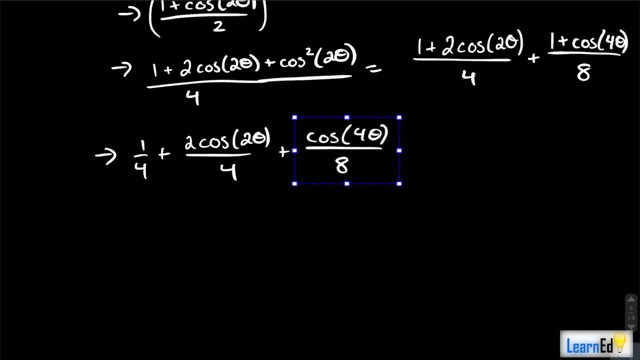 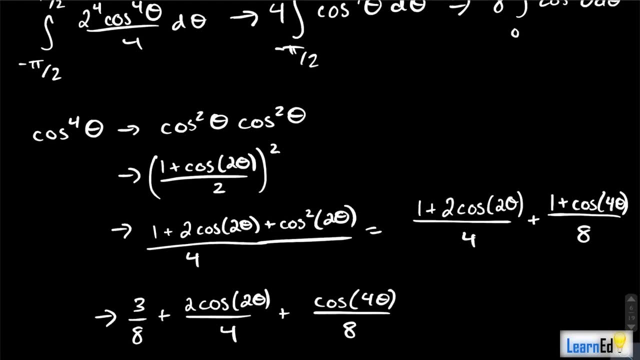 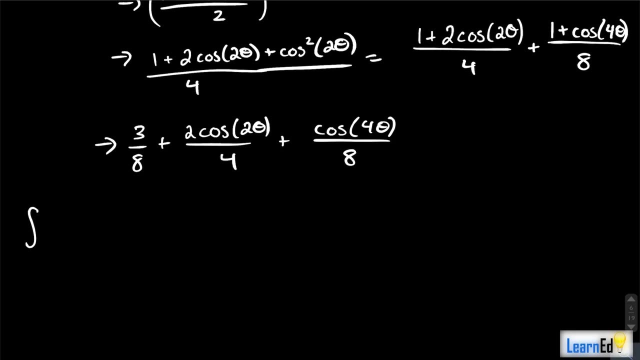 rewrite this as: take out this one eighth, add it on to this one fourth to get three eighths, and there you go, There's our integrand So now we just have the integral from negative. well, no, we don't. no, we don't. zero to 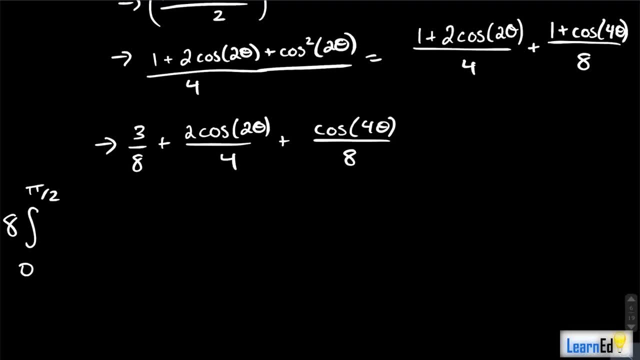 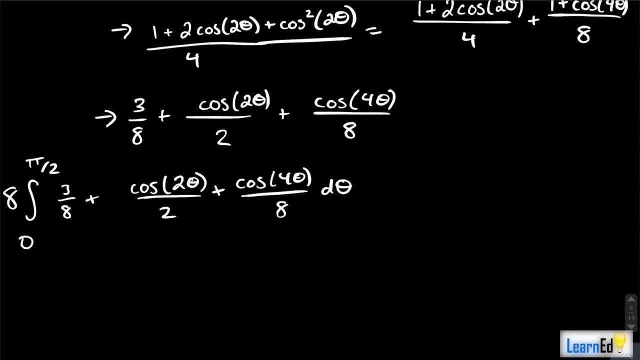 pi over two. we have an eight on the outside and we have a three over eight plus two cosine of two theta over four, which we can rewrite as cosine of two theta over two- didn't see that at first. So plus cosine of four theta over eight, and then we have a d theta. 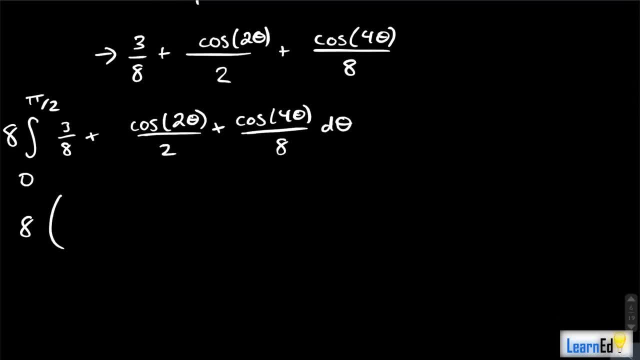 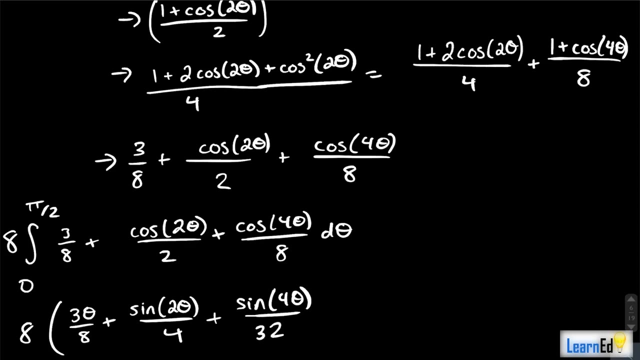 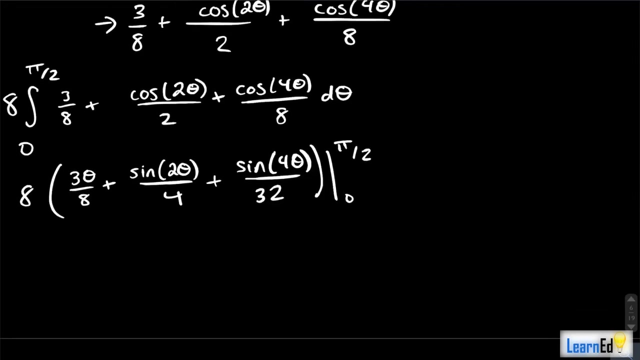 Integrating, we get eight times three theta over eight. plus this will be a sine of two theta over four, plus sine of four theta over 32, and then we will be evaluating this from zero to pi over two. Okay, the zero will make everything go away. pi over two, that's a different story. what 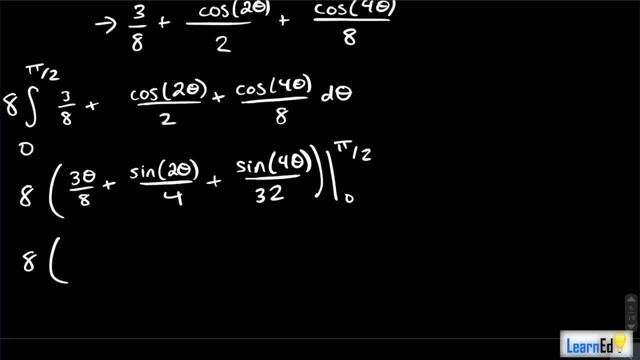 we'll have is a eight times three, pi over two, divided by eight, plus pi over two. well, we'll get a sine of two, theta, theta. we have a pi over two there. so two pi over two, that's just pi. sine of pi is zero, so that's gonna not do anything. also for the sine of four. 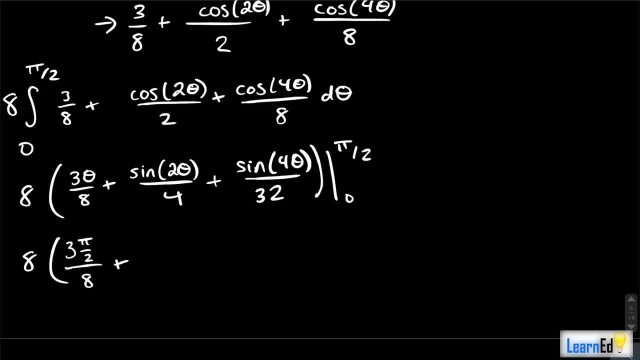 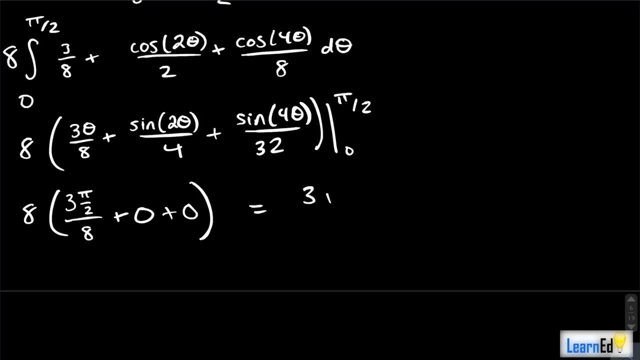 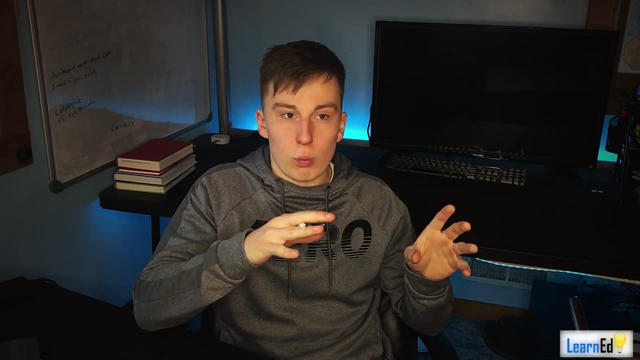 theta that becomes sine of two pi. that won't do anything, so this will just be plus zero, plus zero and the eights cancel. so you're just left with three pi over two. okay, While the the polar stuff was, you know, pretty, pretty intense, right we had to make 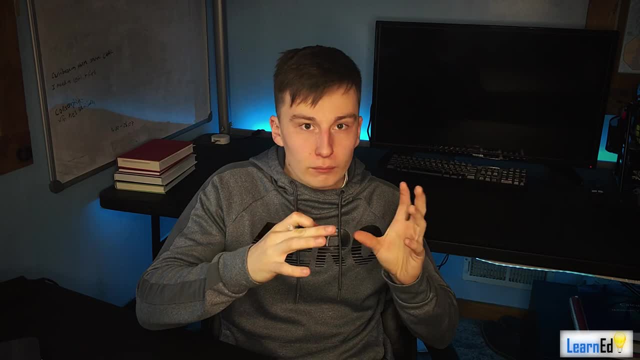 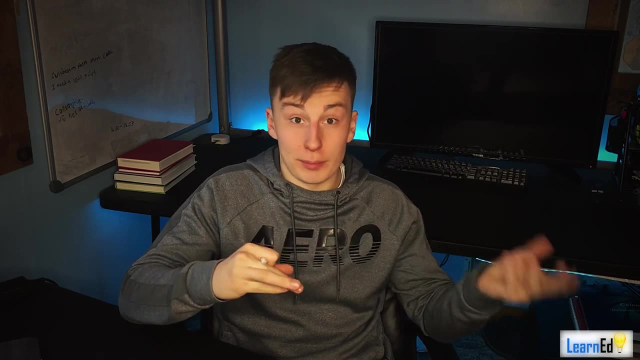 sure that we understood, Okay, What our, our region of integration actually was. you also need to understand how to you know, do like integrals from calculus two, like cosine to the fourth of theta, because something like that is going- you know, is most likely going- to pop up on your final. 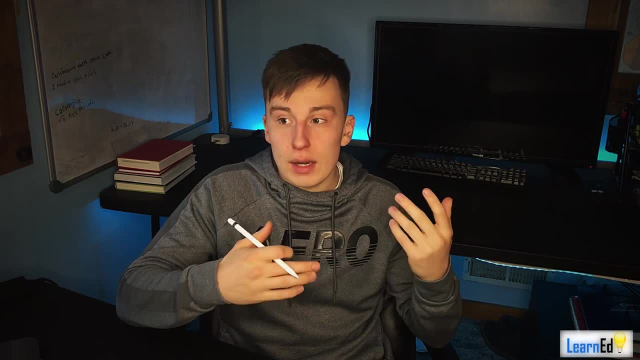 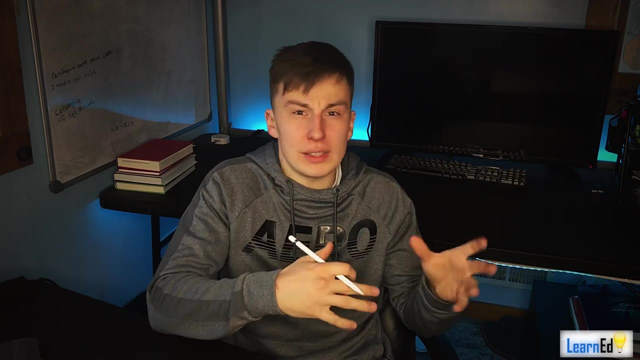 okay, some integral that's a little bit tougher to do. okay, and- and I'm not sure how many of those they'll really be throwing in, because of course you know this is a calculus three test. I want you to focus the most on the calculus three information, but you know. 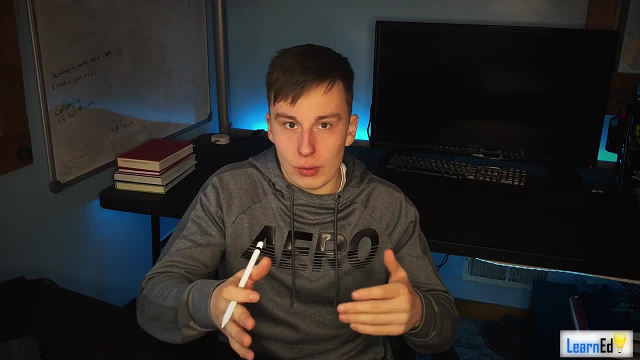 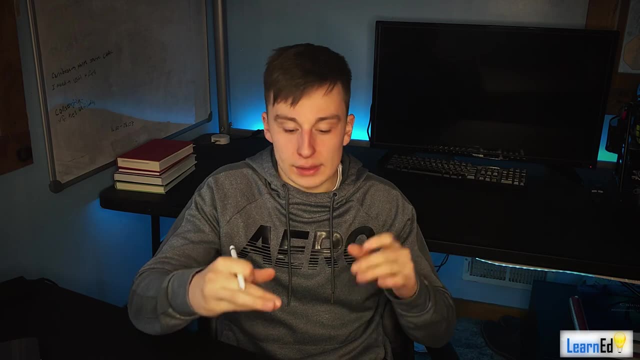 depending on the how, how rigorous that calc course has been so far, you know maybe expect more or less of those types of integrals on your test. so you know, just really refine your knowledge on certain techniques of integration if you don't feel very comfortable on them. 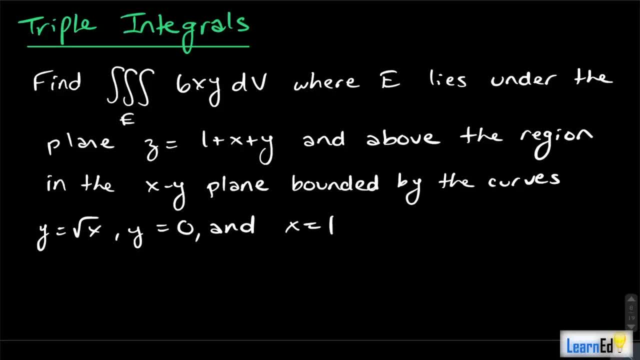 All right. so next we're going to be focusing on triple integrals, So we're going to find the triple integral, over some e, I guess, of six, x, y, d, v, where e lies under the plane. Under the plane, z equals one plus x plus y, and above the region in the x- y plane bounded. 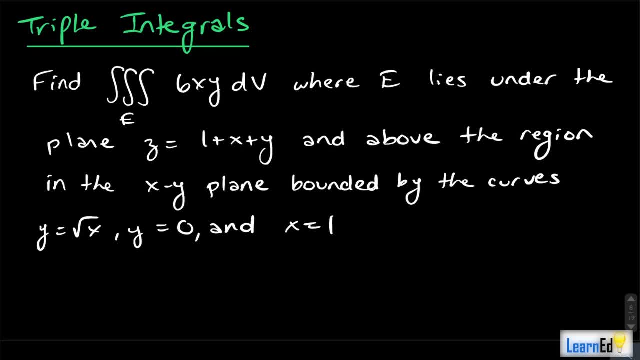 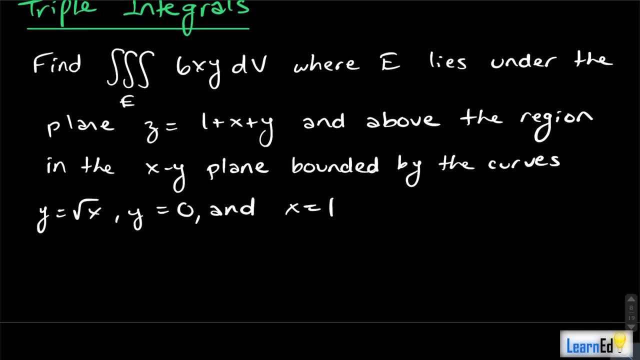 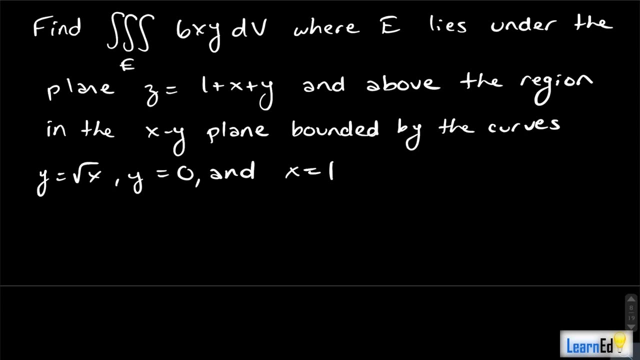 by the curves: y equals the square root of x, y equals zero and x equals one. Okay, so you know, we can see here that we have. you know, our region of integration is going to be some volume. okay, some, some, some volume. we need to find what that volume. 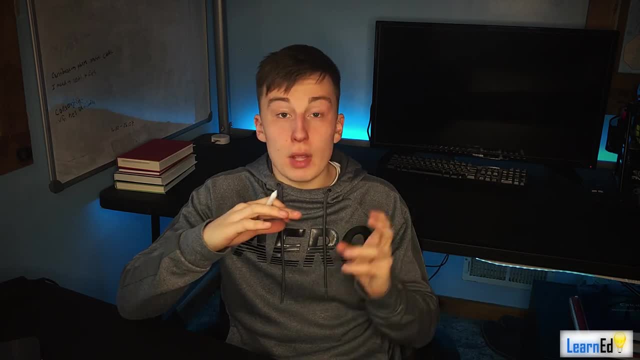 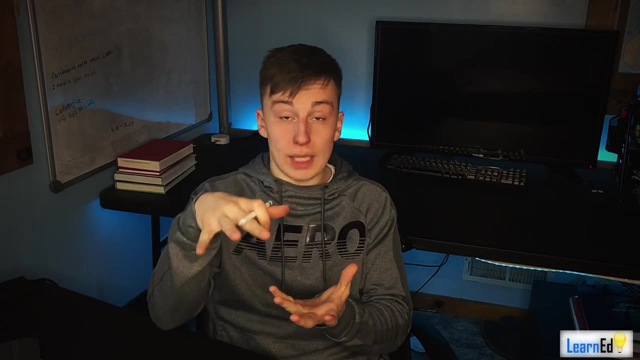 is. We need to find what we can use to replicate that, Okay. So we're going to represent that volume. We have the curves, and these are all in the x- y plane, okay, and we have some surface over top of it. 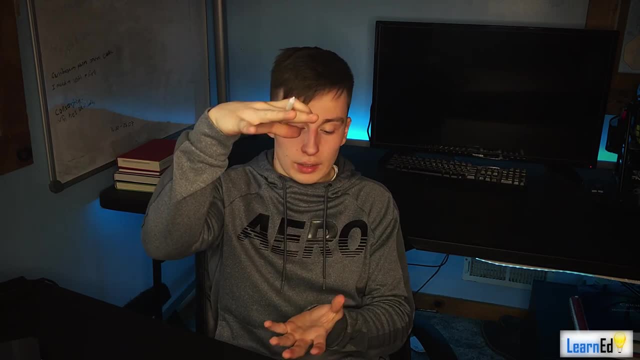 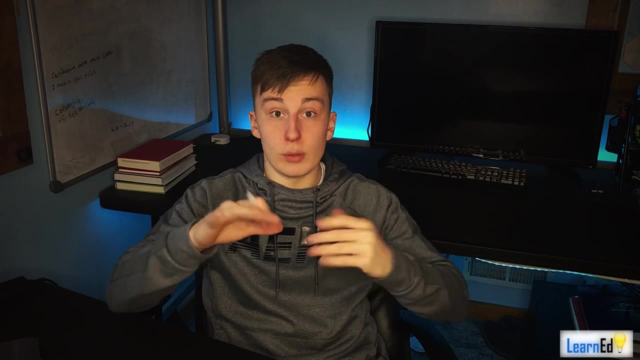 So it's kind of like the double integral setup. We're going to kind of extrude those, those x, y plane curves up and they're going to intersect the surface and that volume is going to be what we use as our bounds for. 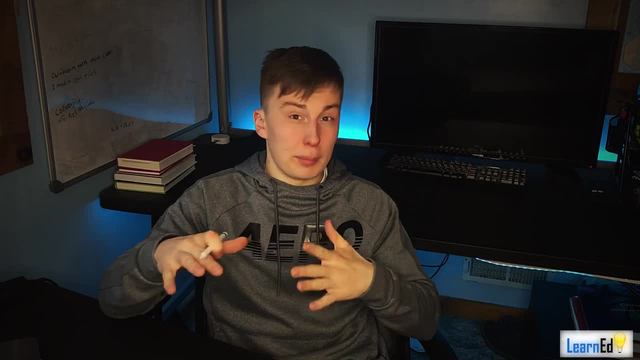 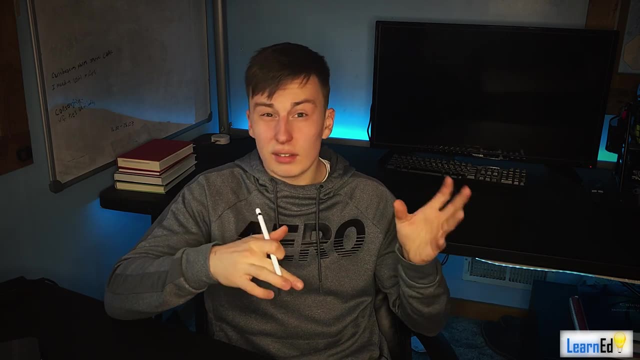 our triple integral. Now remember our integrand that's something completely different. That is, you know, a function of three variables, Meaning it's a, it's a four dimensional deal. okay, so we're not going to be able to really 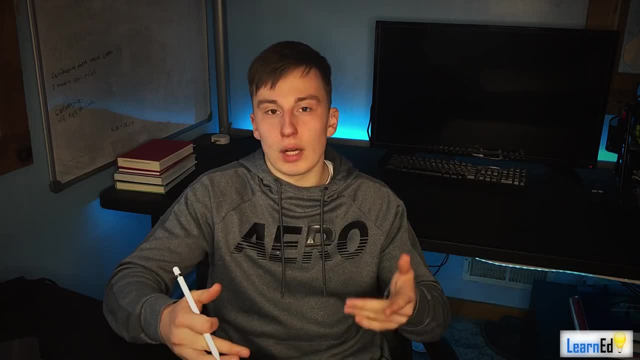 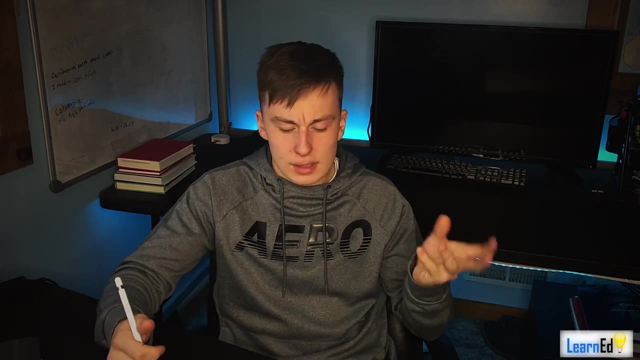 visualize that. We're not going to be able to truly visualize what's going on here unless you use some different, unless you have some other understanding of it, like a density deal, but you know that's. that's a whole different thing. 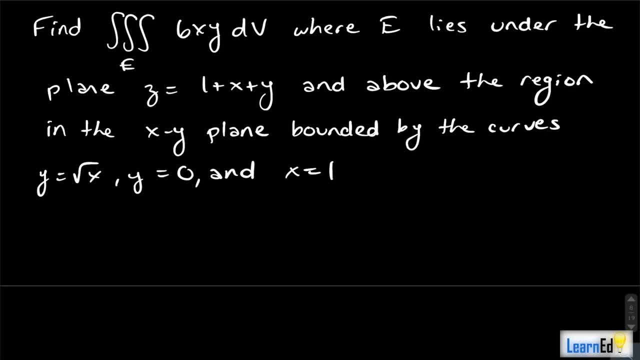 Okay. so now, what we're going to start off by doing. okay, and I mentioned we can't visualize this completely, Okay, But we can try to find our bounds, okay, and that'll you know, that'll be it. 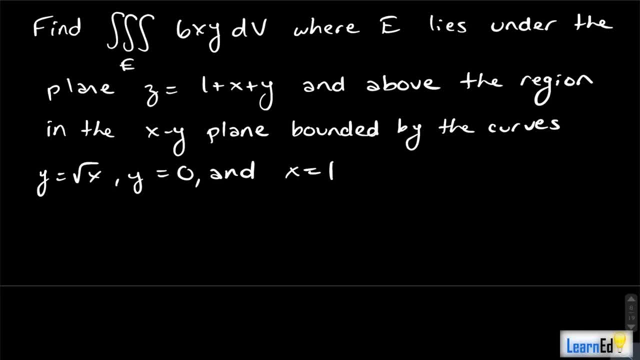 So we can. we can then move on to find our integral. Let's first understand what our our curves in the x y plane look like. Okay, First off, y equals rad x. that looks like that and of course we'll have like that. 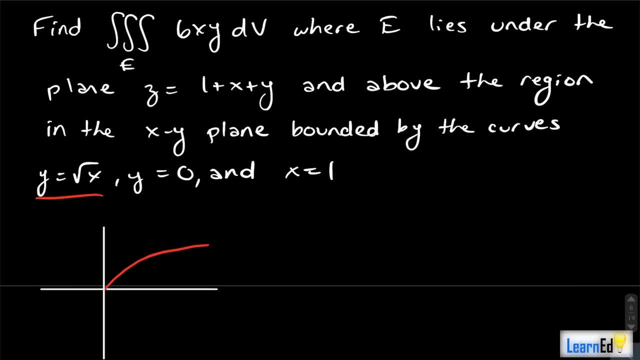 Okay, Actually, sorry, that's not. no, it does not extend down there. We also have y equals zero, Which is just going to be this line right here, And then we have x equals one, which is going to be this line over here. 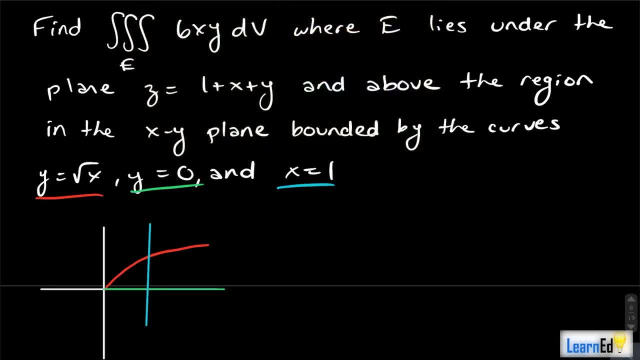 Okay. So when you combine those you have kind of the, the starting point, right. This is just going to be e on the x- y plane, Okay So. so that's the base of our volume. Now we kind of extrude that base up to our surface. 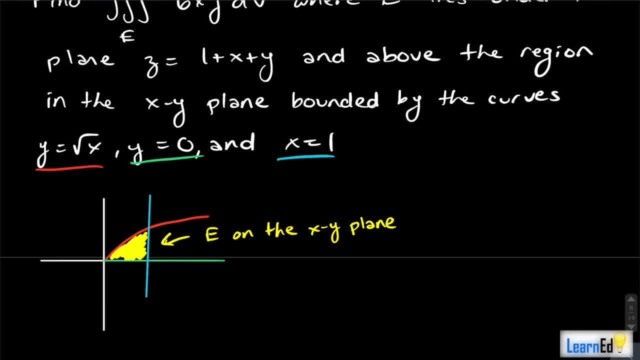 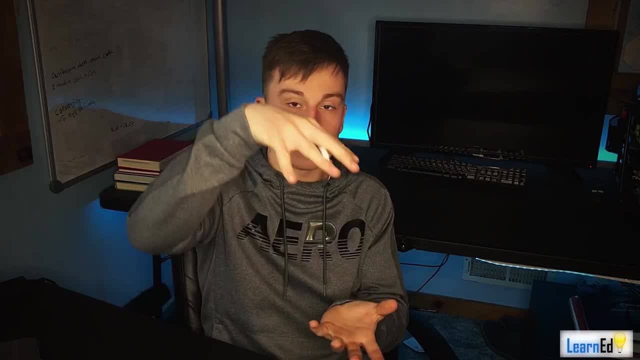 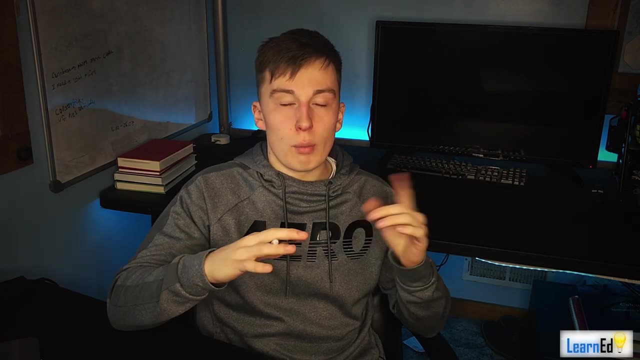 Our surface is one plus x plus y. Okay So, and this is flat, so we can say that our z just starts at zero and extends up to one plus x plus y. Okay So, since that's a, you know, one plus x plus y, that depends on both x and y what we can. 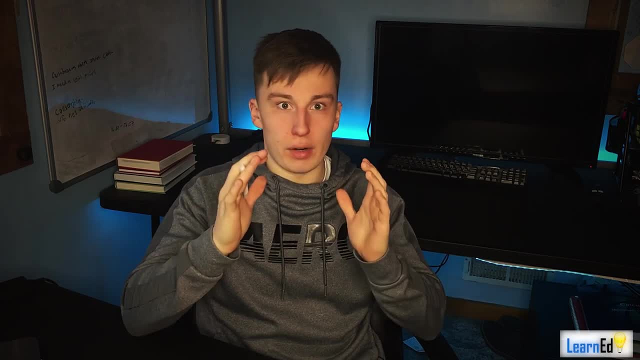 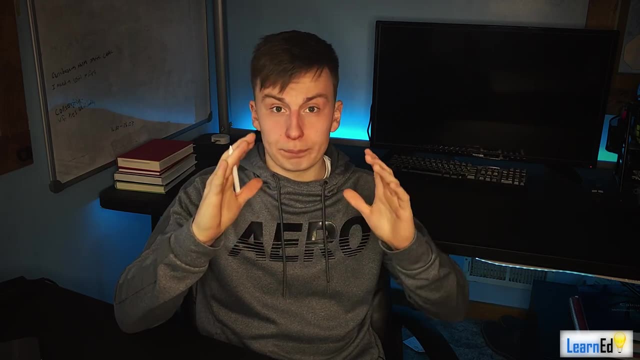 do is have z be our innermost integral. Okay, And just take care of that first. Okay, And that's actually not going to be the worst thing in the world. Our- excuse me- our integral, our integrand rather does not have a z in it. 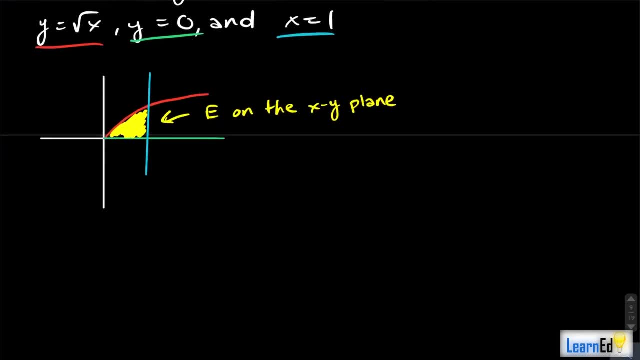 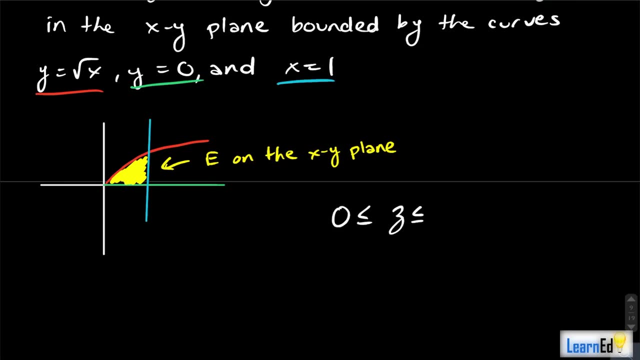 Okay, So it's actually going to be really really nice to take care of that. Okay, So let's figure out our what our other bounds are going to be. Like I said, z is going to be from zero to one plus x plus y. 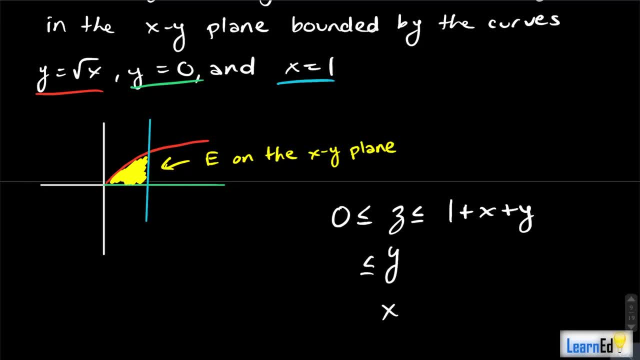 Our y and our x are the other bounds that we need to figure out. Okay, Now it seems pretty easy to me for our x just to be from zero. Okay, To be from zero to one, and then our y to include the curve rad x. 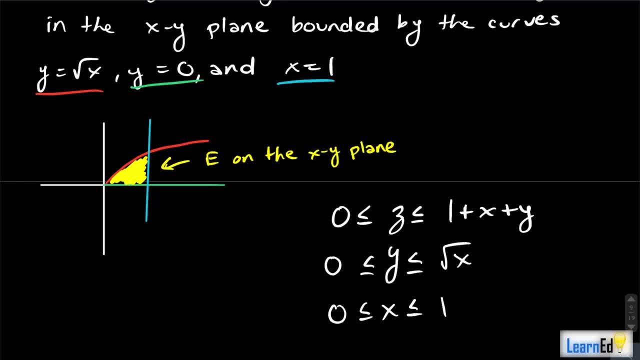 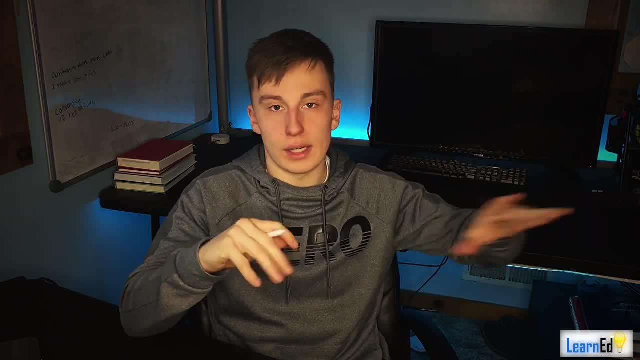 So we can just have y go from zero to rad x, and that way we've taken care of it. So first, what we're going to do is extend y, So let's forget about z. Okay, That's, let's throw that out for a second. 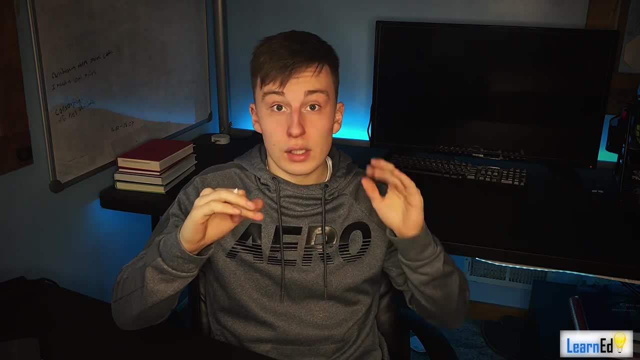 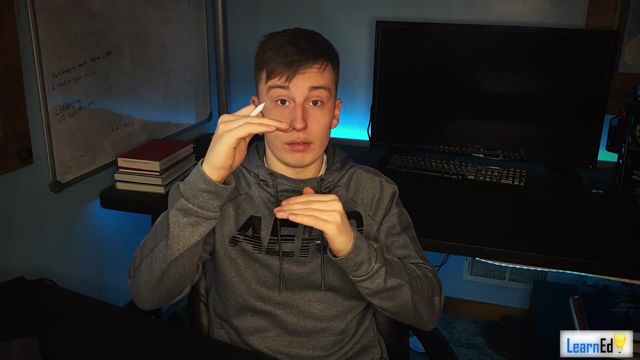 We have just two integrals that we need to focus on: the y one and the x. So for our y, we're integrating from zero to rad x and that takes care of that rad x curve, Okay, That rad x curve Okay. So for that region, 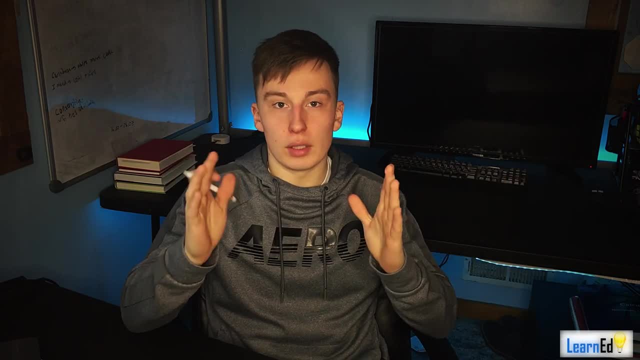 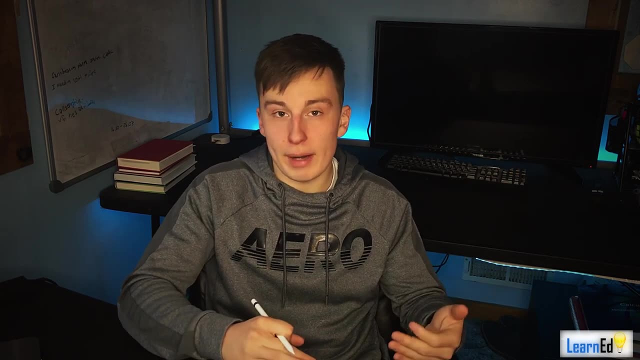 Okay, You know, how much of that region in the x-direction are we going to integrate over? Well, just from zero to one. Okay, Those are just, that's just two straight things. That's not any, you know, any curves or anything that we need to worry about. 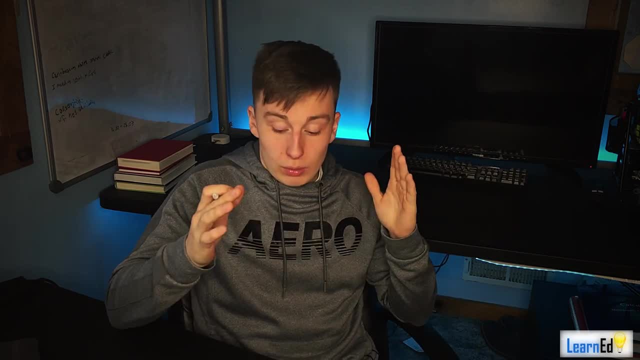 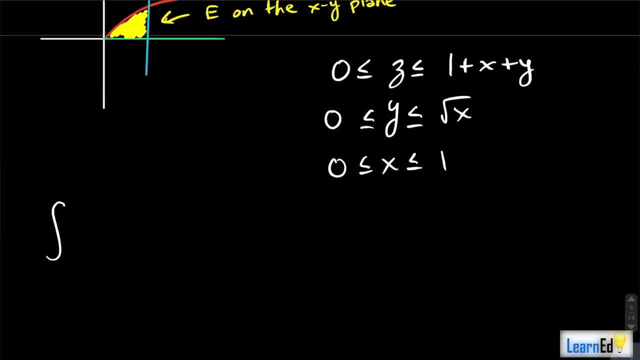 Okay, So that's the idea, All right. So now that we have our bounds, we can just do our integral. Okay, And that's, you know, going to be the probably the easiest part for for most of you at. 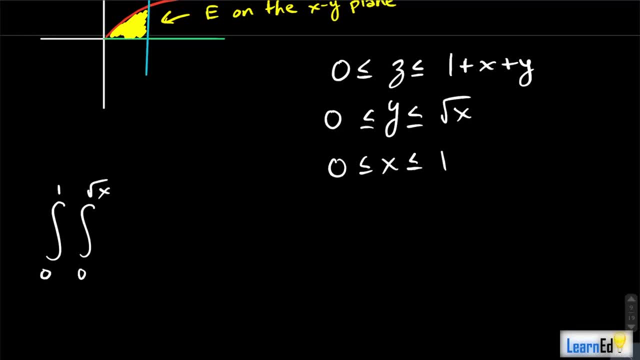 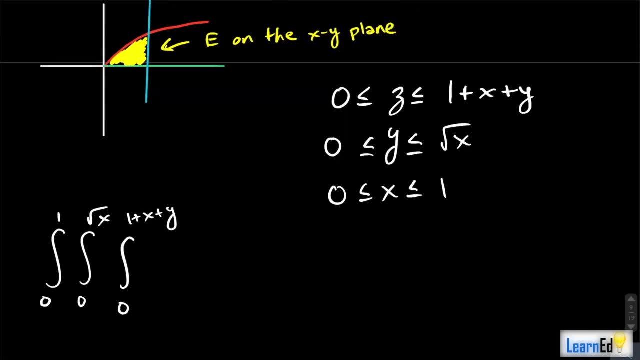 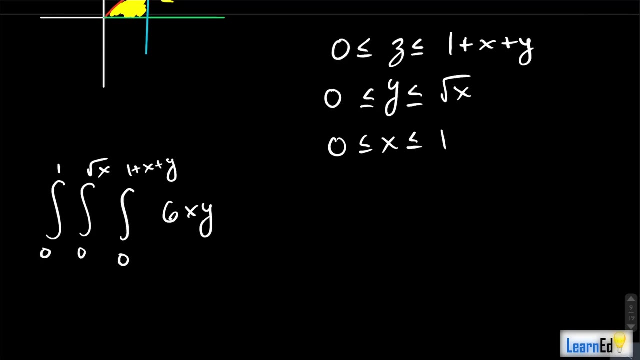 least, at least it was for me, Like I always. you know, the integrals kind of stunk to to uh, to to form, but evaluating them wasn't the the worst thing in the world. So we have six, x, y. our first, our inner integral, is dy. 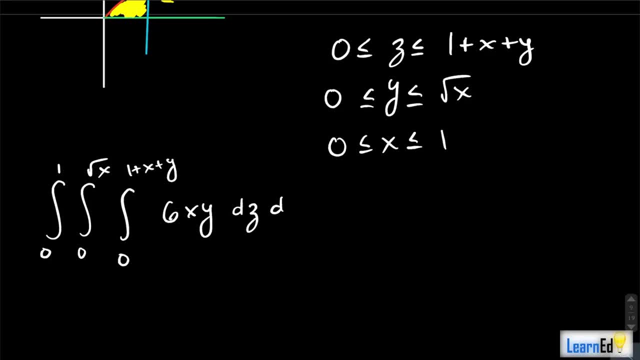 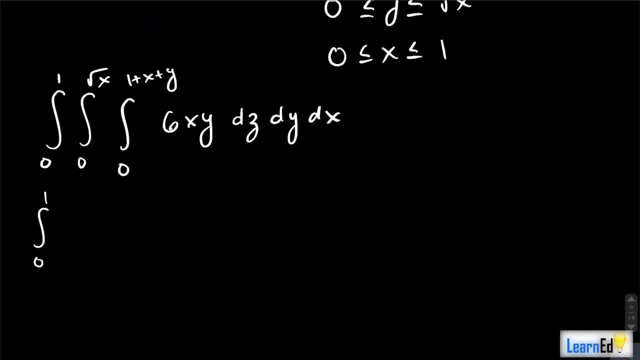 Our second integral is d, sorry, dz. our second integral is dy and then our outer integral is dx. Okay So, First, Okay, So we have zero to one, zero to rad x. We're going to have a six x, y, z evaluated from zero to one plus x plus y. 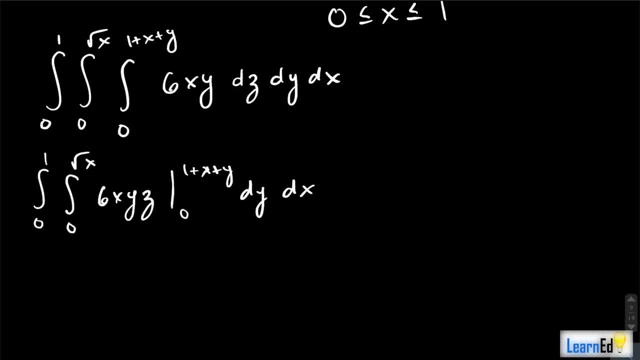 And then we'll have a dy dx. Okay, Plugging that in, we get zero to one, zero to rad x, a six x y times one plus x plus y, which actually what I'll do is I'll just bring these down so we can simplify that. 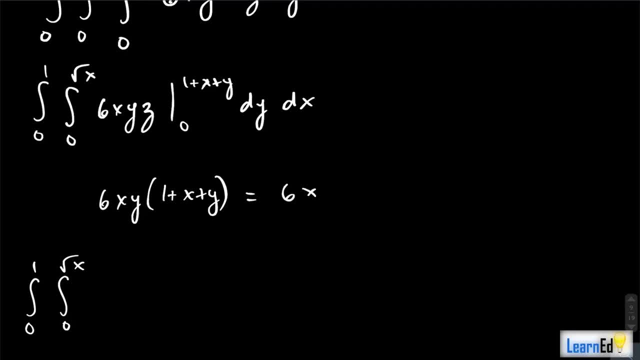 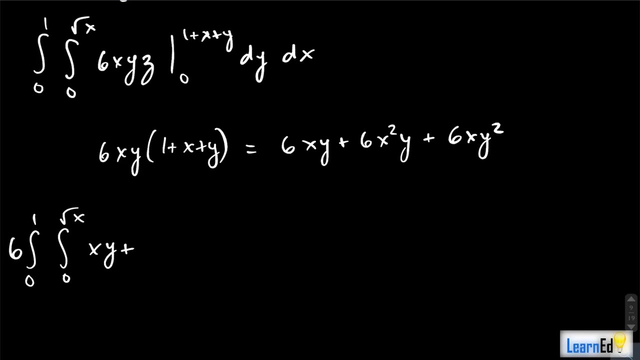 This becomes: Uh, We have six x- y plus six x squared y plus six x y squared. So honestly, we can just get that six out of there and make this a little easier, so we can have six times the integral of x- y. uh, we have x- y- x squared y and x- y squared. 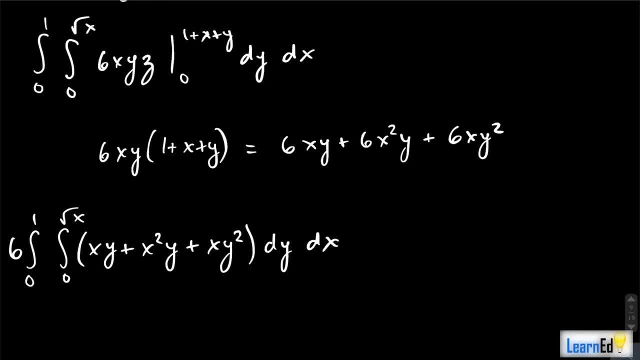 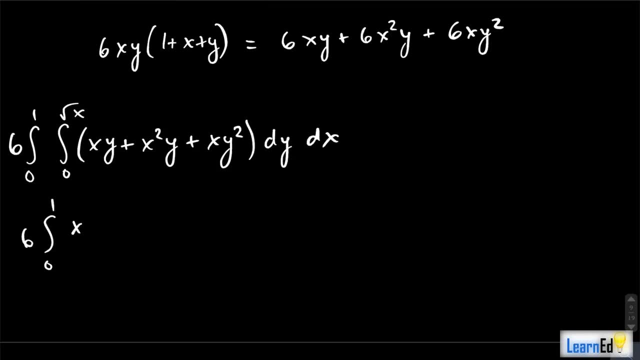 and we have dy dx. Okay, Next we have to integrate with respect to y, So we have six: The integral, from zero to one, of x, y squared over two, plus a x squared y squared over two, plus a x y cubed over three. 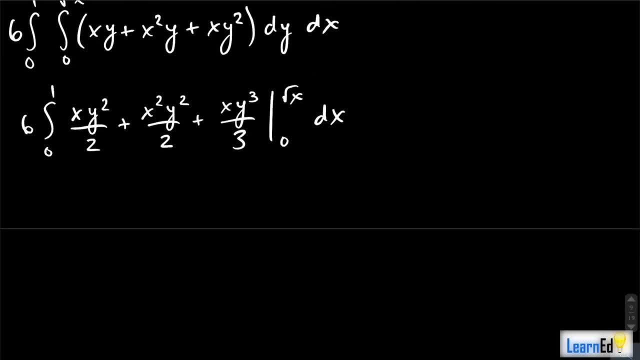 And that's going to be evaluated from zero to rad x. So we have dx. on the end, We get six, the integral from zero to one of that zero doesn't matter, right, Which is, you know, nice. Again, we have that zero in there. 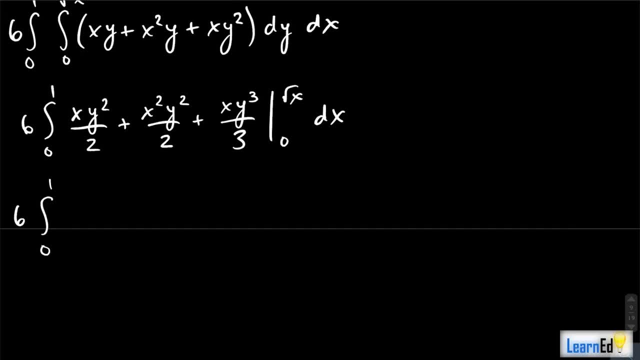 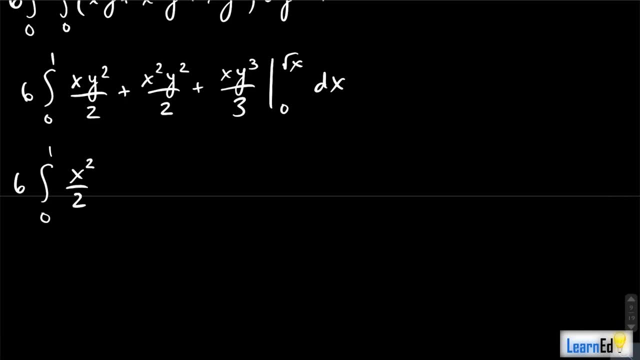 Our rad x does matter. So what we get is a uh x times Okay. Okay, So this will be y squared will be another x, So it'll be x squared over two. We'll have another uh, this will be x cubed over two, right? 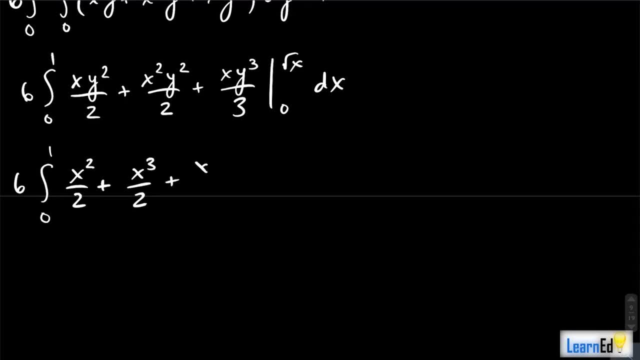 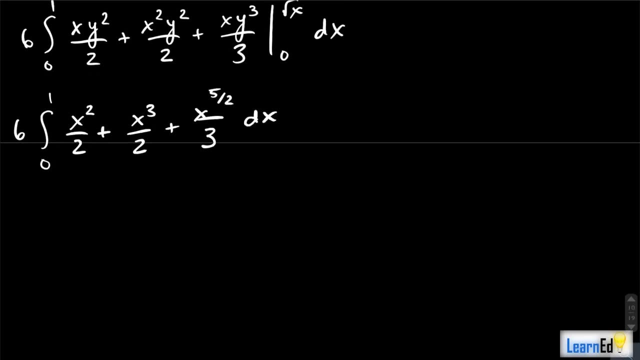 And then we will have a. this one will be a little bit meaner. we'll have x to the five halves over three and we'll have a dx there. but we can just go ahead and integrate this now. This will be x cubed over six plus x. 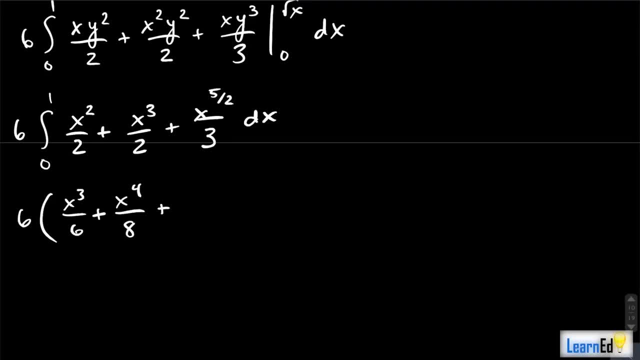 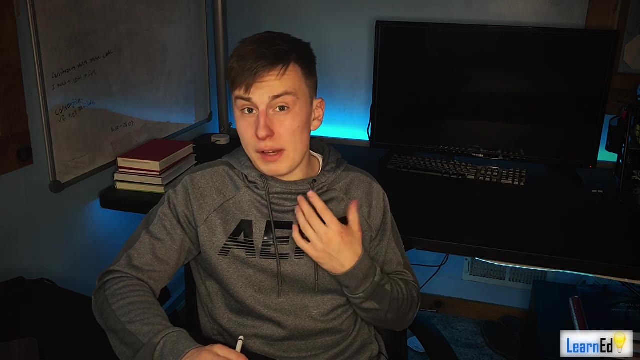 X to the fourth over eight plus we have a x to the seven halves, uh, over three. We'll need to multiply that by a two sevenths and we'll evaluate this whole thing from zero to one. Now I apologize if I'm going a little too fast with these integrals. 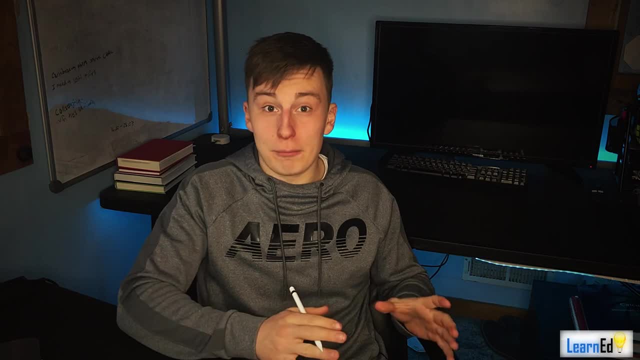 Uh, you know I'm able to fly right through these because I've been doing them for longer than you have. So you know, don't fret if you're not able to do these as fast as me. I'm not, I'm trying. 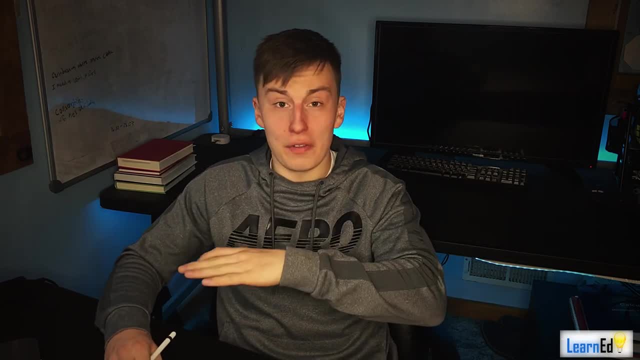 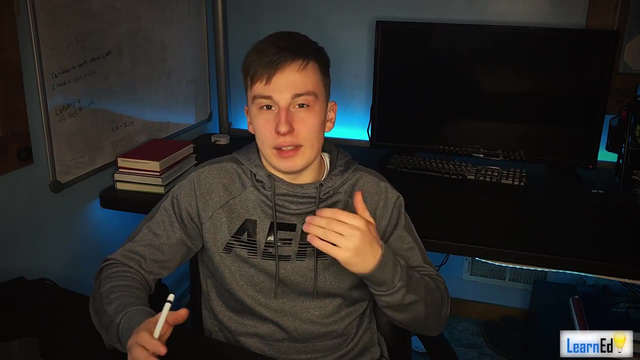 to just get through. Okay, So, uh, you know, uh, all, all the the main calculus, three stuff, and leave the integrals to something you know, you can, you know, not not easily, but uh, easier, Lee evaluate. 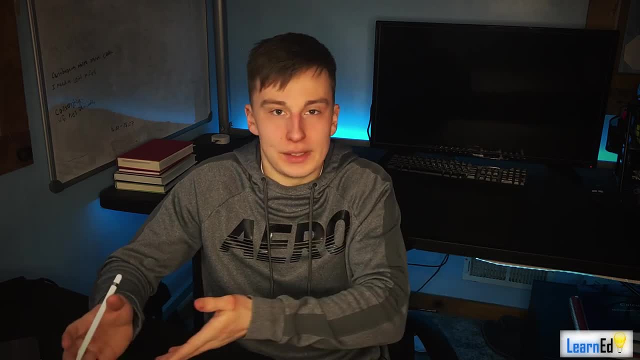 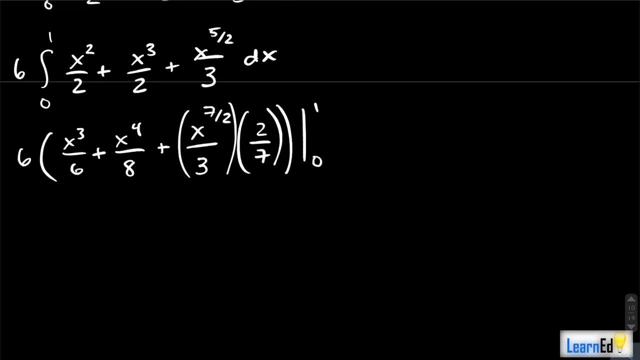 All right- I don't know what the word is for that. It's going to be easier to evaluate the integrals than it is to set up the integrals, So I'm trying to focus more of my time on the setup, All right. 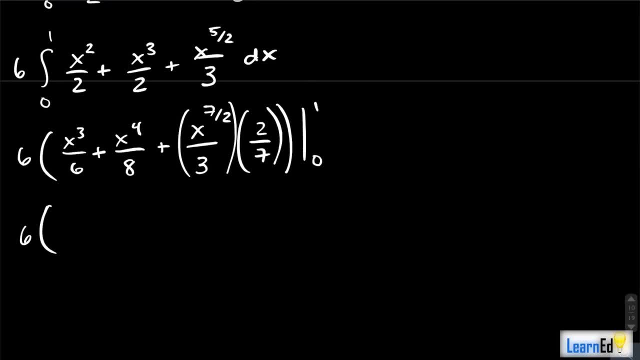 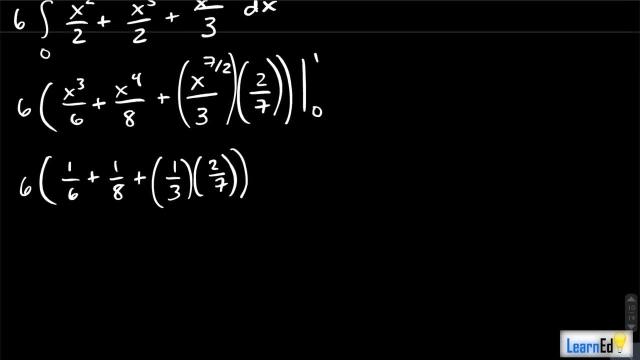 So we have a six times the. all the X's just end up going away. And well, we'll just have like a one sixth plus one eighth, plus a one third times two sevenths, which we'll end up just giving you a six times. uh, actually, no, I'm done with. 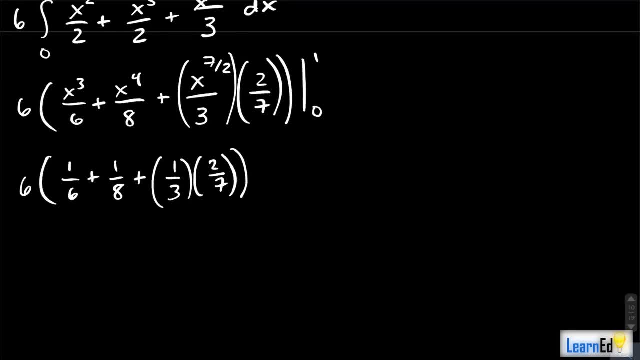 this. This is, we're good. I'm just going to give you the answer here, because I'm not spending time simplifying this. I don't want to 65 over 28.. All right, That should be your answer, Okay, Nice. 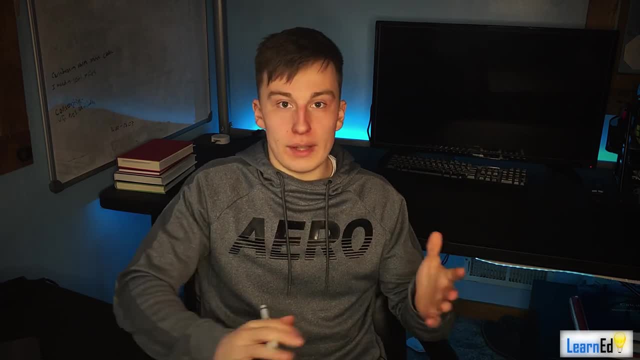 You did it Right. All right, So that's triple integrals. Okay, That's, in a nutshell, what you're going to have to be doing. Uh, you know, you may get some problems that are a little bit more challenging than that. 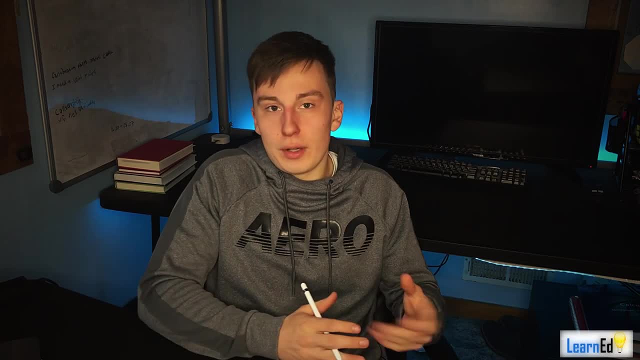 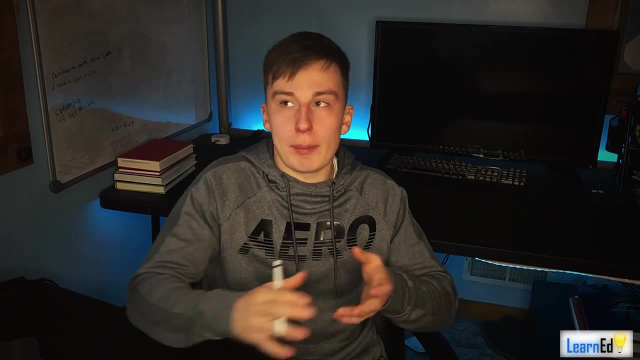 one. but uh, you know, if you get a triple integral that's more challenging, uh, then you're most likely going to be getting a double integral That's less challenging, or you might be getting a cylindrical, uh, a cylindrical coordinates. 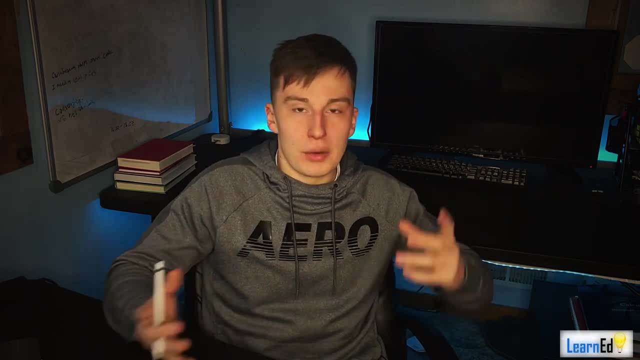 problem That's less challenging, or spherical coordinates problem That's less challenging. You know things are going to start to offset when you're going to take a test. That's how tests are made right. They always have that time factor in mind. 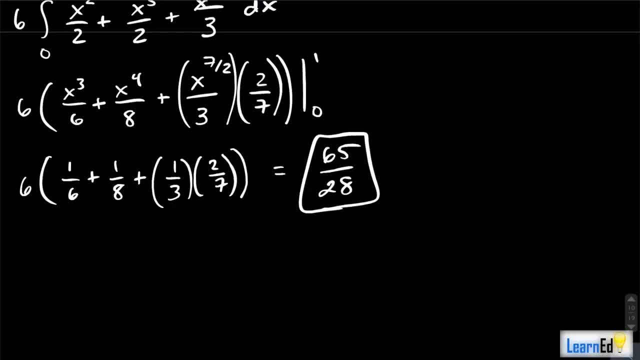 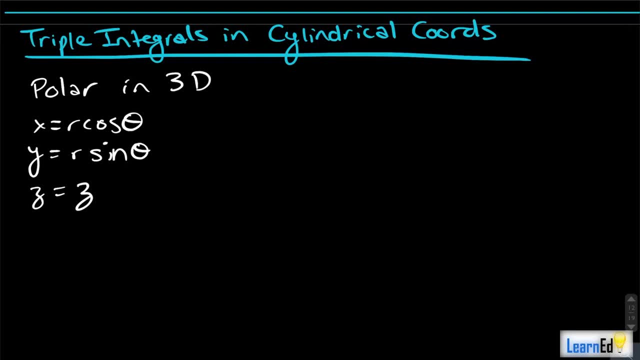 Well, I can say that for most people, All right. Triple integrals in cylindrical coordinates is our next stop. Okay, Basically, cylindrical coordinates, that's polar and three dimensions. So you keep the X equals R cosine data, You keep the Y equals R sine data, and now you're just adding the Z. 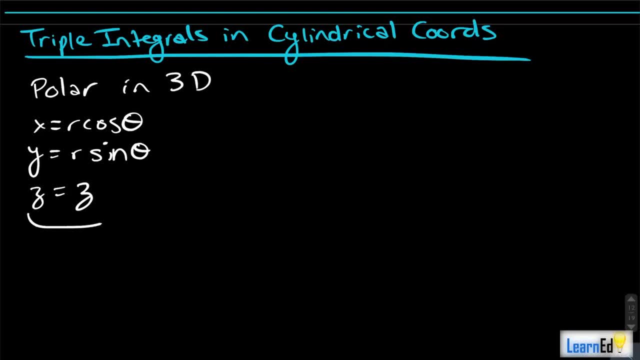 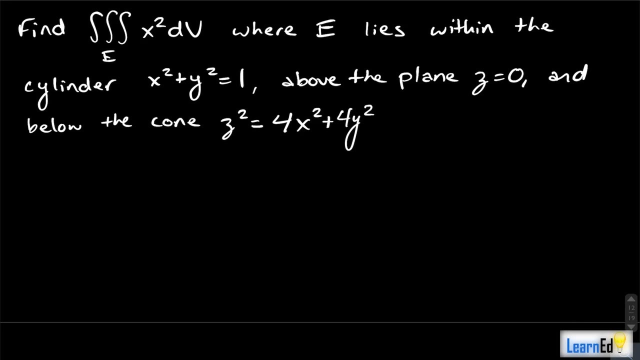 So you're kind of extruding polar into the third dimension, which would give you a cylinder, right? So Z equals Z, All right. So our problem here is that we want to find the triple integral over some volume, E of X squared DV, where E lies within the cylinder. X squared plus Y squared equals one and above. 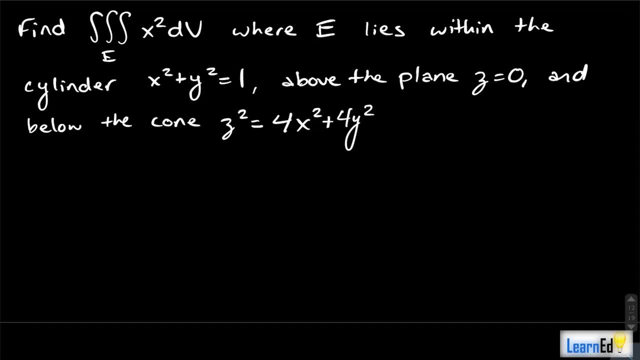 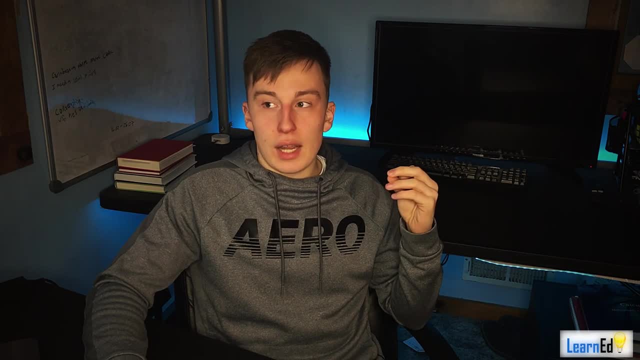 the plane, Z equals zero and below the cone, Z squared equals four X squared plus four Y squared. Now you can't count on them to be that nice and and say that it's a cone. Okay, They might not say that it's a cone. 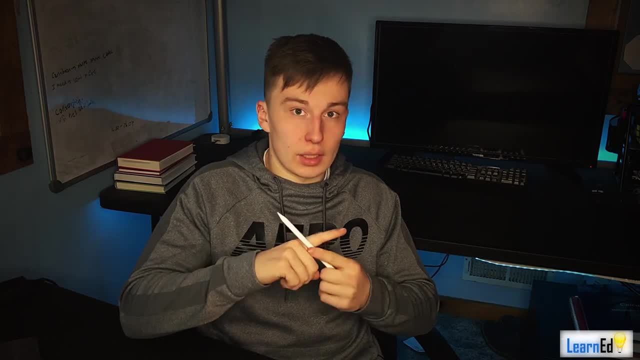 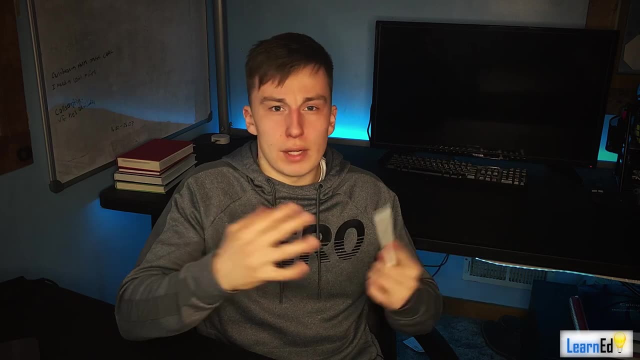 You might have to figure that out And you know, if you don't know Automatically that that's a cone, you can figure it out by doing traces. Remember doing traces earlier in calculus three. you know like level curves you might've. 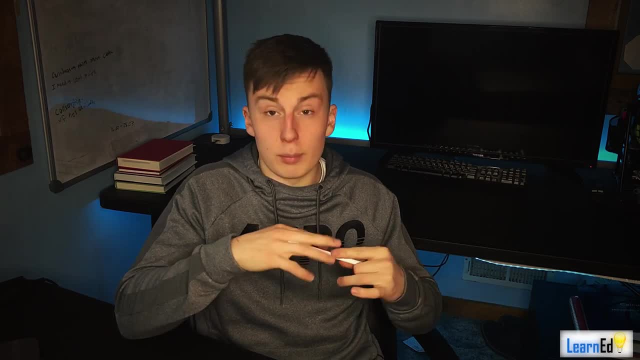 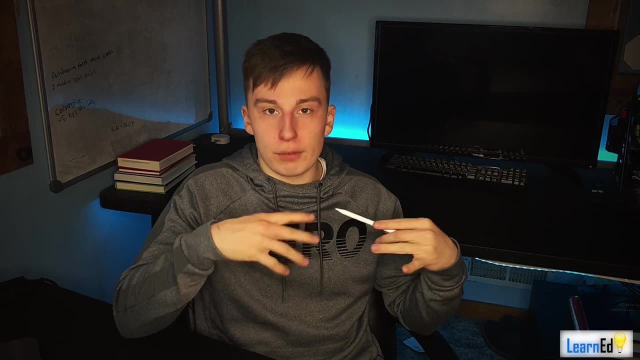 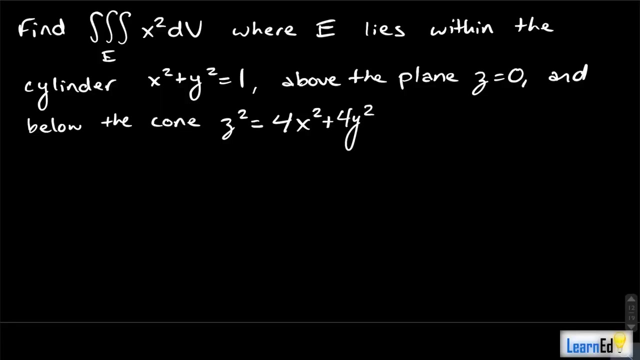 heard of it like that. I don't really know exactly the term terminology that you guys used in your calculus three classes, but you know, just be ready for something like that, Be ready for them to throw a curve ball. Maybe they don't call it a cone and you have to figure out that it is indeed a cone. 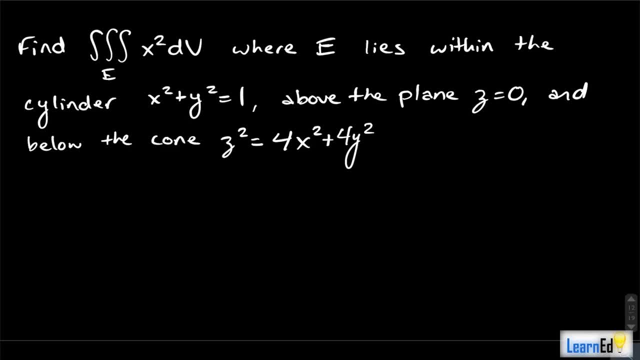 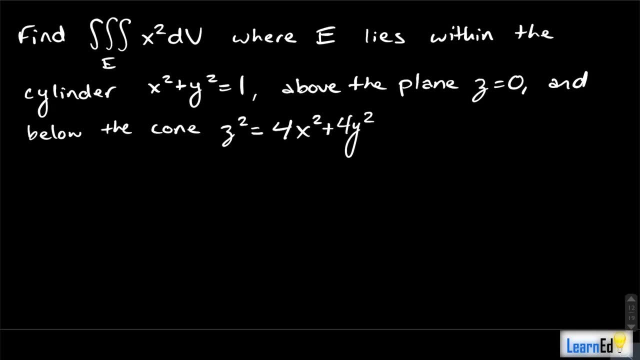 Okay, So we're above the plane. Z equals zero, So that's nice, We think positive here And really all we have to do again is figure out our bounds. So how do we figure out our bounds? We have to graph this thing in three dimensions and figure out what this region is. 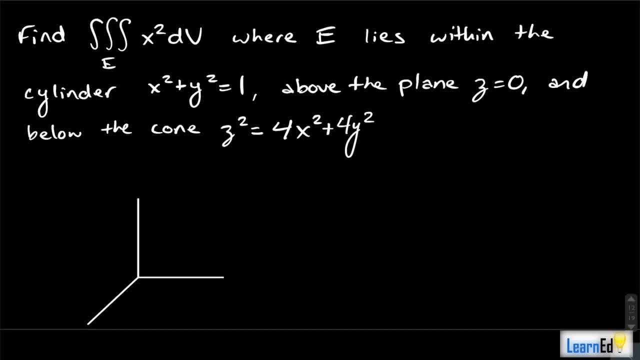 And then we find our bounds, the bounds of that region. Okay, We have X squared plus Y squared equals one. So I'll graph that in blue. That'll be the cylinder right here, We'll go up. Okay, So we have X squared plus Y squared equals one. 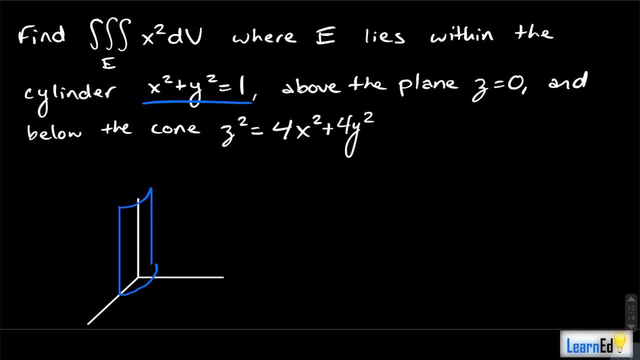 So I'll graph that in blue. That'll be the cylinder right here. Try to make it look a little bit nicer. but you know what? Yeah, Art students give me tips. What do I do when I mess up like that? 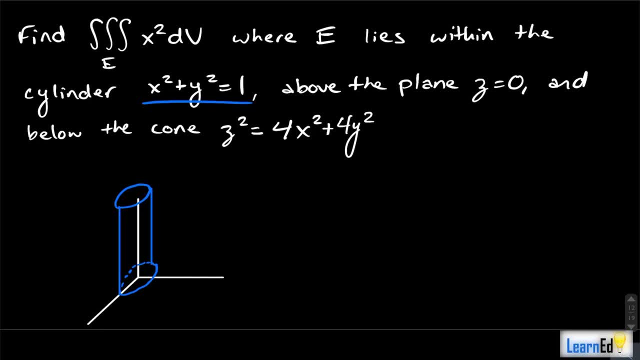 How do I draw cylinders? We're above the plane. Z equals zero, So this is all positive And we have: Z squared equals four X squared plus four Y squared. This cone, excuse me feeling a little bit under the weather today. Okay. 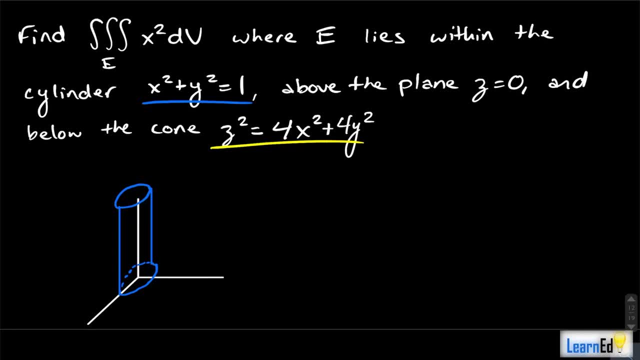 We will. what we'll do is we can just kind of use some level curves to figure out what this looks like. as equals zero. We get that four X squared plus four of Y squared. The only way for this to be true is for X and Y to both be zero. 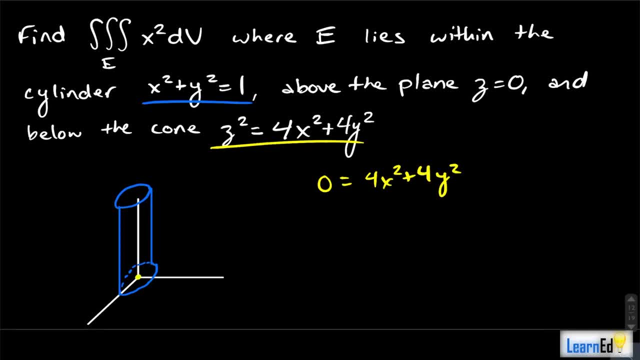 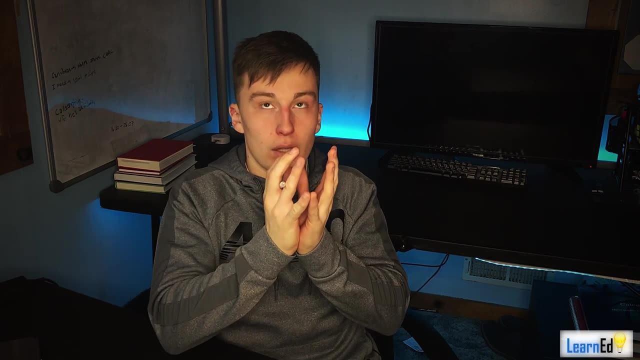 So we'll start at the origin and then when will these guys actually be intersecting the, the cylinder? So, since this cone has, you know, four X squared, Okay, And four Y squared, We know the cones like, it's not like elliptic on the inside, necessarily it'll be like circular. 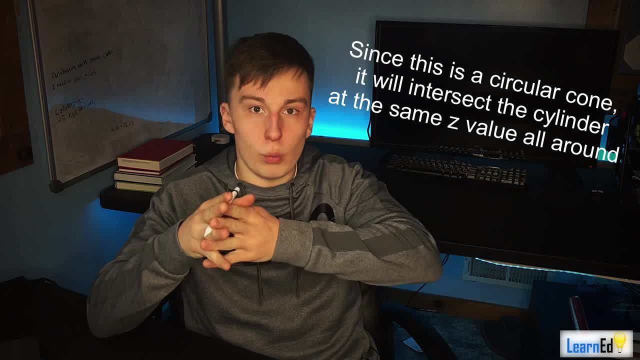 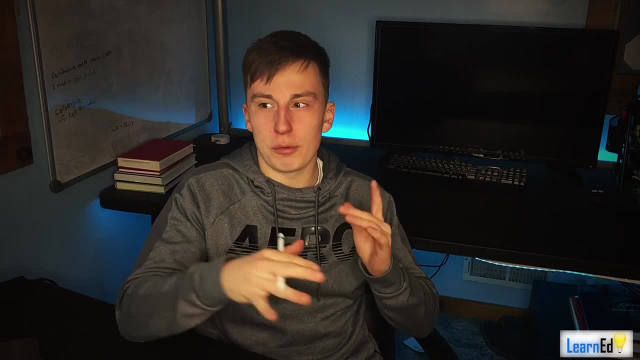 cross sections of that cone. Okay, If it was like four X squared and two Y squared, or those coefficients were different, then you know it's elliptic as the level curves, if that makes any sense. I don't want to really overwhelm me with all this quadric surface terminology, but it is. 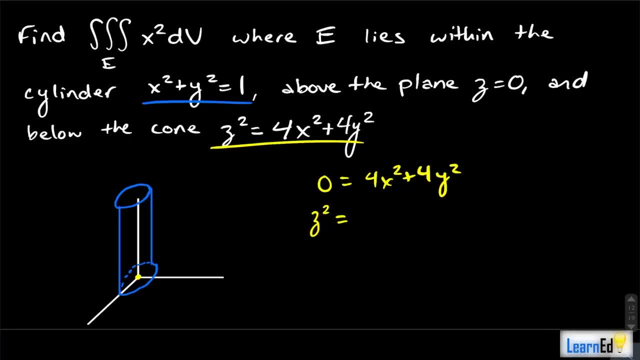 something that you should know. for your final, Let's just try to find the Z value, since we know it's going to be the same all around. Okay, And we just are at the point of X equaling one and Y equaling zero. 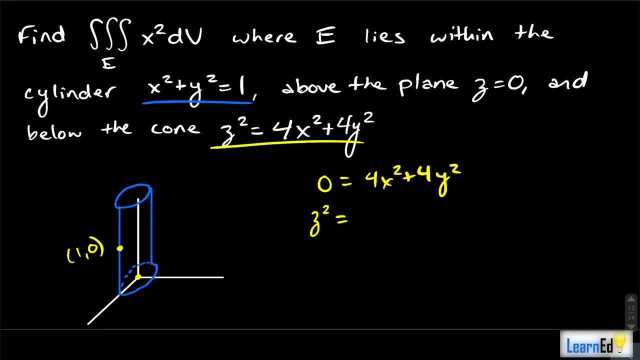 We know that this is a point on the cylinder, because we know that this point right here is one zero, zero. and we know that this point here is zero, one zero. Okay, So we know it's one zero going all the way up. 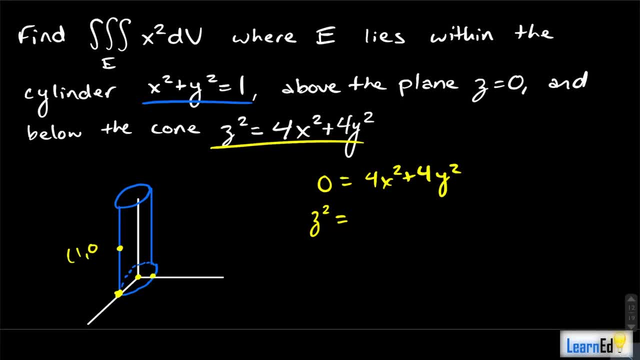 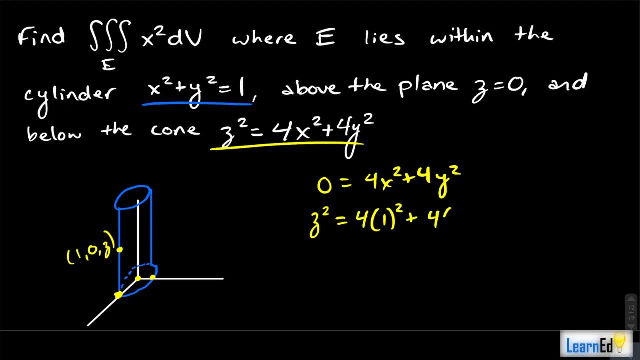 So now the question here is: what's the Z value? Okay, So Z squared equals four times one. Okay, One squared. And then we have our Y coordinate, zero. So we get Z squared equals four, which means Z equals two, not minus two, because we're 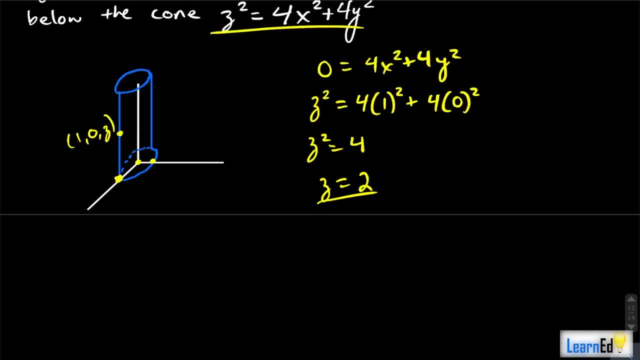 dealing with above the plane. So now that we know that Z equals two, what we can do here is label this point, and I don't want to want to label this down here. one zero two Okay. And that means at this point over here, where the cone will also go up to an intersect, will. 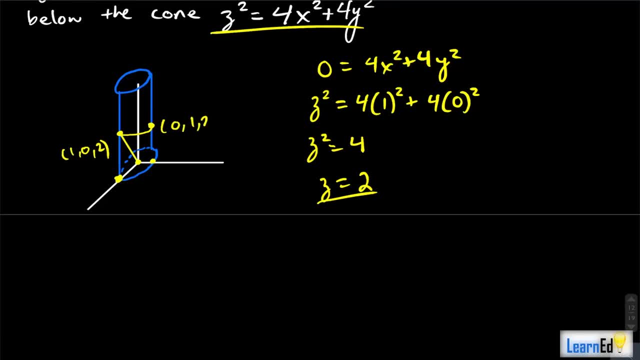 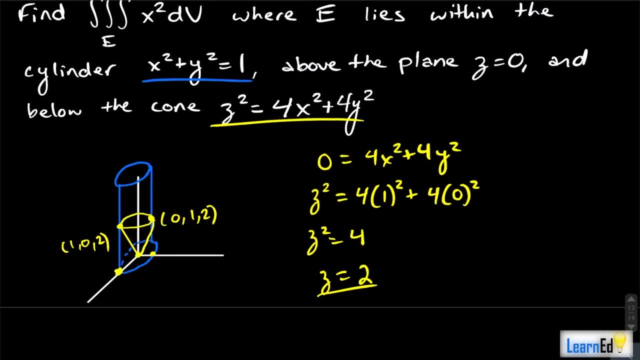 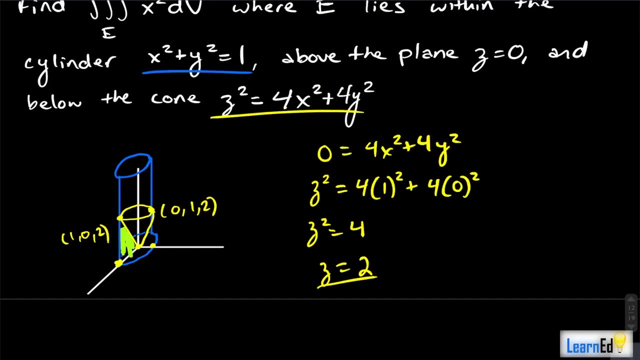 be not one, it'll be zero, one, two and that'll extend around and that's your cone. But you want to find the E. okay, is the volume below that cone. So that's kind of like this surrounding volume here. 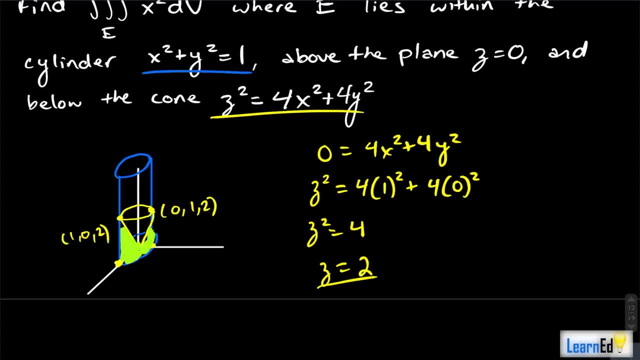 Okay, It's kind of actually just going to come up around the cone on the outside there, Okay, So that's what E is All right. So now, what we're going to do is, well, we're going to represent this using cylindrical. 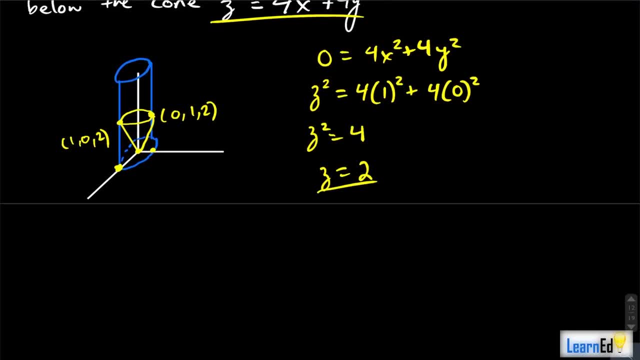 coordinates. because you know, let's face it, how are we, how else are we going to take care of of these curves? Okay, First off, think about what our theta bounds will be. Okay, That's the easiest one to start off with. 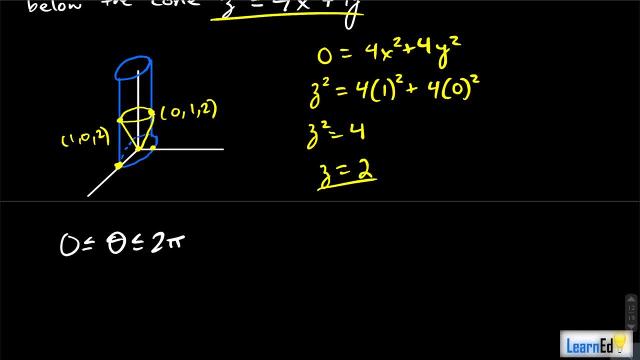 Theta is going to go from zero to two pi, because the cylinder sitting right in the center Now our Z bounds are probably going to be the hardest. We'll save them for last. Our R bounds, well, R is just going from zero to one right. 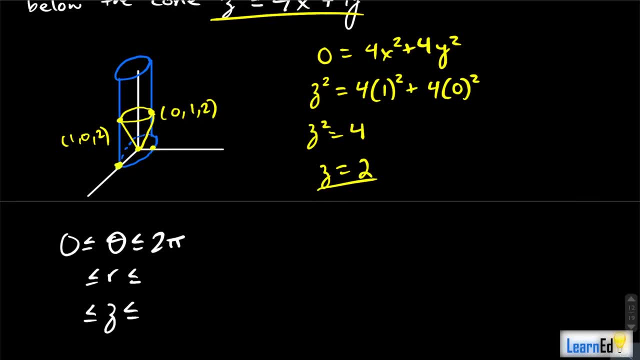 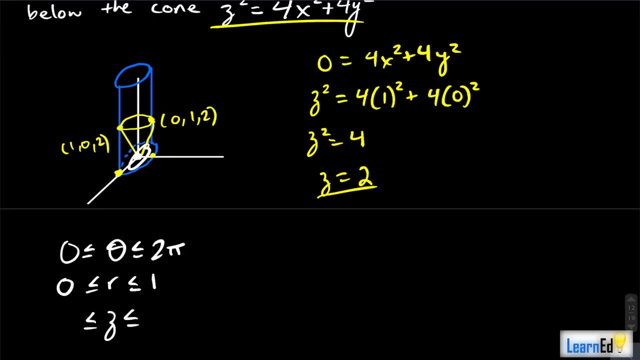 One here, one here, one here. Okay, So R goes from zero to one, The Z, we know it starts at zero. right, It starts universally at zero on the flat of that cylinder, But where does it go up to? 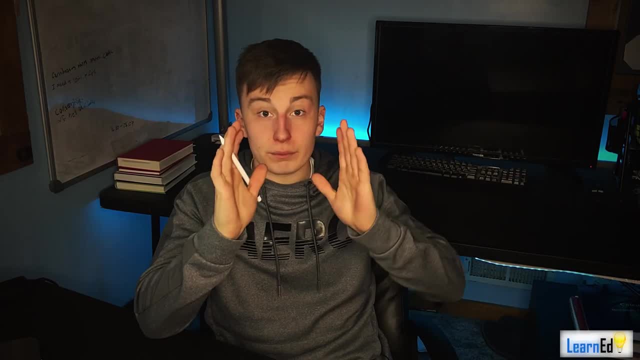 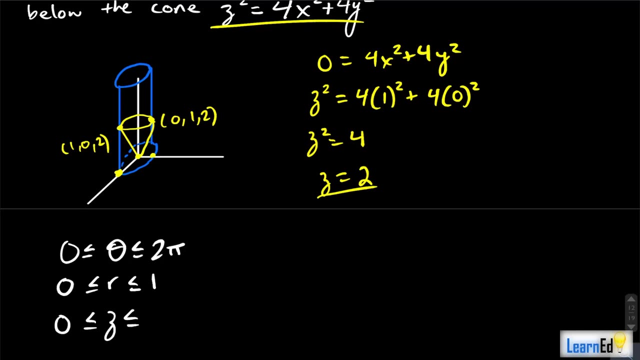 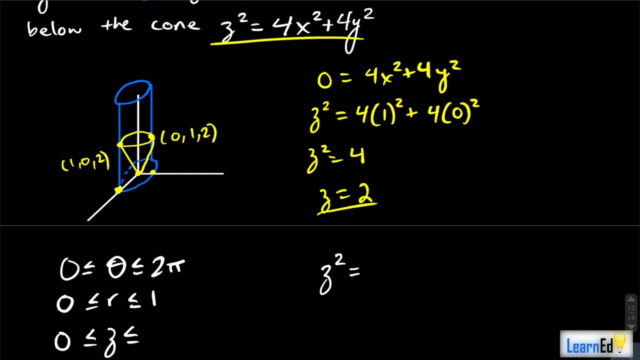 This is where the bottom of that, the cone, That's where that takes effect in this top Z bound here. How do we represent that? Well, let's just talk about the cone as being in polar coordinates: Z squared equals four times R squared cosine, squared theta, plus four times R squared sine. 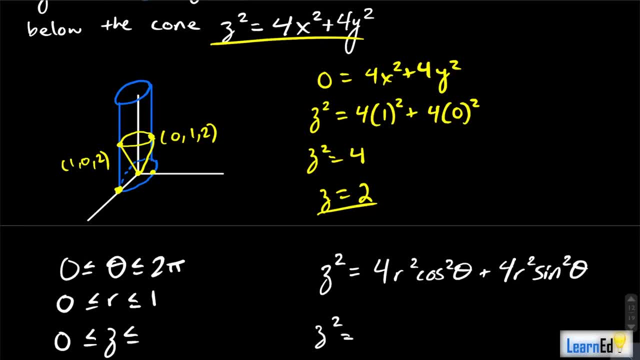 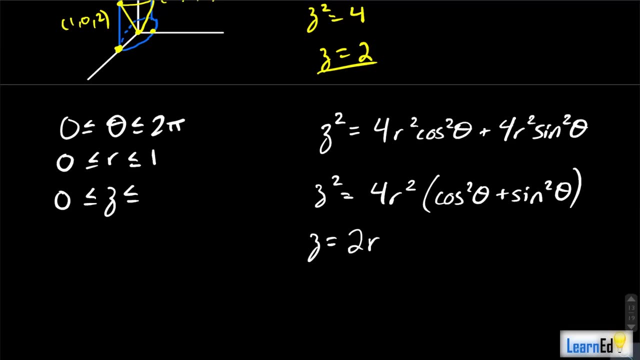 squared theta, This means that Z squared is equal to four times. well, actually I'll also factor out the R squared, and then we have times: cosine squared theta plus sine squared theta, Z equals two R. That's what we get when we simplify that all down. 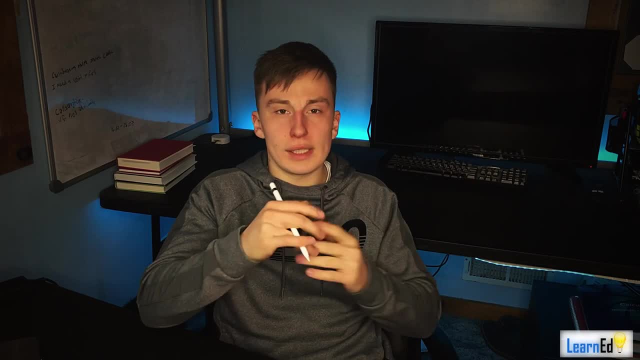 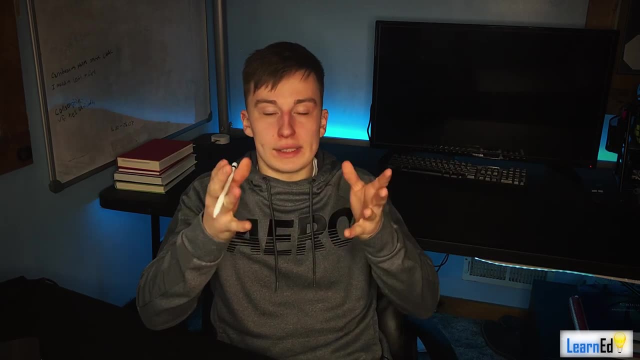 So that's going to be our top bound of Z, right? If you're struggling to kind of visualize that, the cone- okay, there's nothing inside the cone that you have to worry about. That cone is just hollow. The cone itself is defined by: Z equals two R. So that's our top bound, okay. 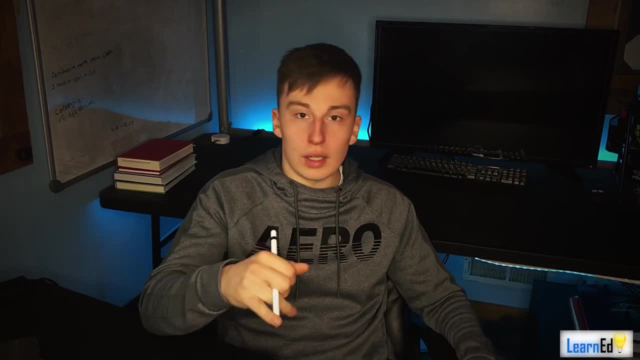 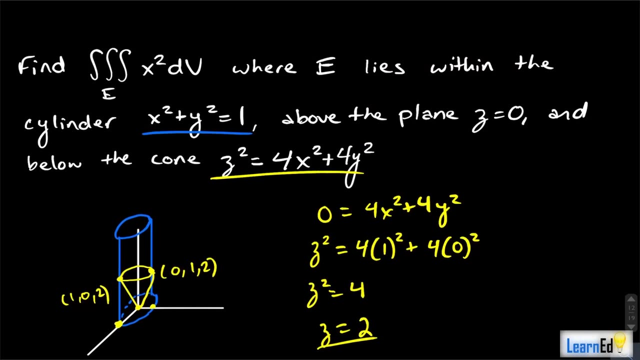 That's how we're taking into consideration the cone. Now my dog's here, All right, going to lay with me during the video, Cool. So now that we have our bounds, all that's left to do is translate our integrand or. 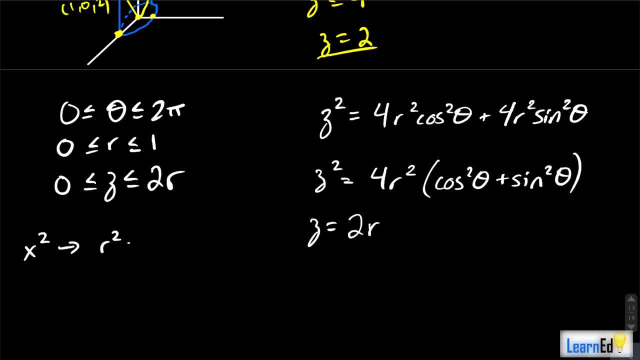 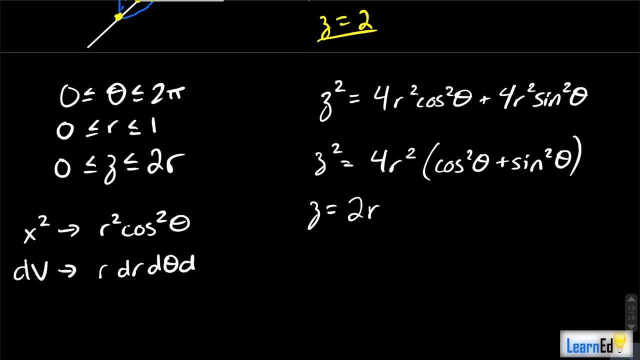 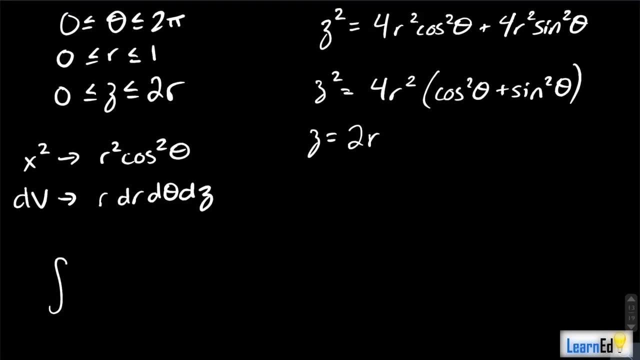 X squared into polar, which just means it's going to be R squared cosine squared theta, and our DV is going to be R dr d theta, dz, which means that altogether we're going to have the triple integral. We're going to have the integral from zero to two pi. 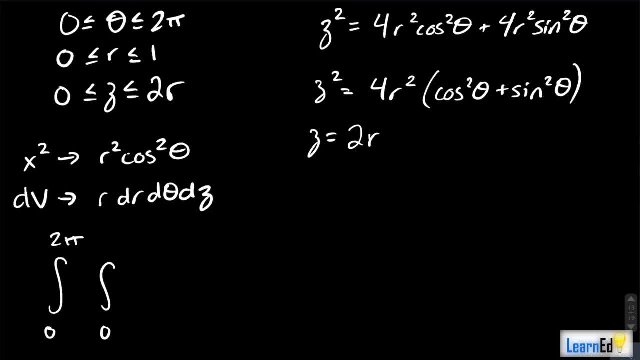 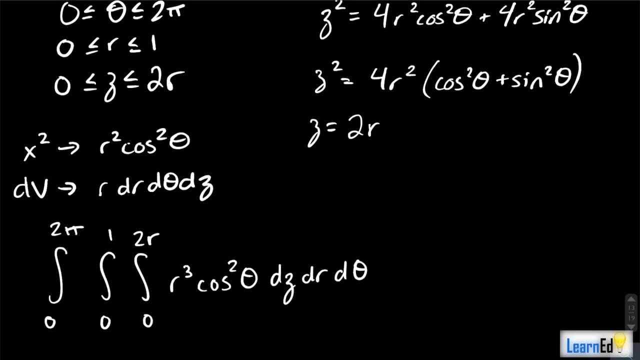 All right, We're going to have the integral from zero to one, and we're going to have the integral from zero to two: R of R, cubed cosine squared theta, And it's going to be dz dr, d theta, And so we have zero to two, pi zero to one. 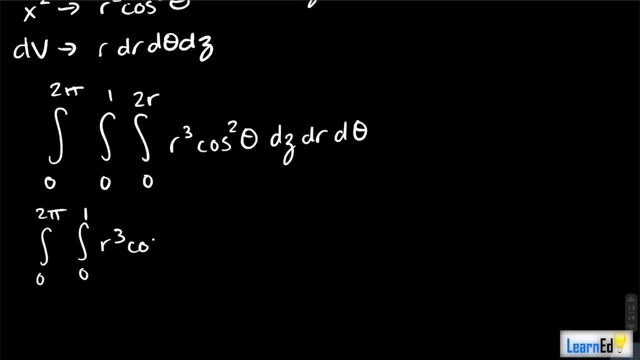 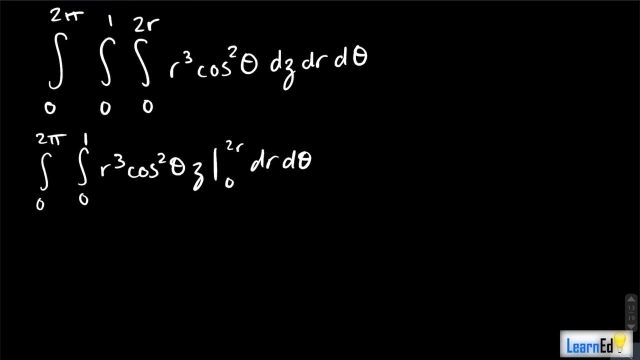 We do our first integral here, That's R cubed cosine squared theta z, evaluated from zero to two: R dz, dr d theta, No problem, Not dz. Okay, Dr d theta, and we evaluate this integral: zero to two pi, zero to one. 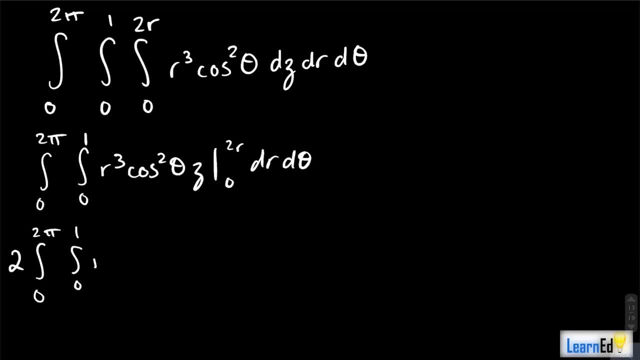 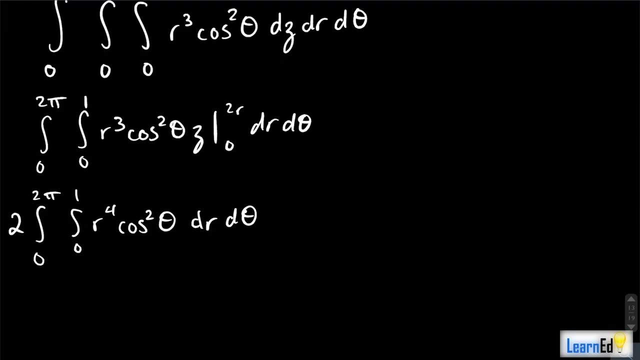 We'll pull the two out because we're going to get a R to the fourth cosine, squared theta. Okay, So stop texting me people. Geez, I'm too popular. All right, Now we have dr d theta, And these we can split apart because they're not dependent on each other. 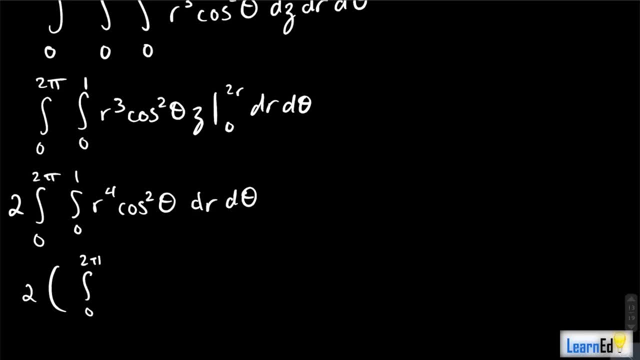 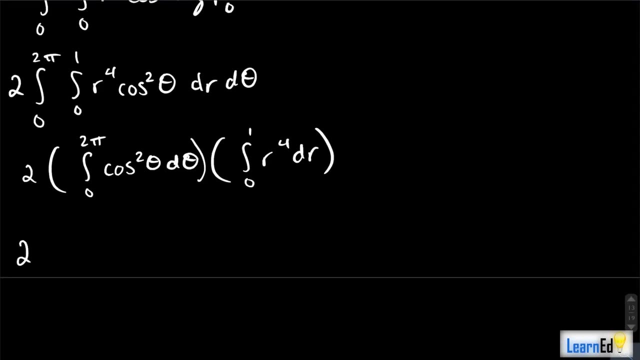 So we can go ahead and just go zero to two pi of cosine squared theta d theta, And then we can do zero to one of R to the fourth dr. Okay, So we have two times the integral, two pi One plus We'll have a cosine of two theta over two. 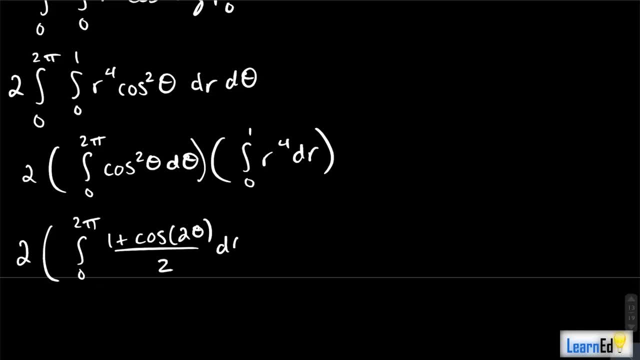 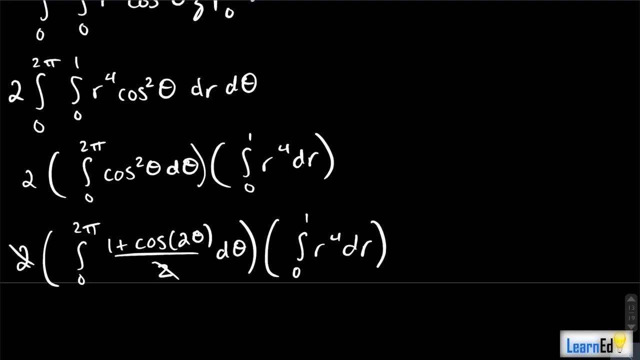 And that'll be d theta Now that two is going to cancel off with the two out here, So that's going to be really nice And we have the integral from zero to one, of R to the fourth dr. I don't want to go through and integrate that yet just because we haven't done the other. 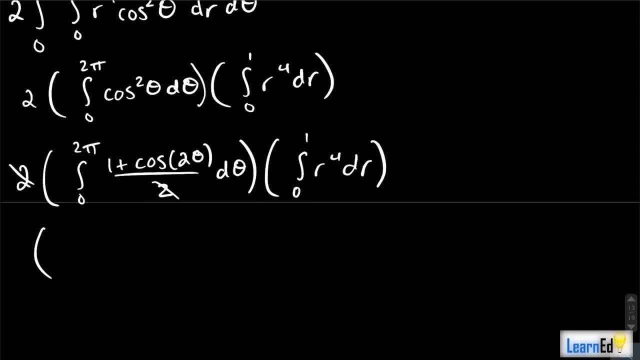 one yet. So it's going to be nice. and even So we have theta plus sine of two, theta Over two, evaluated from zero to two. pi All right. And now we're going to have R to the fifth over five, zero to one. 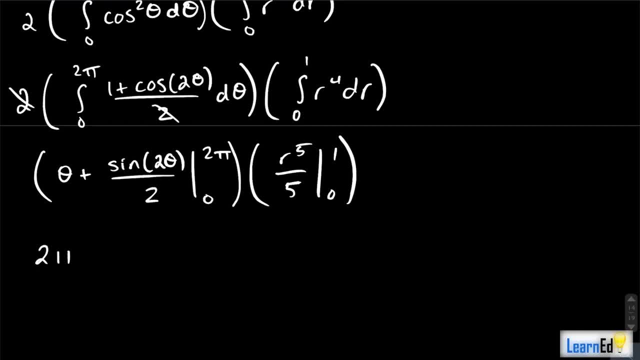 So what we get here is two pi plus we're just going to get the sine goes away, because the two pi and the zero are both going to get rid of that. So we have a two pi from that, Okay, And then from R to the fifth over five, we're just going to get a one fifth. 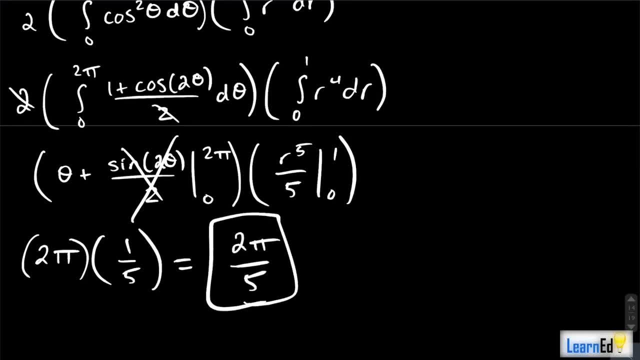 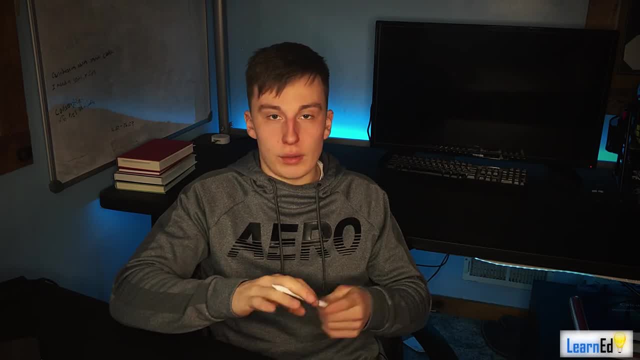 So our final answer is two pi over five. All right, And that is you know, kind of it for cylindrical coordinates. Okay, So you're kind of going to know when you have cylindrical coordinates, because you'll have something that's cylinder like it. 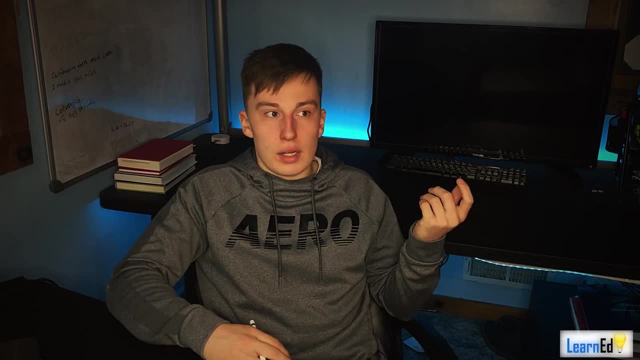 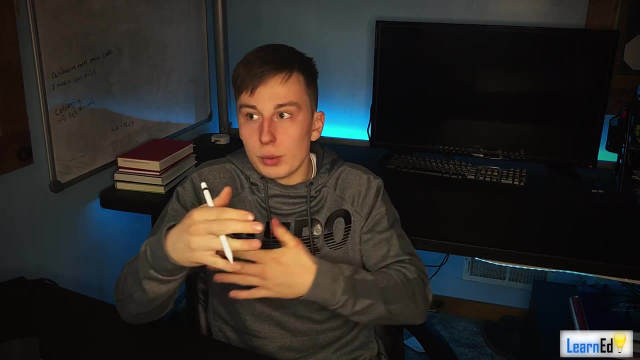 You're mostly likely going to have a cylinder in the problem first off, And if you have things you know, like a cone, like that's great for spherical coordinates. Okay, We were able to define the curve By, just like Z equals two, or the cone, sorry, by Z equals two R, which is like that's nice. 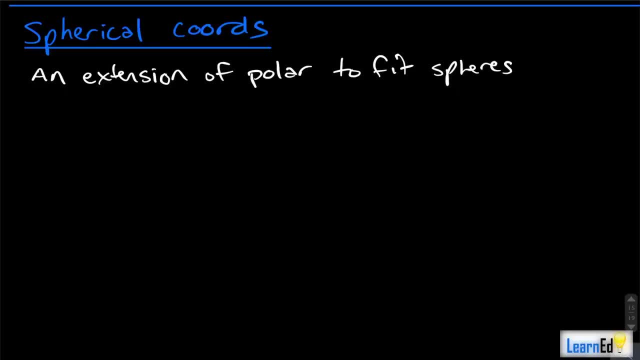 Okay, Moving on to spherical coordinates: Okay, Uh, the big thing to know about spherical, okay, the the, the heart. another rough part about spherical is that you're going to have to know what the actual conversions are. Okay, 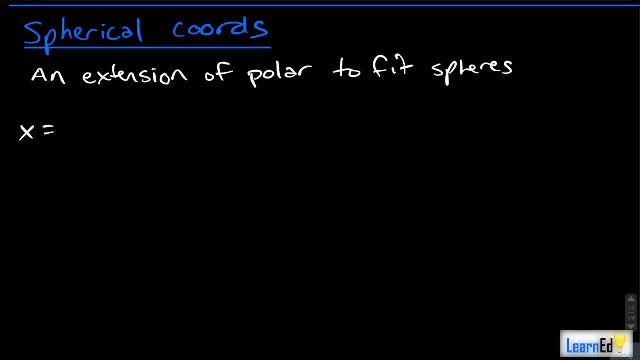 That's something you already probably thought of when I mentioned spherical. So I'm going to start off with um Polar and I'm gonna show you how, with polar, it's pretty easy to get spherical. Okay, And I'm not going to drive the whole thing. 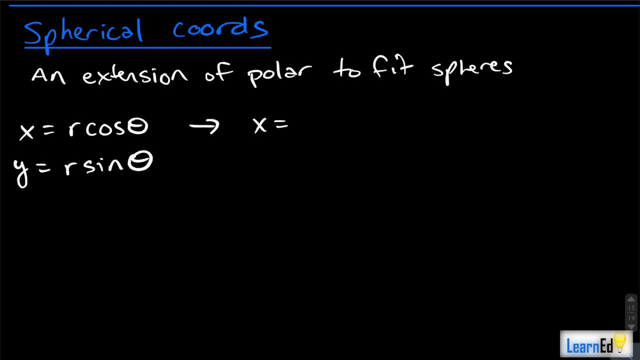 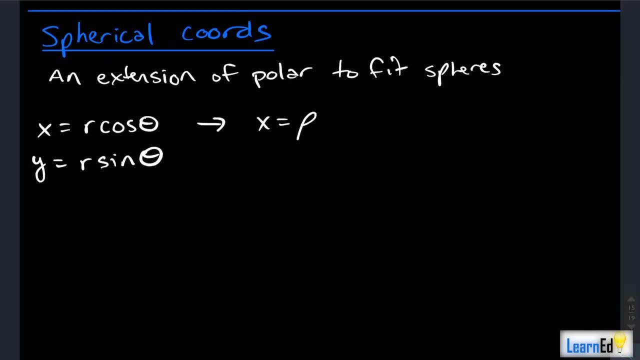 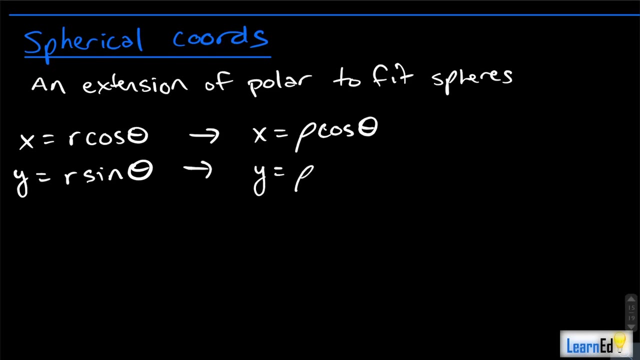 Okay, I'm just going to kind of do a cheaty way to remember this. Let's just convert all the Rs to rows, Okay, The, the P thing, And so I'll put in cosine theta, Okay. And then I'll say: for Y, this is row sine theta. 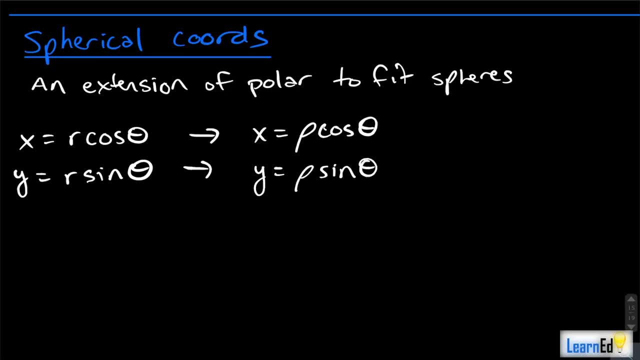 Now you may be thinking: well, this is not complete. This is not what X and Y are in spherical. You're right, Cause all we have to do is add a sign of Phi to both of these. Okay, So you just got to remember. for X and Y, you add sine Phi. 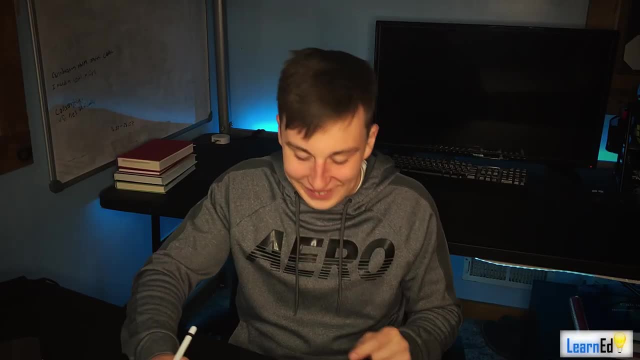 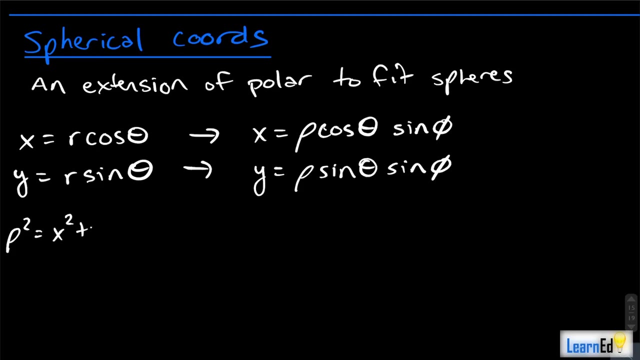 Ooh, that rhymed. Yeah, Remember it that way. All right, So for Z, how you can figure this out? if you catastrophically did not remember this, you can derive it using a row: squared equals X squared plus Y. squared equals Z squared. 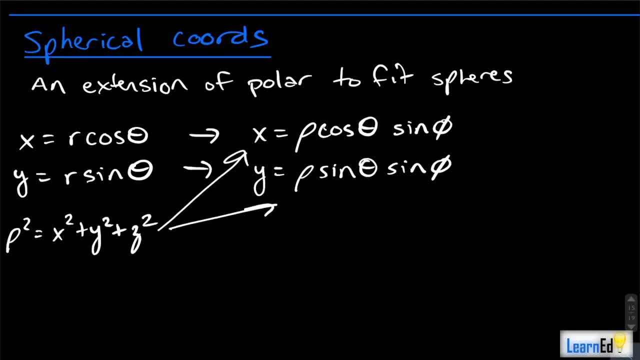 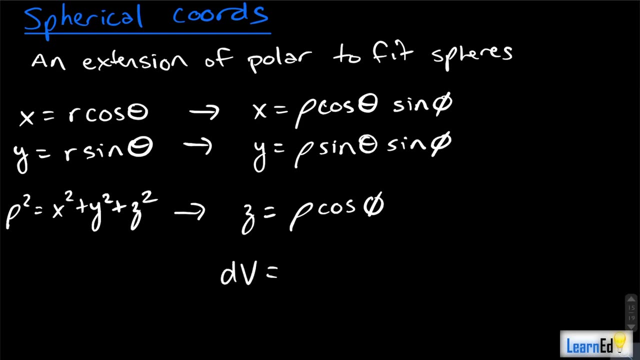 You substitute these guys As in to this equation and you'll get the equation for Z, which is that Z equals row cosine Phi. Okay, And then for DV- I would just try to remember this- Okay, Or you could use a Jacobian, and no, you don't want to do that. 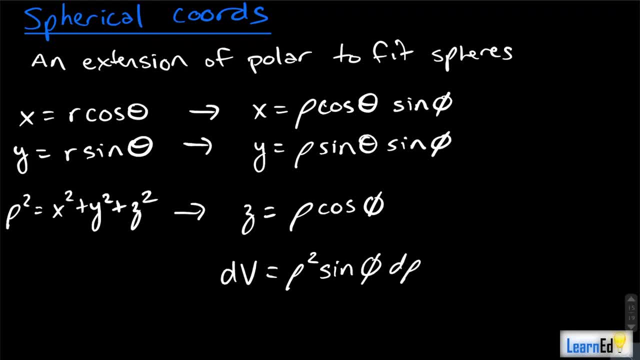 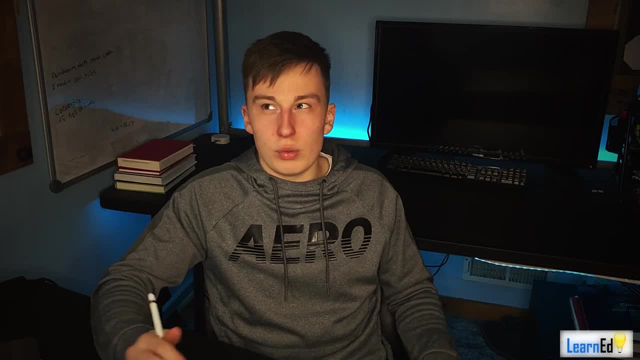 So, row squared, you'll get a sign: Phi D, row D, theta D Phi. Okay, So you're going to have to use that, But so so, really, the only thing that you have to remember is the, the, the DV, the differential. 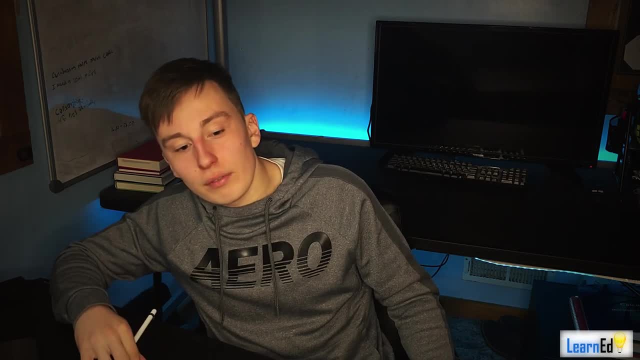 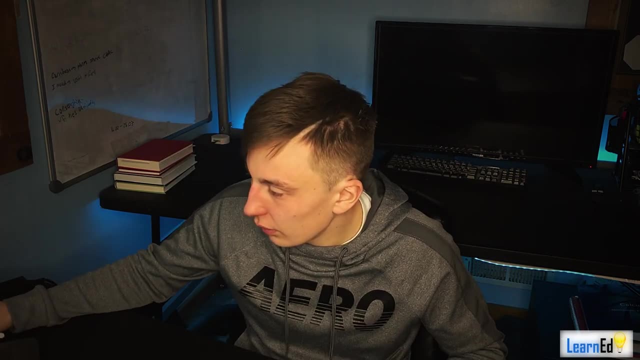 of the volume. Okay, Hey, I'm trying to record a video. Stop, No, my dog's whining at me. I'm trying to do video. I will feed you later, or well? a treat, No, a treat, I don't know. 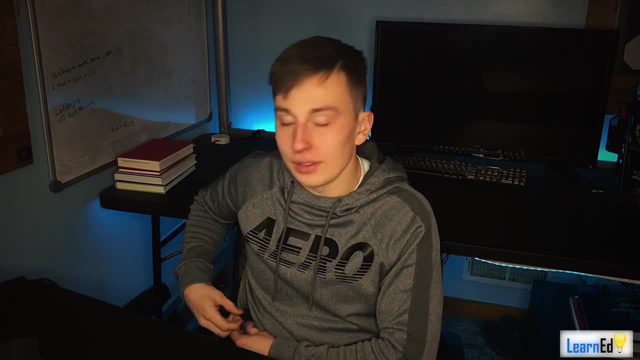 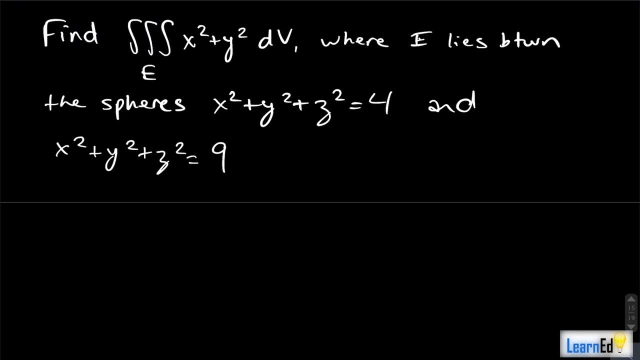 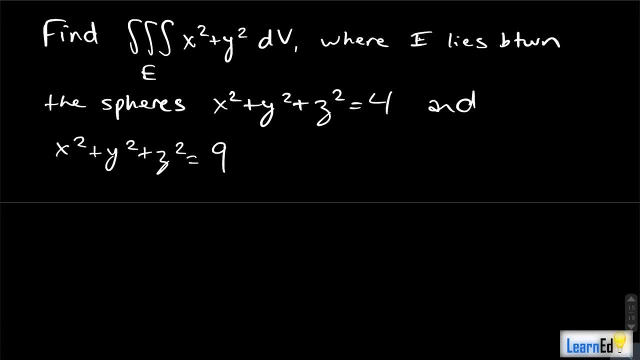 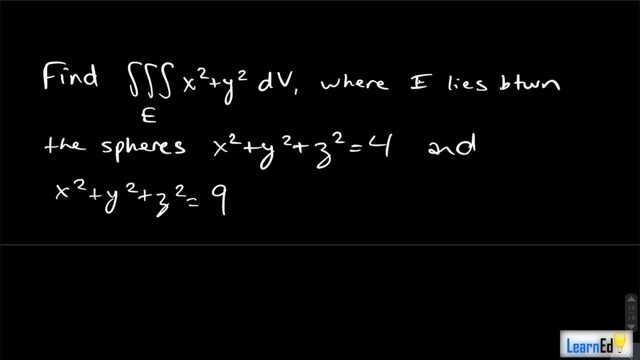 Y squared DV, where E lies between the spheres, X squared plus Y squared plus Z squared equals four, and X squared plus Y squared plus Z squared equals nine. It's almost impossible to not think spherical when you, when you look at something like this. 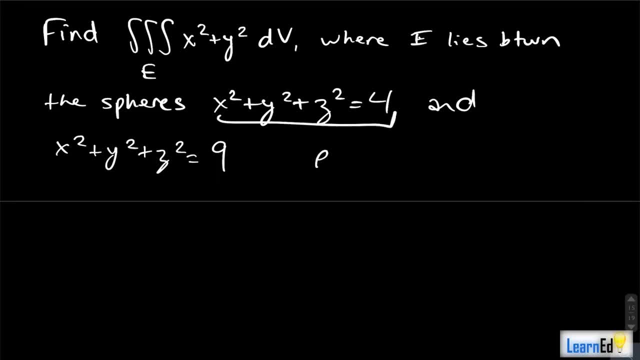 Okay, Cause here this is just row equals two, Essentially Okay, And this is just row equals three. So you just have your row between two and three as your bounds. So there's that one done for theta. Well, these are spheres centered about the origin. 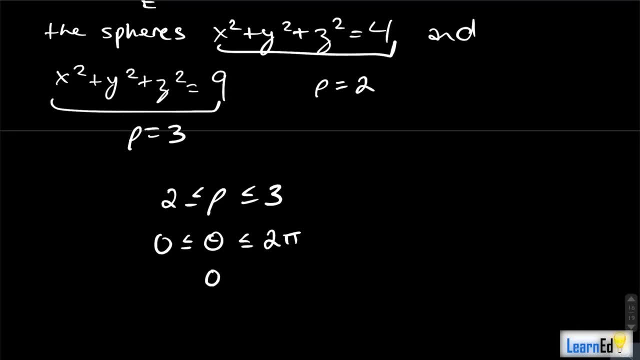 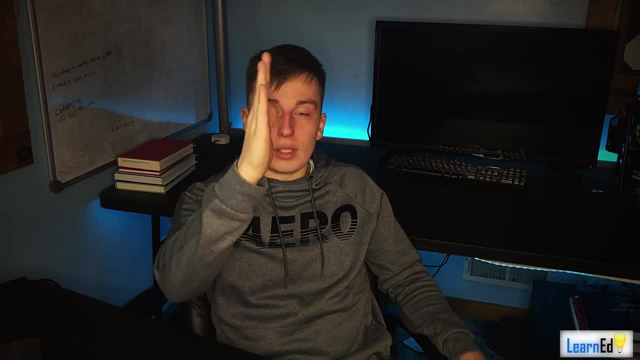 So it's zero to two PI. and for five? well, remember what five is. by the way, it's the angle made with the positive Z axis. The maximum value that can make is from zero to PI. Don't make the mistake of making that from zero to two PI. 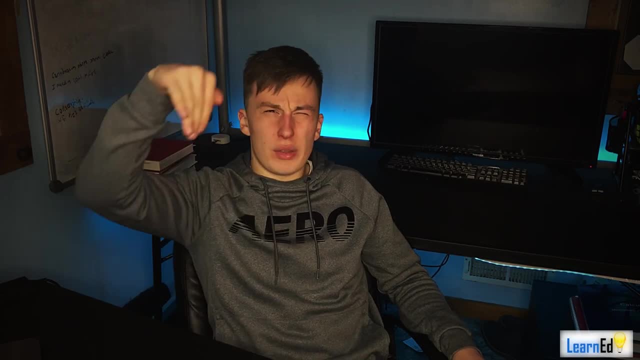 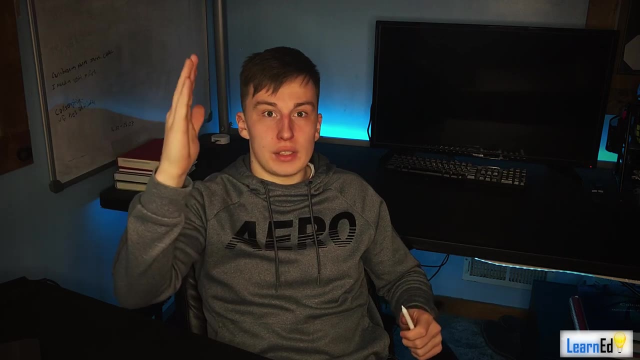 That's redundant. Okay, That'll be redundant. That'll kind of integrate the whole thing twice. I think it's not going to work right. So yeah, from zero to PI, because that's the maximum angle that you can make with the positive. 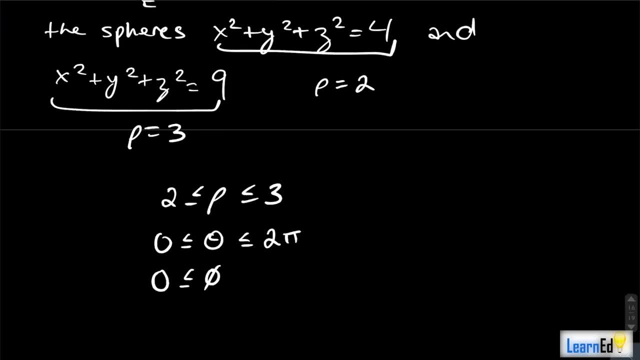 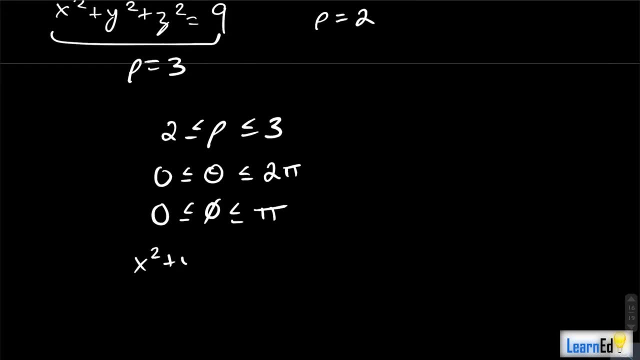 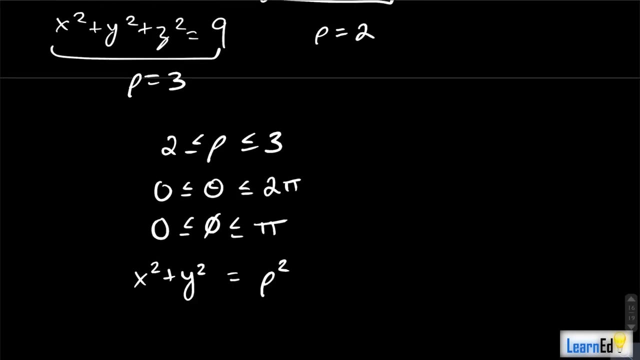 Z axis. Okay, So zero to PI. Okay, Now we just got to set this integral up, and also, in doing so, we'll have to figure out our integrand X squared plus Y squared, What does that become? Well, I'm just going to write that as: row squared, cosine squared, theta sine squared. 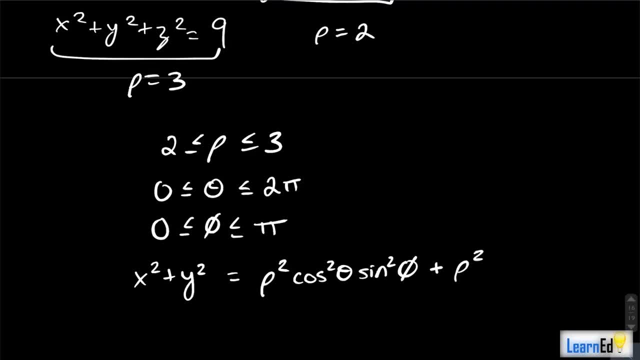 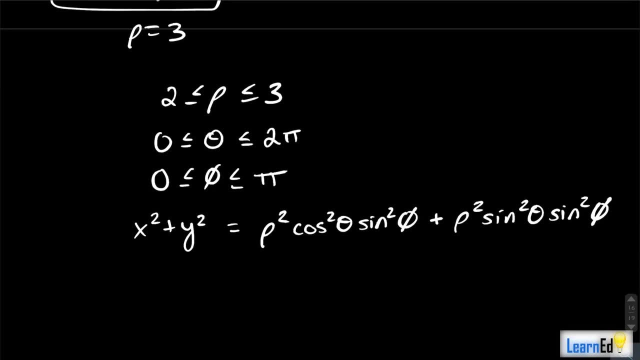 five plus row squared sine squared theta, sine squared five. You can probably guess what we're going to do. We're going to pull out everything but the cosine squared theta and the sine squared theta and get row squared times a sine squared theta or, sorry, sine squared five. 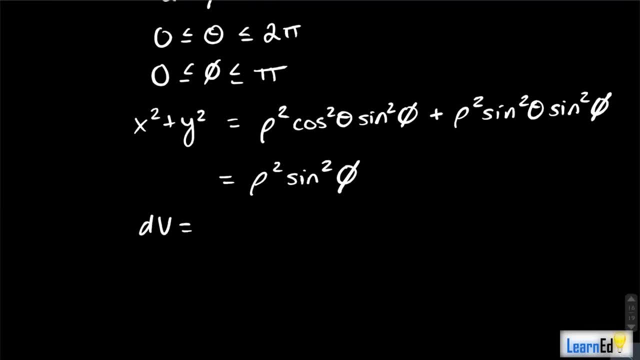 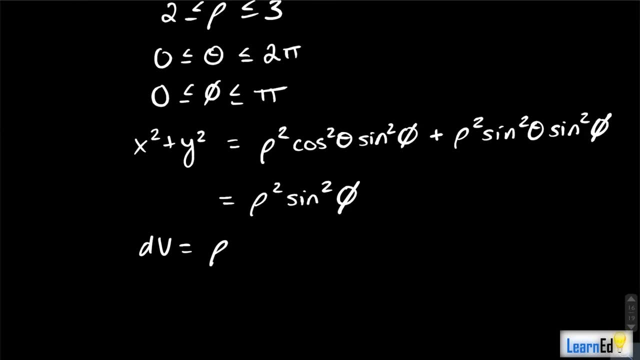 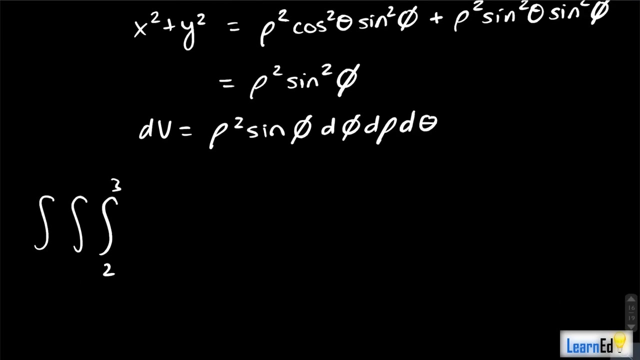 Okay, And remember DV. It is equal to row. was DV equal to row squared? I don't have to remember it. You do row squared sine five D, five D, row D. theta was the other one for setting up this triple integral. We have row going from two to three. 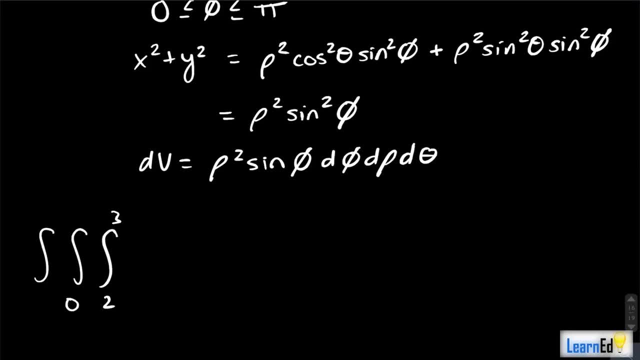 Okay, And our, uh, we're going to have theta going from zero to two PI and we have five going from zero to PI. Okay, And we, uh, we'll have our integrand being row squared, So so that's going to combine with our DV. 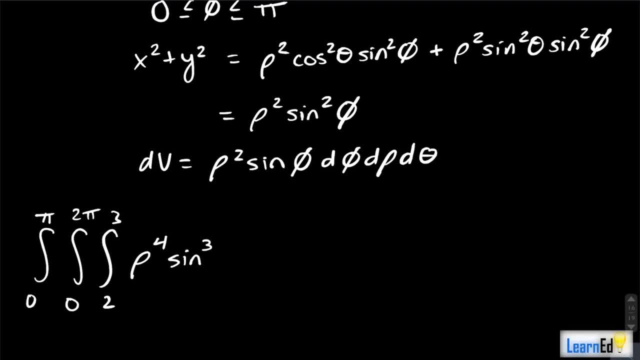 So we get row to the fourth and we get a sine cubed five and we'll have a D row D theta D five. Okay, And make sure you do those, those differentials, uh, in order, because if you don't, then you're. 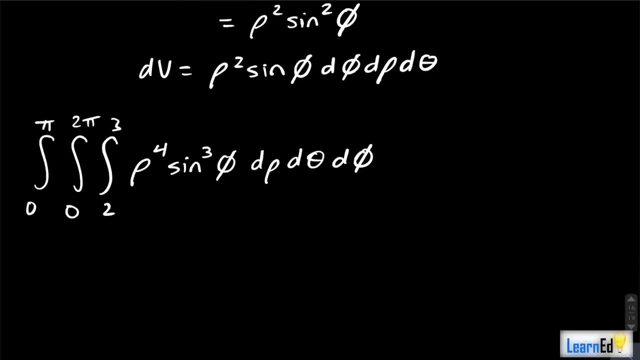 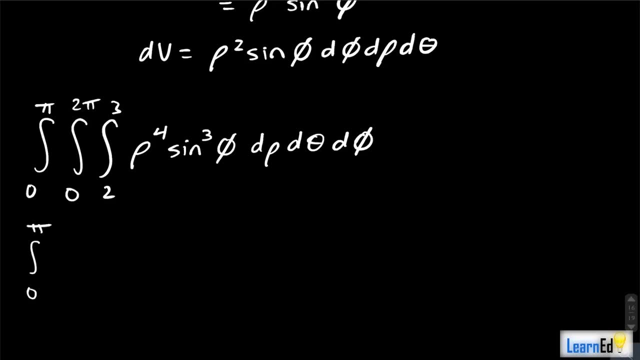 going to get points off. That's going to be annoying for you, Okay, So what we can do, since these are not dependent on each other, is we can just break these integrals up So we have integral from zero to PI of a sine cubed D five times the integral from zero. 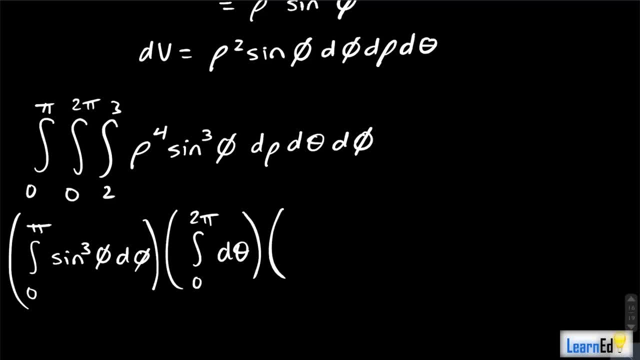 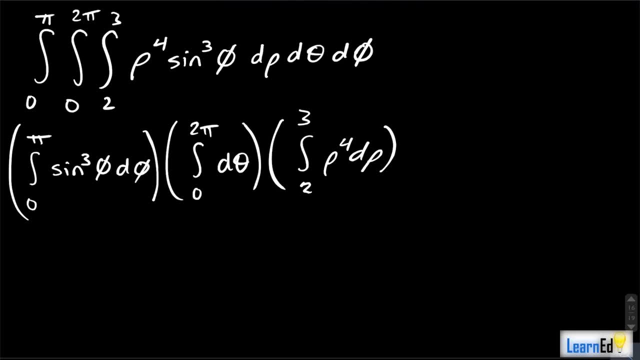 to two. PI of D theta times the integral from two to three. I've wrote the fourth D row Okay And uh, so. so the hardest integral is going to be, of course, the one all the way over to the left, the five integral. 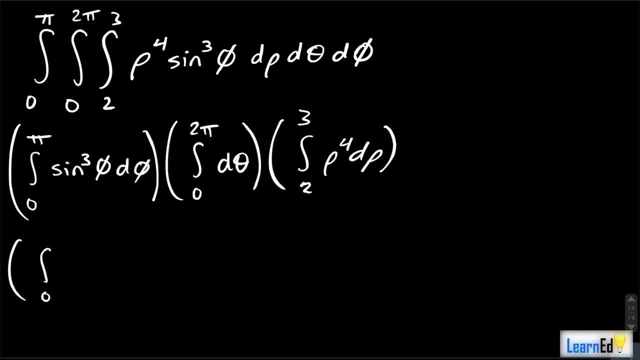 So all we have to do for that, if you remember from Calc two, is we would just. since this is an odd power of sign, we can just represent this as sine five times one minus cosine squared five. Okay, Which use trick identity? 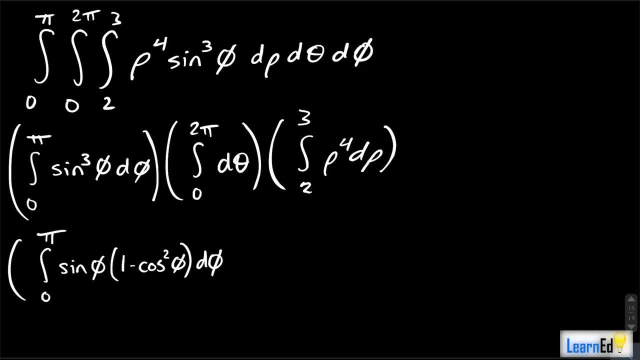 Uh, so, like you know, we break it up into sine five, sine squared five, and sine squared five is one minus cosine squared five. Okay, So now we have a theta evaluated from zero to two PI, and we have a row to the fifth over. 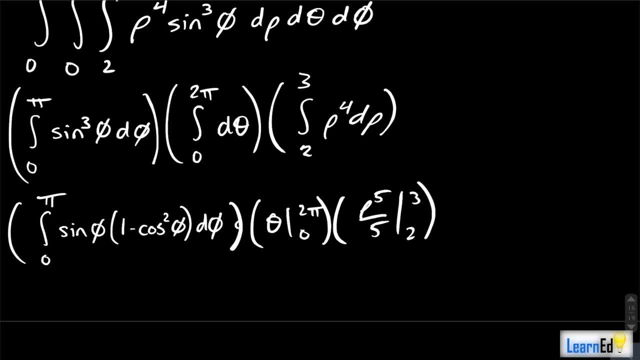 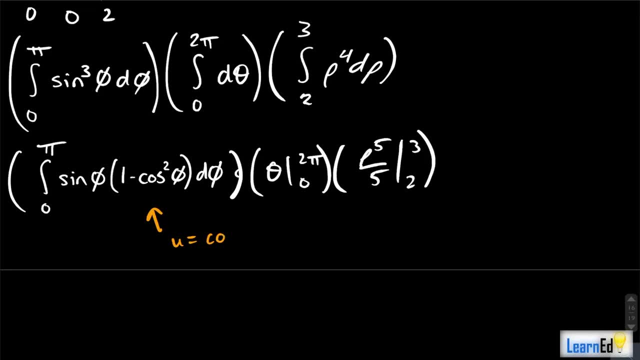 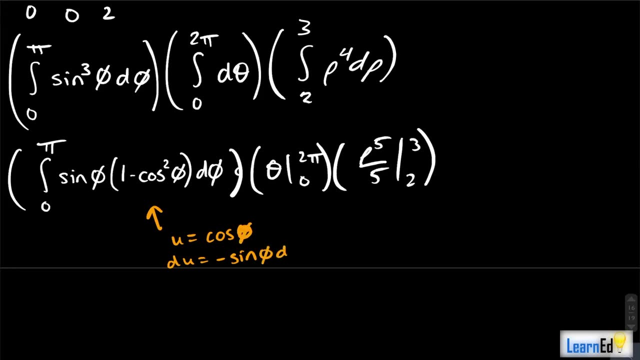 five, evaluated from two to three. Okay, This integral here is going to be you substitution. You equals a cosine. theta D equals a negative sign. Sorry, Cosine five, Oh, Okay. So the amount of times that I made a mistake like that in Calc three, you would not believe. 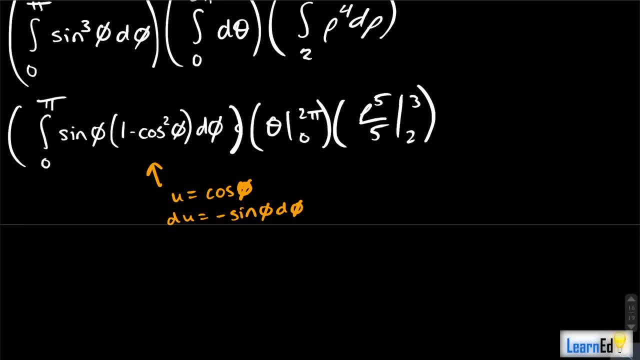 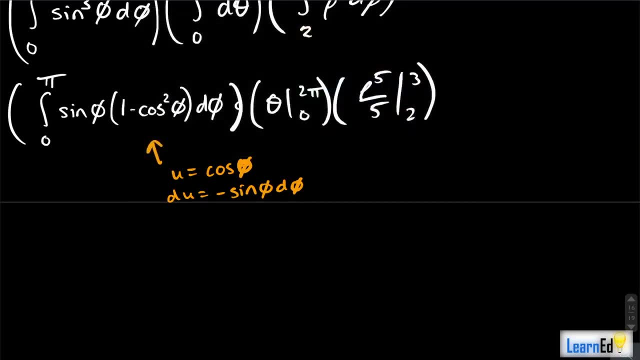 it honestly. So hope you. hopefully you can relate there, if not, and that's fine, I guess. whatever, I guess I'll be fine, It's no big deal, I guess. So also, uh, when I'll do our bounds here, when you uh sorry, when five equals zero, 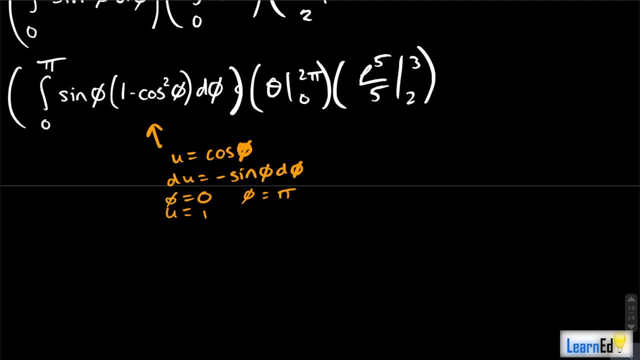 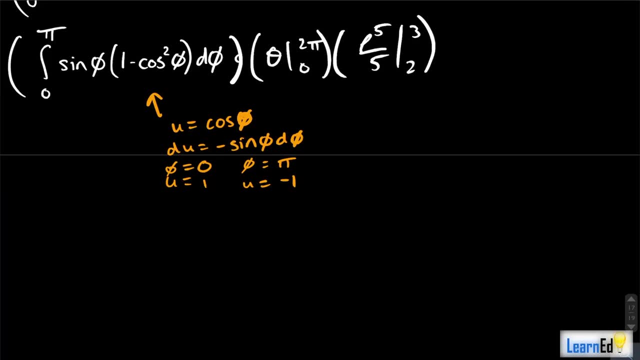 you equals one. When five equals PI, uh, you equals negative one. Okay, So what I'm going to do here is I'll do two steps here, just so you guys can see exactly what I'm doing. but we end up with an integral from one to negative one, and it's a negative. 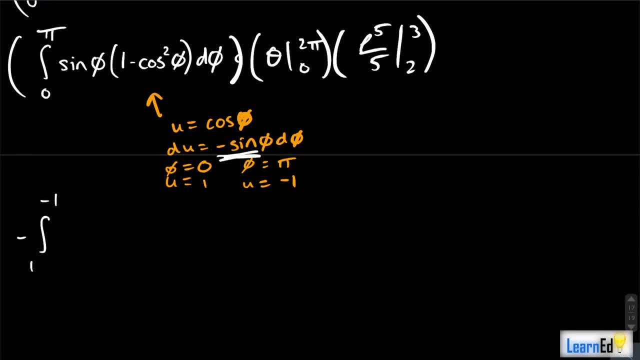 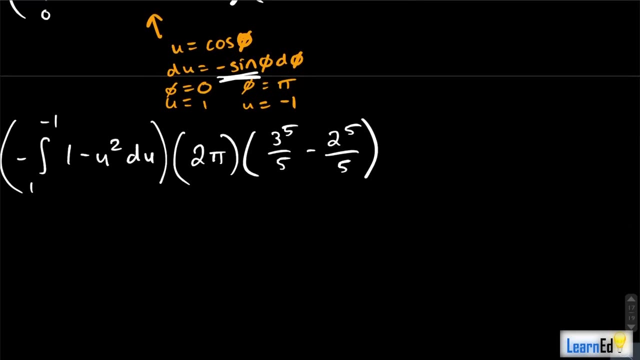 integral, because this negative sign five. So what we get is a one minus U squared DU. So what I'm going to do here, as you can probably expect, and I'll just substitute in these other guys here- is I'll switch the bounds. 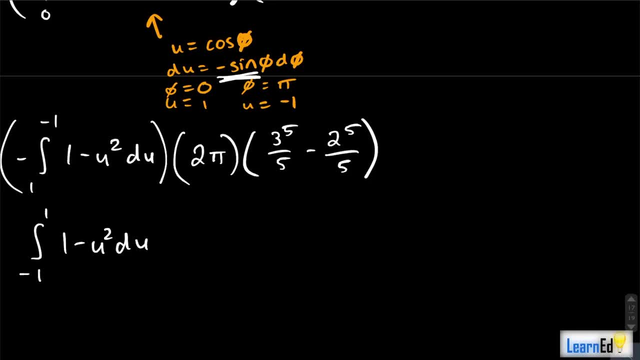 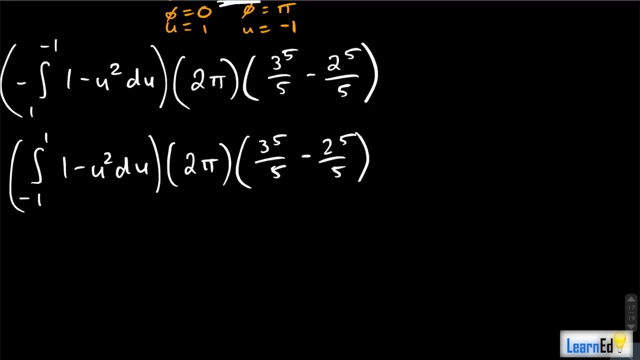 So we have negative one to one of a positive integral. Uh, we have negative. sorry, we have one minus U squared DU, and that'll be nice or to deal with. So actually, this is even so. uh, what we can even go further and do is just integrate from. 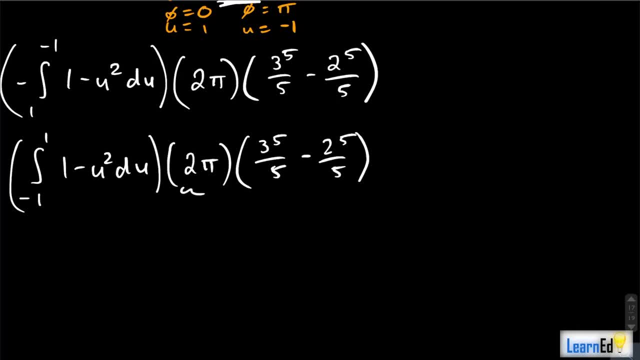 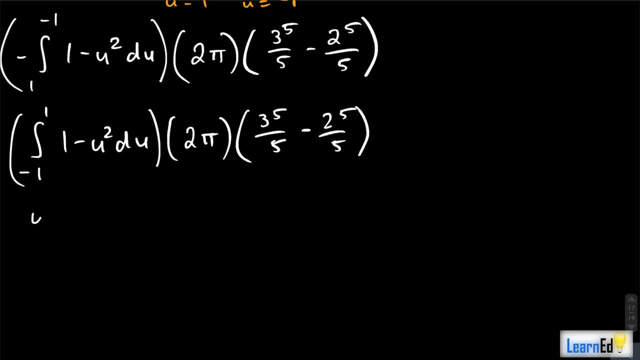 zero to one and make this a four PI or something like. I don't know, we can make this thing a four PI, Um, just like taking out a two, So what else? Okay, So what I'll do is I'll integrate. 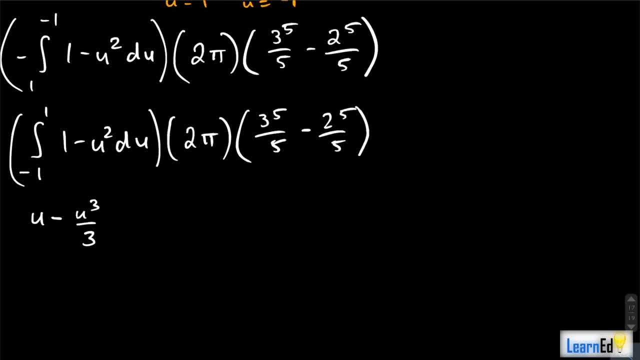 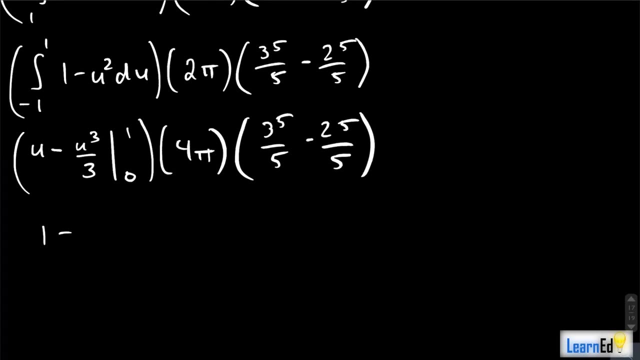 So we've you minus U cubed over three, and that'll be evaluated from zero to one. We'll multiply that times four, PI. multiply that times three to the fifth over five, minus two to the fifth over five, And this'll just be one minus one third, which is two thirds. 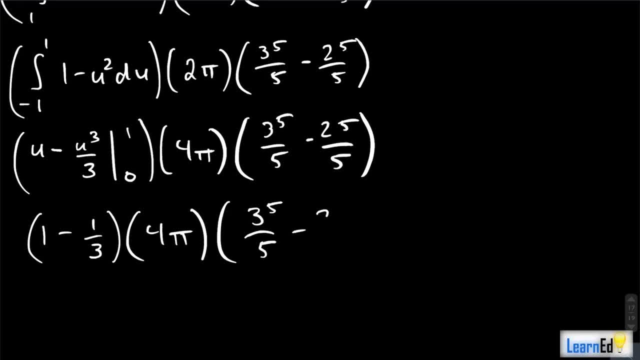 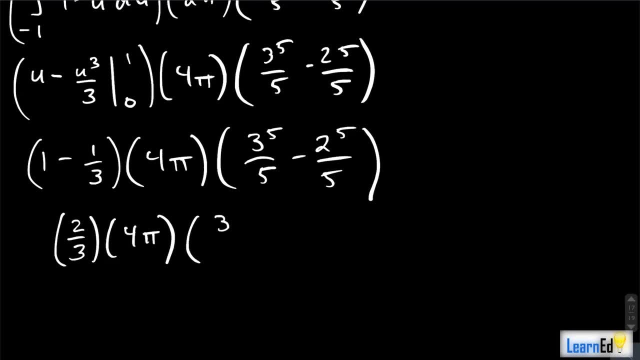 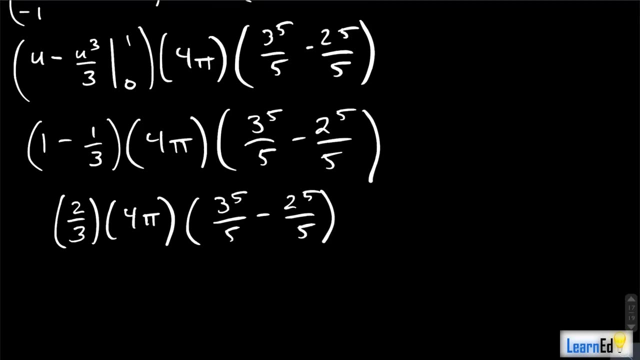 Uh, and I'll simplify down one more time before giving you just the answer: Uh, this is two thirds. This is two thirds times four. PI comes whatever. three to the fifth is over five, minus two to the fifth over five. What you will uh end up getting is hundred 1,688 PI over 15.. 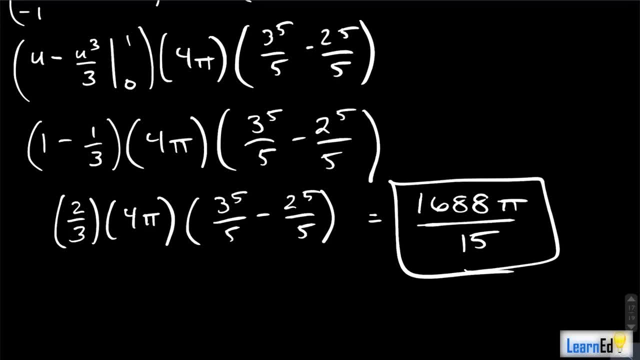 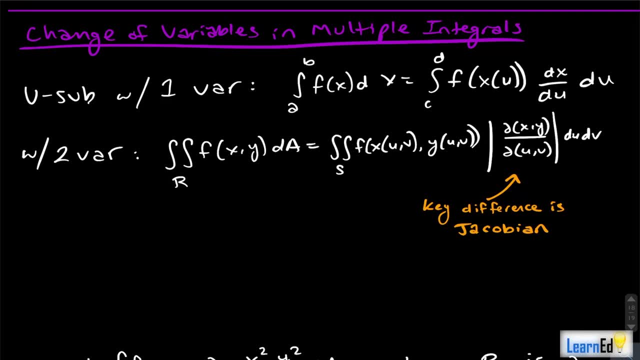 So that is ginormous. uh, yeah, have fun with that. So we're going to move on to the last question here, the last kind of section that we're going to cover. Okay, It's the change of variables. uh, with multiple integrals. 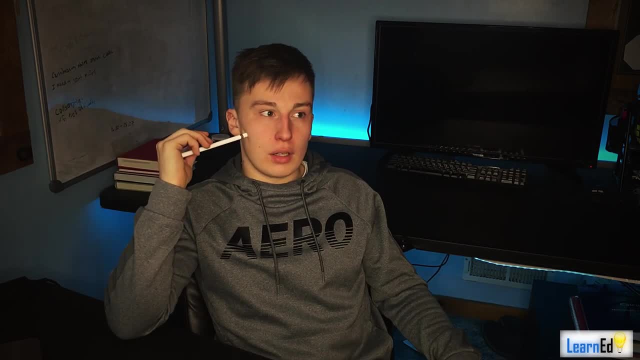 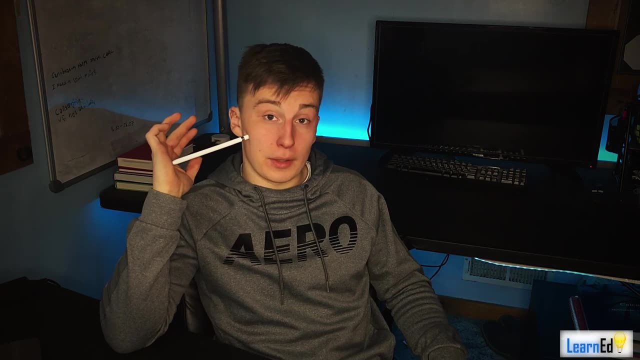 Okay, So this is probably everybody's least favorite thing, uh, other than just straight out: triple integrals, not cylindrical, not spherical. probably everybody's least favorite thing about multiple integrals, including me. Uh, although triple integrals is a pretty, I mean, triple integrals is now my least favorite. 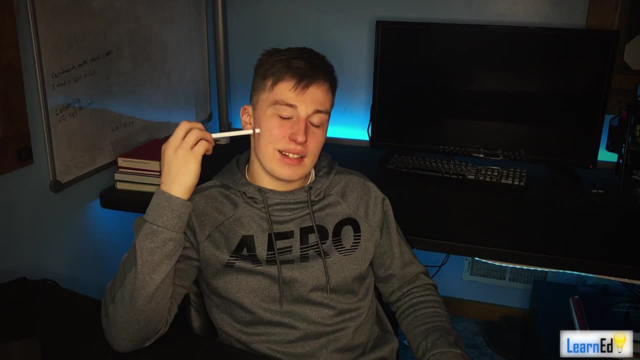 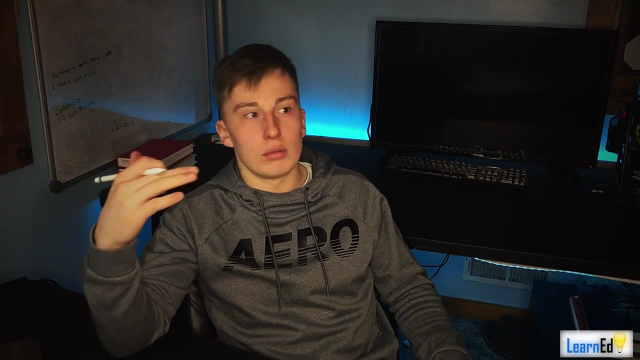 because I realized that change of variables isn't that bad Um. but also, I guess the example I'm going to give you here is not going to be the worst thing in the world. It's going to be, you know, I don't know. it's going to be a decent example. 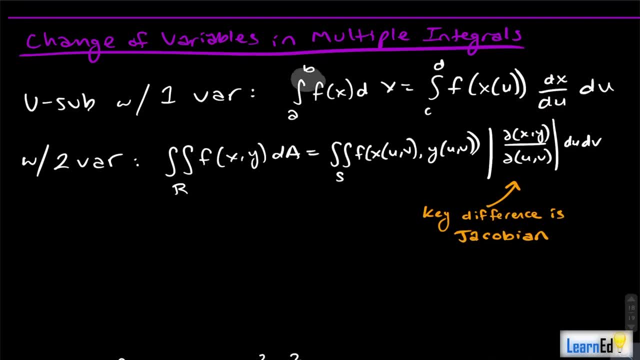 We'll see when you do a use substitution with one variable. this is essentially what you're doing here. You have the integral from a to B of F, of X, DX, and that's equal to the integral from C to D of. so you know you change your bounds in the with respect to you you represent. 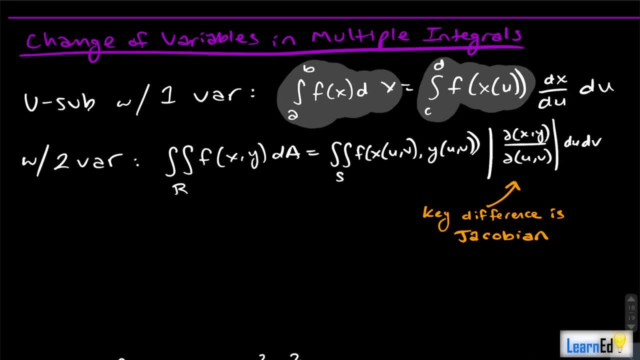 your function of X as a, as a function of you, you multiply by DX, DU kind of. the logic behind this is that you're multiplying by DU over DU, So it's still equal to DX, So it's essentially like you're multiplying by one. 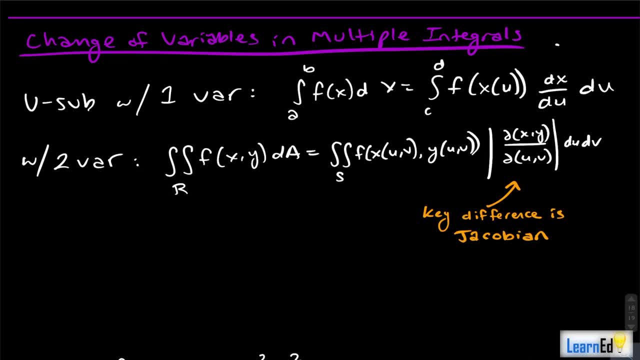 Okay, So that's what we're doing when we- uh, you know, we said DU equal to two DX or something like that, And then we substitute in for DX. This is essentially what you're doing here, Okay, But when you have multiple derivatives to deal with, when you have partial derivatives, 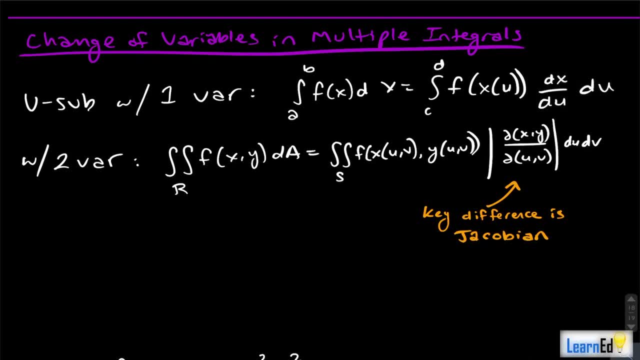 what you need to do is put that into a matrix. Okay, That's how you have to compute, whatever this thing is. Okay, So with two variables. Yeah, You know, you can see that we have our, our, our function of X and Y and we change this. 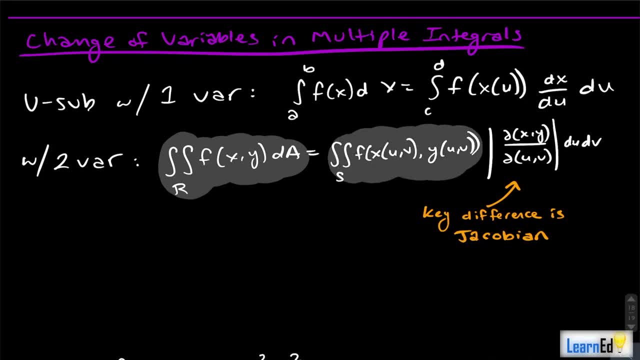 to a function of X and Y, but now X and Y are represented as functions of you and V. Okay, So you know. now we have something completely in terms of you and V. we multiply by our Jacobian, which are Jacobian in one variable is that DX over DU. 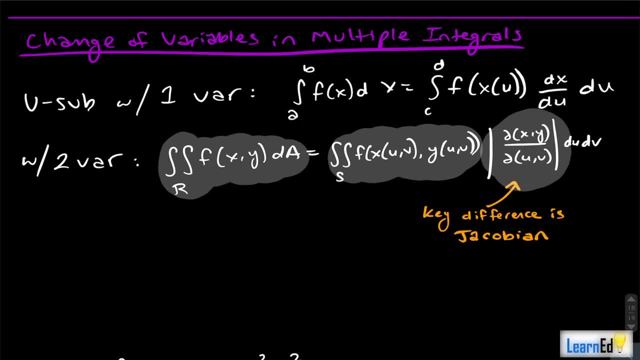 Okay. But now it's a matrix. Okay, Because we have multiple derivatives. So we have- you know, we have to do- a lot of correcting factors, Okay. And then we have our DU and DV on the outside. Okay. Now our Jacobian. I'll talk about that in a little bit. 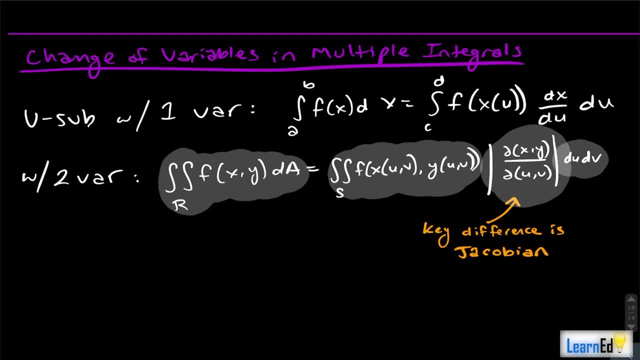 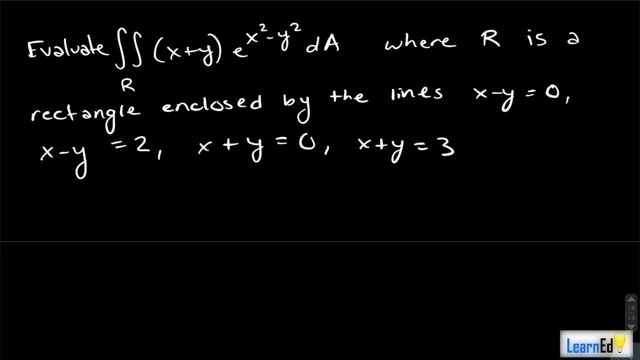 There's some nice things that you can do with a Jacobian that makes it look or that makes your life a lot easier. So we want to evaluate the double integral over the region R of X plus Y times E to the X squared minus Y squared DA, where R is a rectangle enclosed by the lines X minus Y. 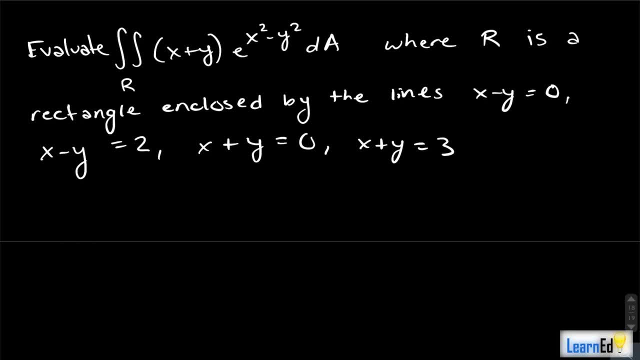 equals zero, X minus Y equals two, X plus Y equals zero. Okay, And then we have our X plus Y equals zero and X plus Y equals three. Now you, you know, you can look at the integrand to see what you can do to simplify this. 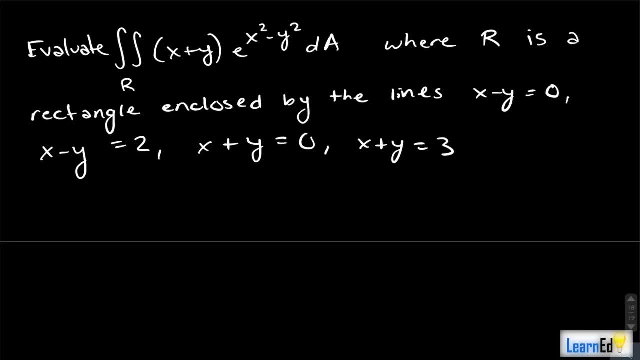 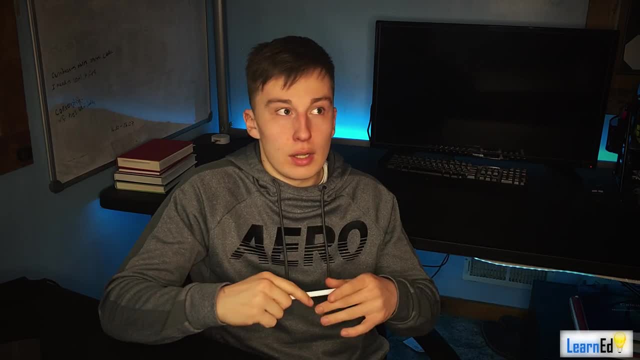 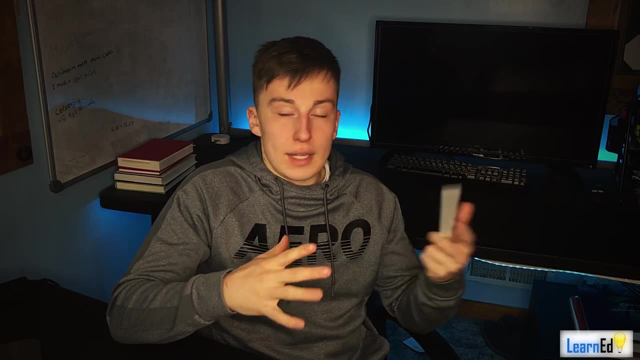 And that's fine. I mean, you can look at either the integrand or the bounds of how you want to simplify this, because that's, you know, that's what our, our use, our UV substitution is doing. Right, It is simplifying this, whether it's simplifying the bounds or it's simplifying the integrand. 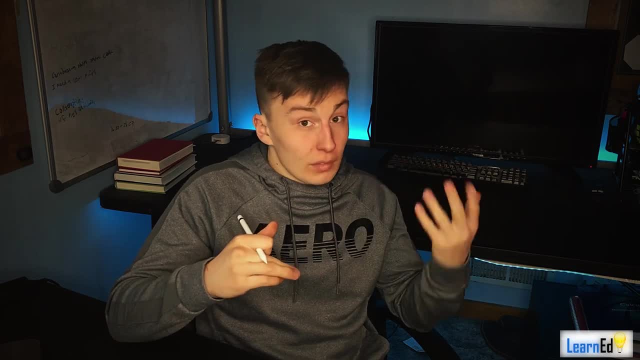 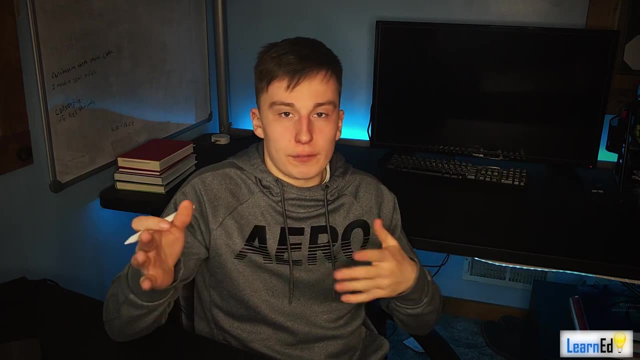 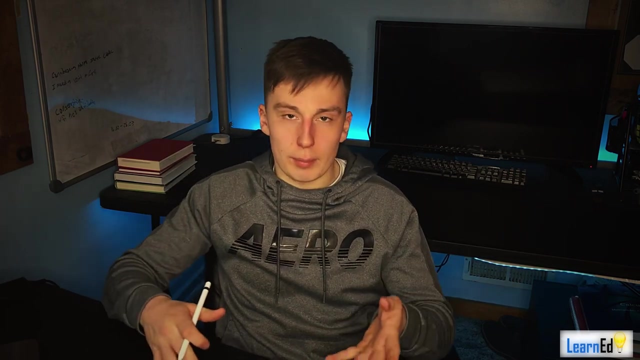 in general, Like with cylindrical And spherical, those are essentially UV substitutions. well, UVW substitution because, because those are for triple integrals, we're dealing with double integral. So this is essentially like polar cause. you know that'll be more relatable of the case. 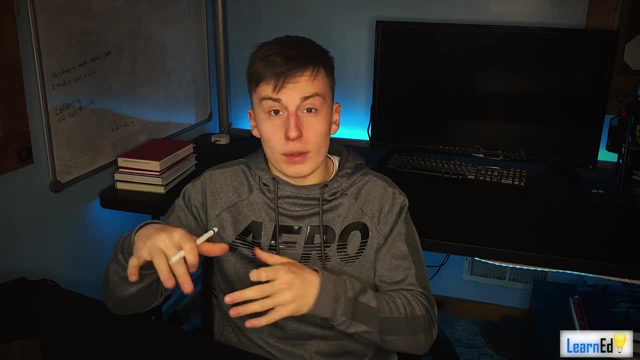 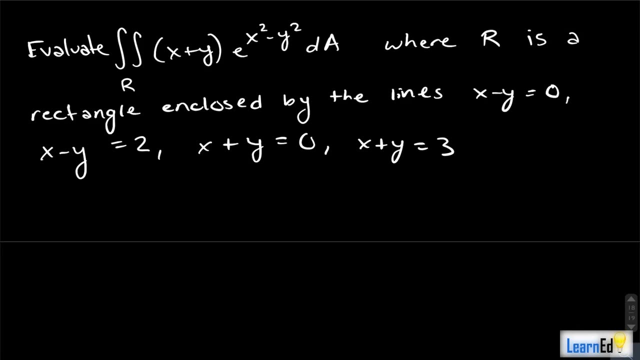 we're doing right now? Okay, We're switching to other coordinates to either make our bounds nicer or our integrand nicer, Okay, So now you know we can look at either our integrand or our bounds to try to figure out what we want to do here. 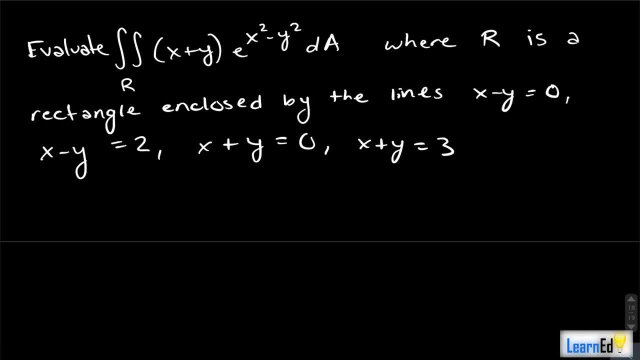 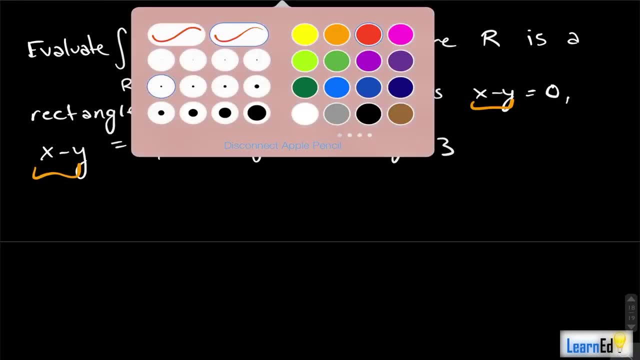 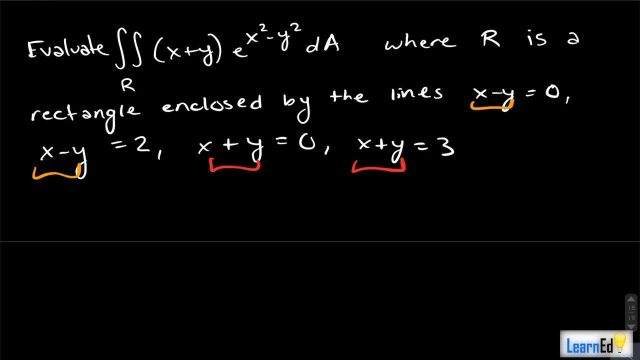 Now, what you'll notice here is that, first off, if you look at your bounds- X minus Y, X minus Y, X plus Y, X plus Y- okay, That should kind of throw something right out to you already. but you know, you see. 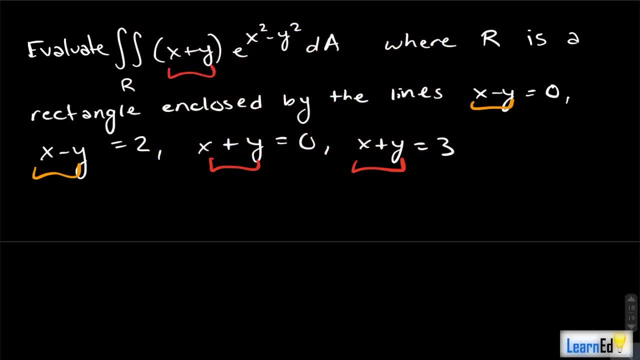 the X plus Y show up again in the integrand. but then you have this different thing to deal with right here, which is an X squared minus Y squared. Okay Well, So remember right, If you multiply X plus Y and X minus Y together, you'll get X squared minus Y squared. 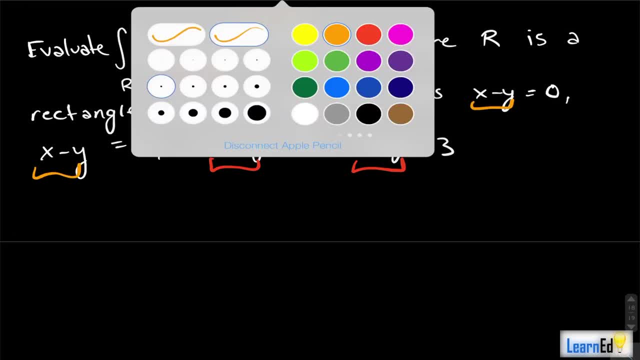 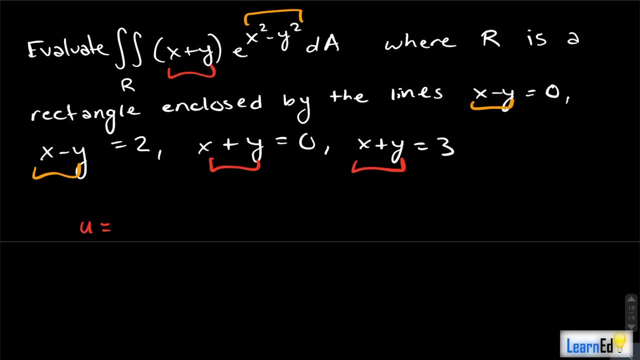 Okay, So you've kind of have hopefully figured out your substitution. you, we can say, is equal to X plus Y. Okay, And I believe that's what I did in my notes too. Yes, Okay, I did say X plus Y, not X minus Y. 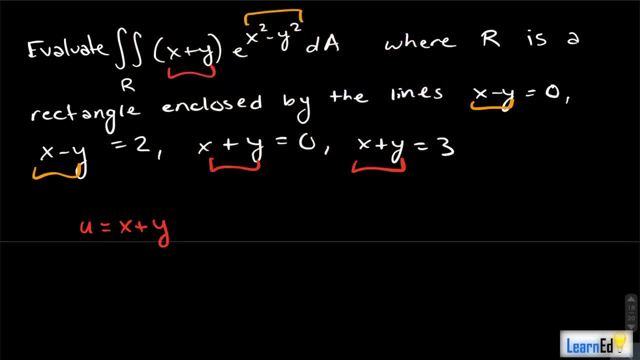 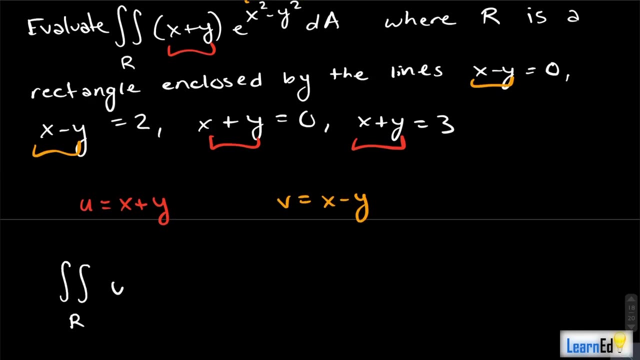 It doesn't matter, I just want to stay consistent with what I did. Okay, So here's what I did. And V is going to equal X minus Y. Okay, Watch how nice this becomes. Now we're going to have the integral over some region, R of U, E to the remember this. 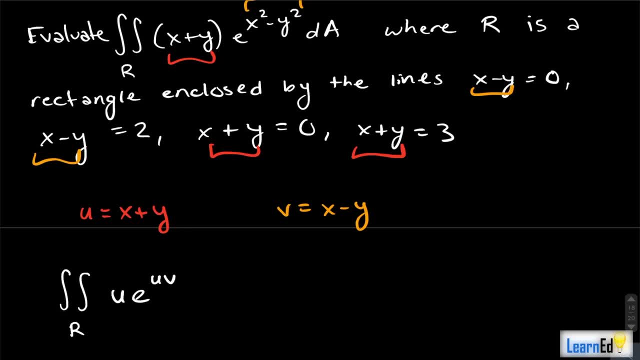 will now become a UV in the exponent. Okay, You can check me on that if you'd like. We're going to have this all times. a Jacobian Okay? So we'll call that J Okay, And we're going to have D U D V. 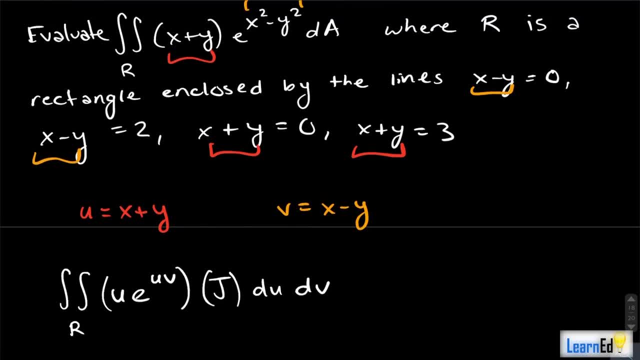 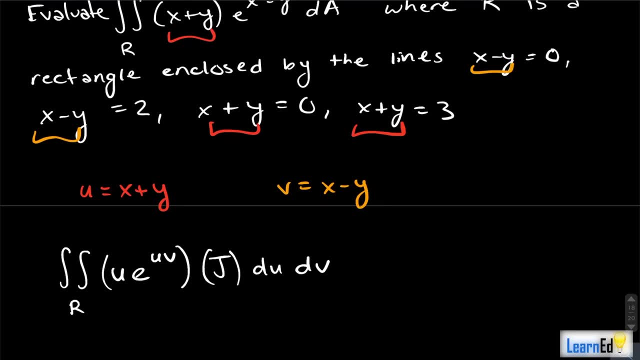 Okay, Now our, our region is a rectangle enclosed by the the lines in this, is you remember? this is going to be in the X- Y plane: X minus Y equals zero. That means that we're going from V equals zero to V equals two, and we're going to be 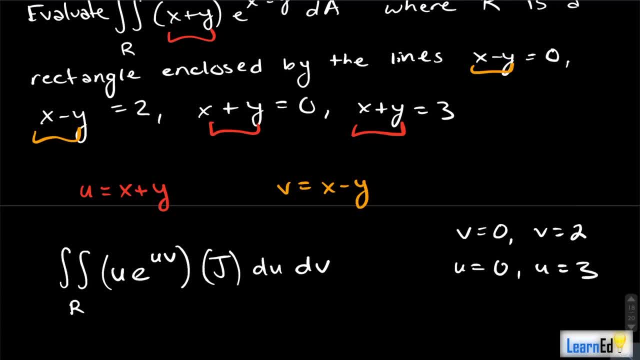 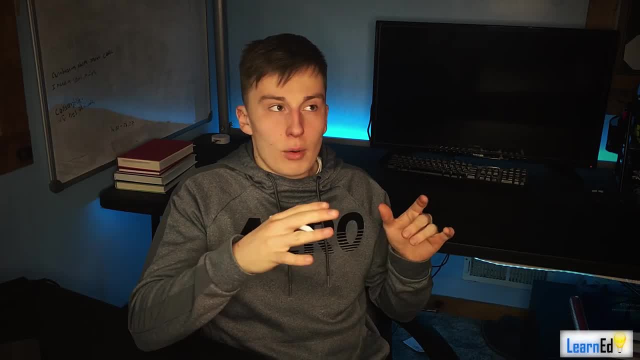 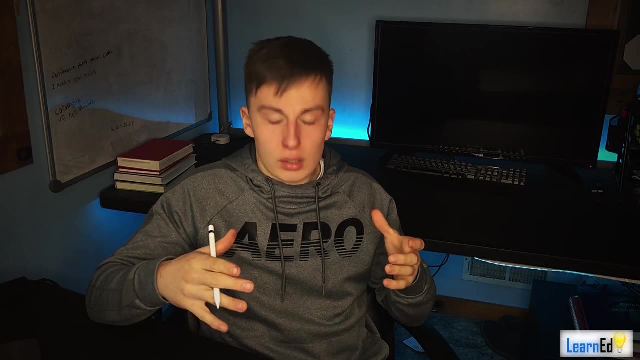 going from U equals zero to U equals three. Okay, So those are our bounds. And so now we didn't only make our integrand nicer, Okay, We also made our bounds nicer, because now we just have a rectangle, right, We have a rectangle that we're kind of extruding upwards, uh, up to a surface that is U E to. 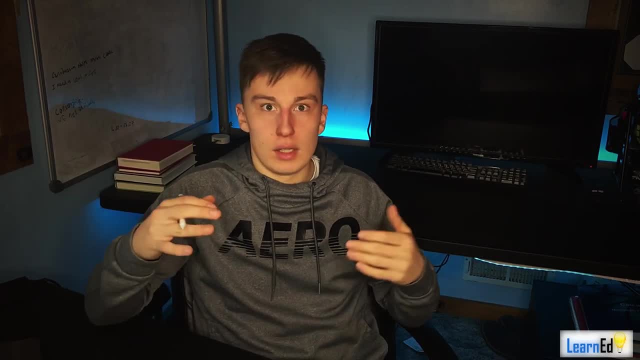 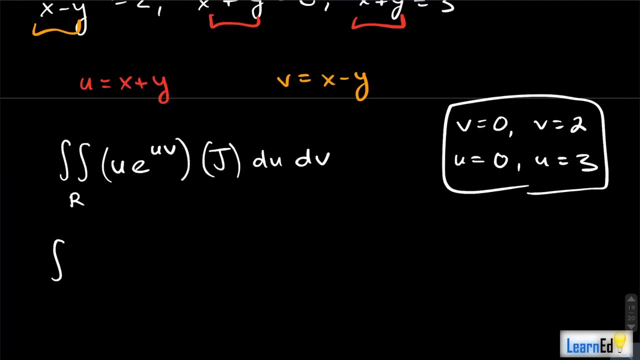 the UV, which is nicer than X plus Y? E to the X squared minus Y squared. Now we can set this up as the the integral from uh. we can do zero to three, zero to two. So we're going to have U? E to the UV and this will be a D V D U. 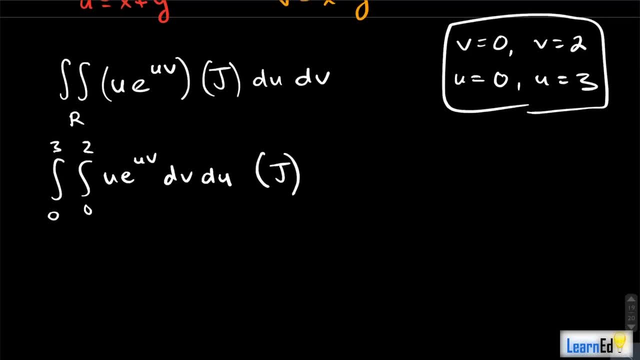 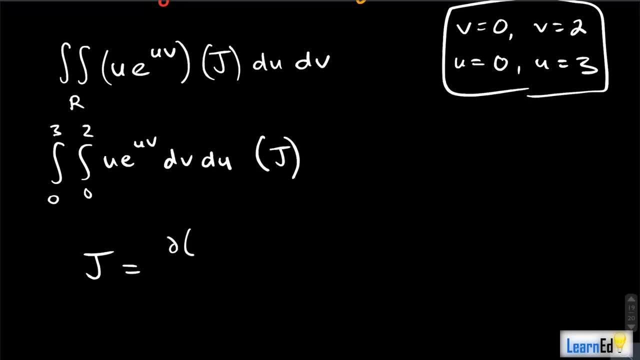 Okay, But remember we also are missing our Jacobian. How do we do our Jacobian Remember? I said our Jacobian was the uh partial derivative of X and Y over the partial derivative of U and V, and that's a matrix. 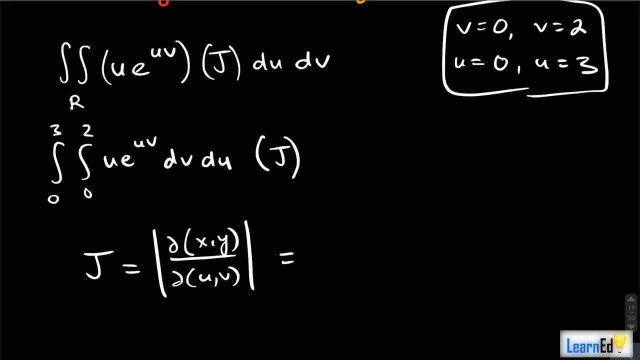 So how do you represent a matrix of that? Well, you're just going to do: Okay, So we're going to do X, D, X, D, U, right, Uh? so we kind of go X, U, X, V, and then the same thing with the wise, okay. 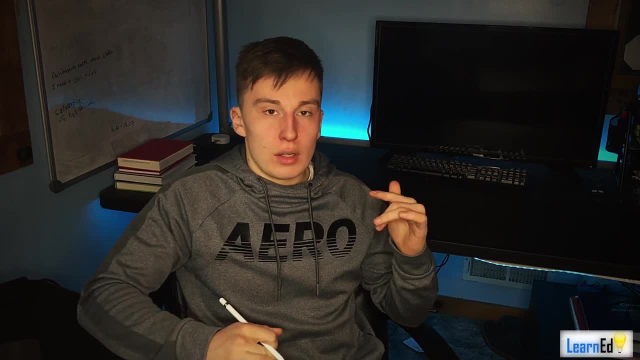 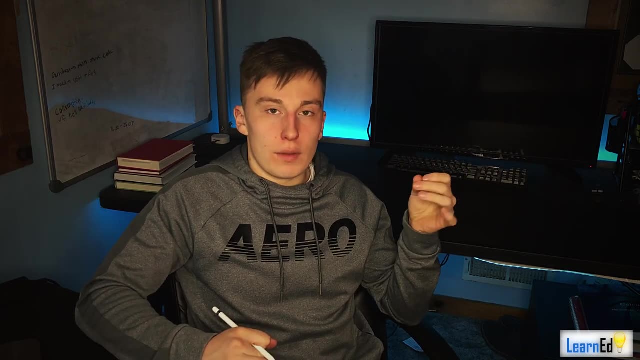 But here's the problem here. The partial derivatives in our Jacobian are not partial derivatives of you with respect to X, or a V with respect to Y or anything like that. They're of X with respect to one of our transformed variables. Well, you are V. 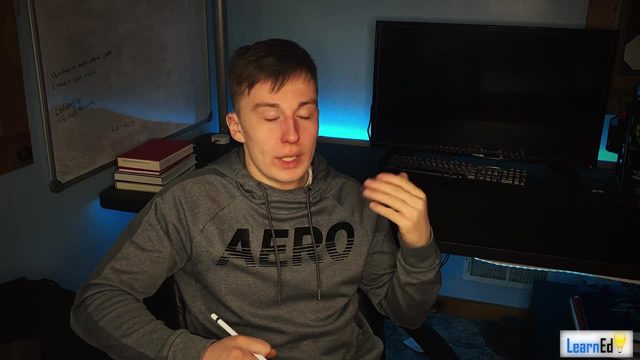 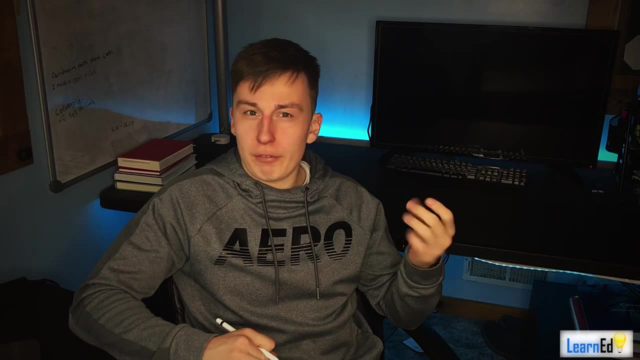 Right, Okay, So you know. we can either solve for what X and V or- sorry, X and Y actually are, or what we can do is modify our Jacobian a little bit to incorporate different partial derivatives. Here's how we're going to do that. 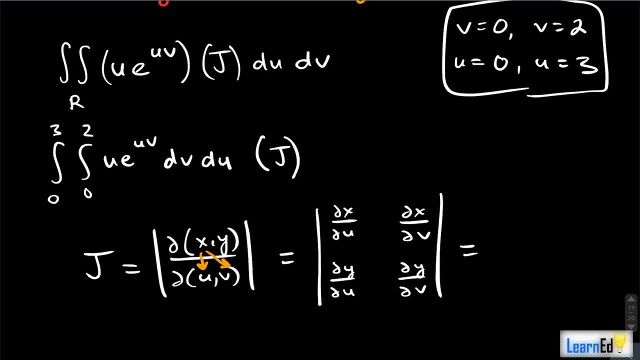 Okay, We can represent this. Let's do you know we can do an operation Like, let's say, we do one over some matrix. Okay, This is this matrix, right here, It's equal to one over some matrix, Okay. 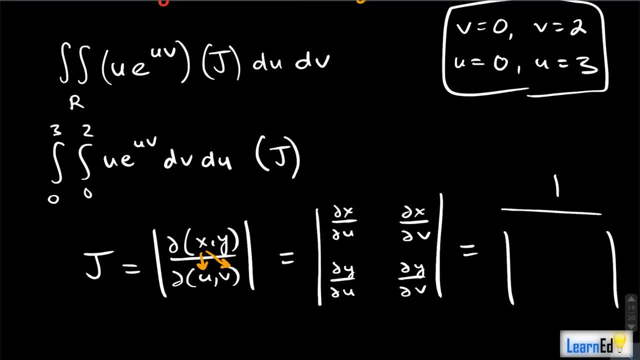 Well, if you're going to do an operation like that, it has to apply to every single term in the matrix. So essentially, what we have to do is we just flip every term in the matrix. Do you DX, DVD, X, D, U, D, Y and D Y, DV right? 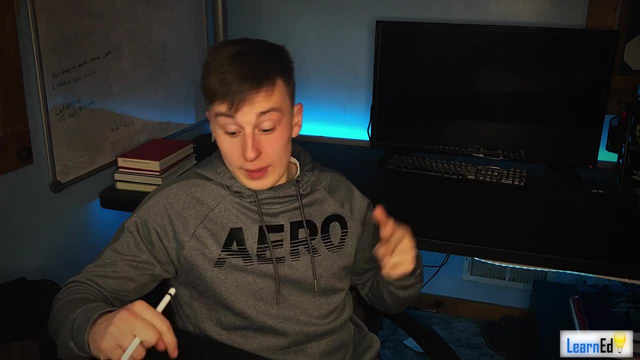 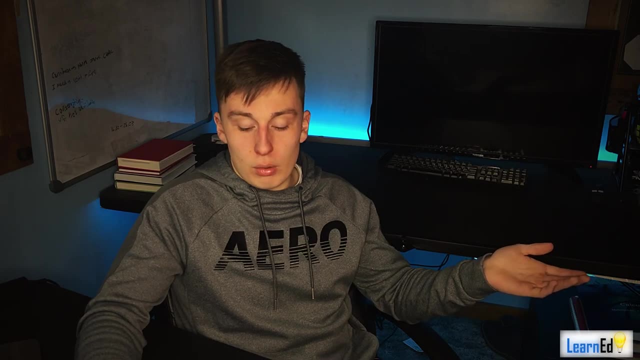 So all we really have to do is compute the Jacobian this way right, The new way that I just showed you. Okay, Let's do one over that And that's going to be our Jacobian. So you know, this is another way to do it. just, you don't have to solve for X and Y. 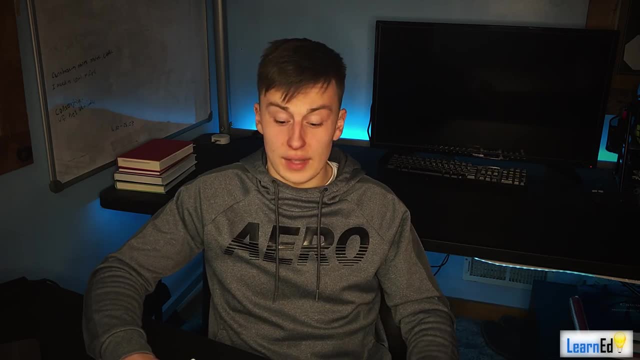 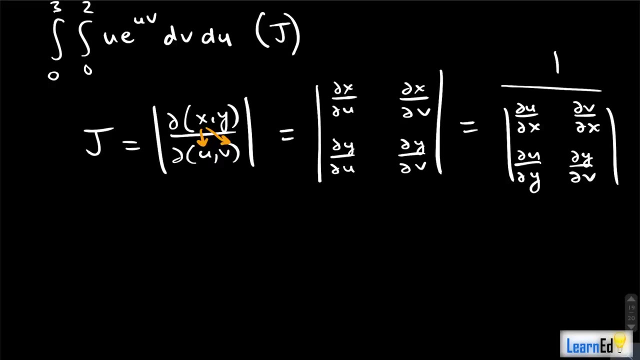 because sometimes it might get a little nasty honestly, like that's what I would do. So cause I don't want to do like systems of linear equations or anything like that. So let's figure out our Jacobian is going to be so actually, let's do one over our Jacobian. 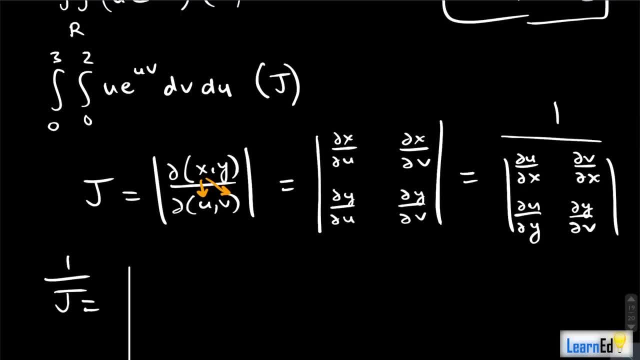 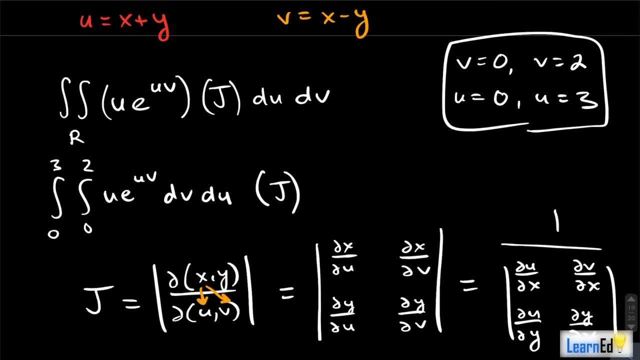 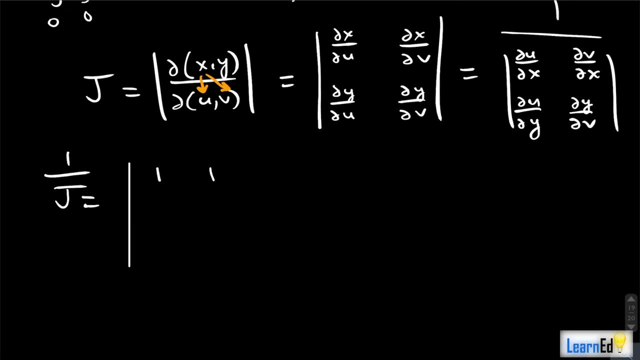 is this, this matrix? Okay, Okay. So we're going to do one over DX, which will be one: DV over DX. That'll just be one as well. The only thing that will be negative is DY over DV. So this will be one and negative one. 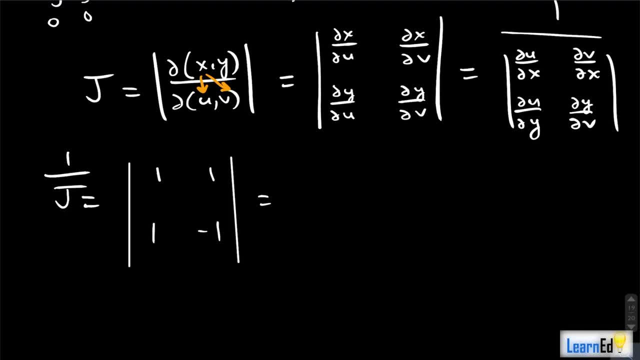 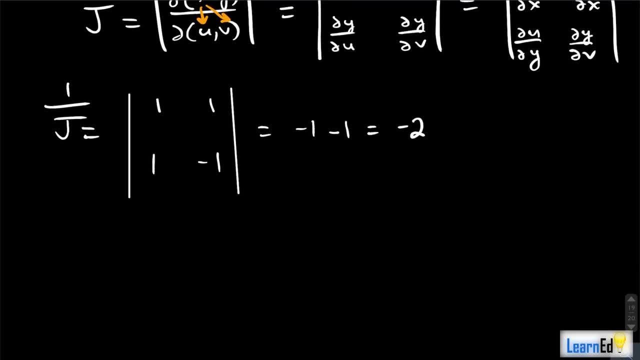 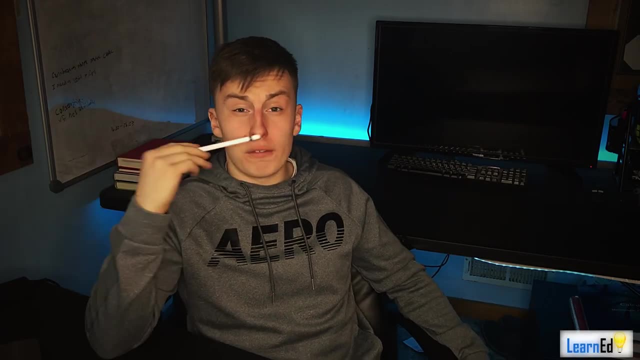 The determinant of this is AD. So negative one minus BC minus one equals negative two. one over the Jacobian is negative one half, So the Jacobian is negative one half. Now, if you want to check my work, you can also solve for X and Y and then compute the. 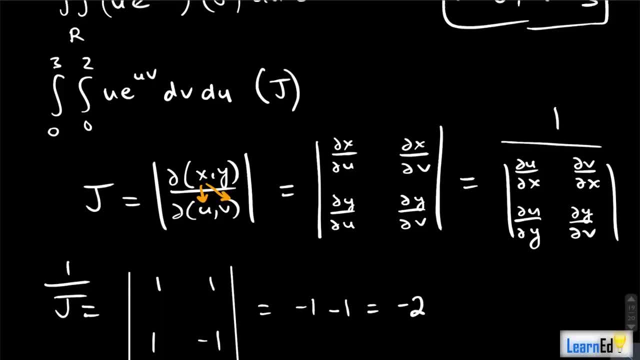 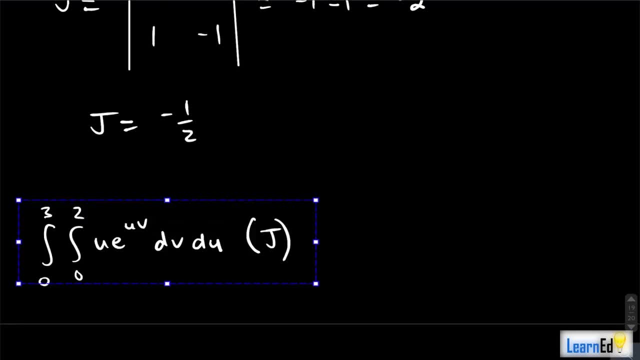 Jacobian. that way You'll see that it also comes out to negative one half. So writing our integral. I'll copy it from up here And what I'll do. instead of having this Jacobian there, I'll just put it outside. 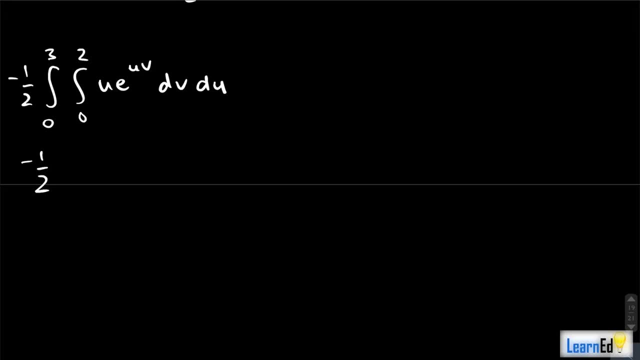 Okay, So we'll have negative one, half The integral from zero to three. We'll have a. we'll integrate this. uh, if we're integrating with this respect to V, we're just going to have a U over U, E to the UV. 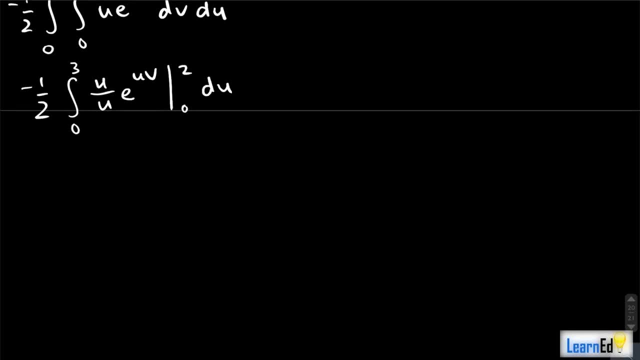 We have this evaluated from zero to two, and then we have DU. So what we get is negative one, half the integral from zero to three, of E to the two U and then minus E to the zero V. Yeah, So we just get one there. 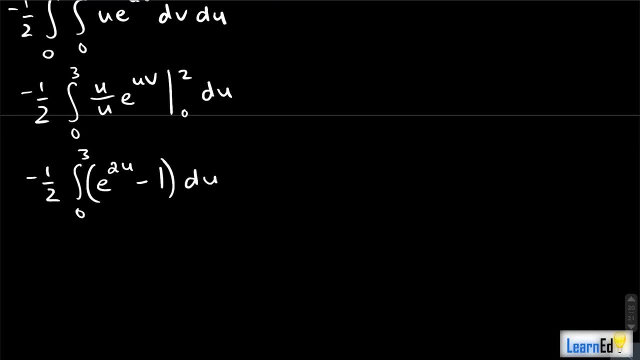 Okay, Okay, So now we can just integrate again: We get E to the two, U over two minus uh- yes, I did that right, Okay, Uh minus U, and we evaluate that from zero to three. So we get negative one half times E to the sixth over two minus a three. 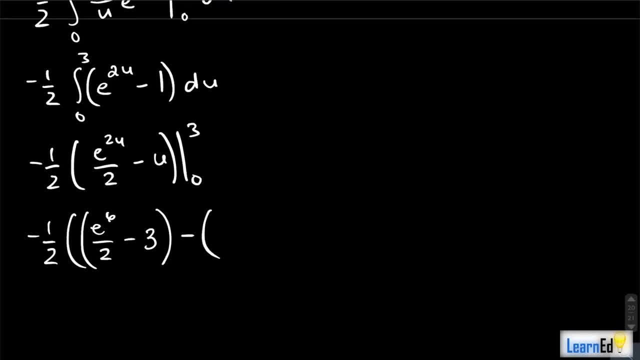 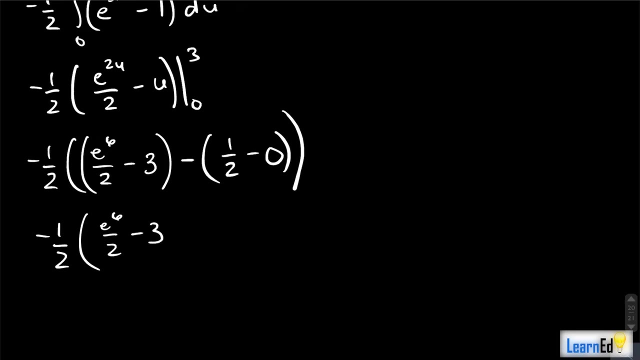 Okay, And this will be minus a. We'll get a E to the zero uh, which will just give us a one half minus zero. So we can simplify this down. We get negative one half uh. E to the sixth over two minus three minus one half negative. 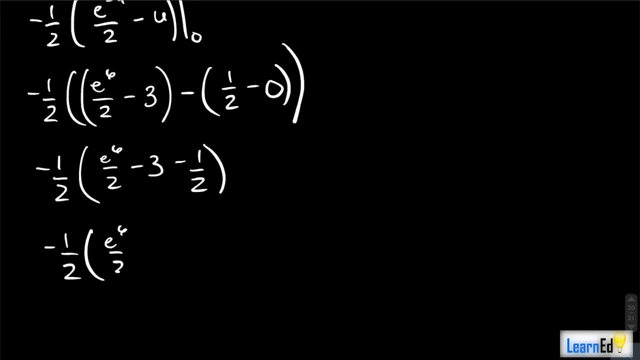 one half, uh E to the sixth over two minus seven halves, And finally we can just say that this is um E to the sixth over four. Okay, Okay, Okay. So you know that we now have our math here and we need to do the math for, uh, you know. 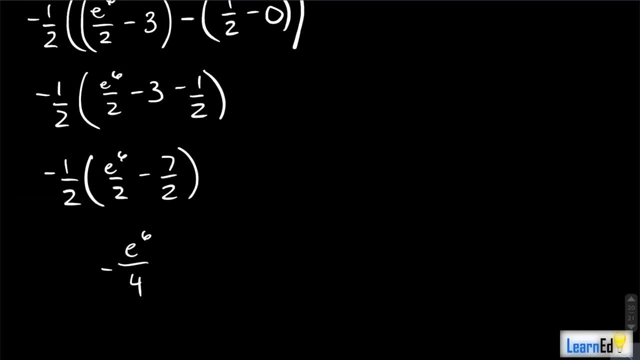 what? Um, I'm going to make this look as nice as possible, since this is the last thing I'm going to write down in this video. uh, let's do that. Yeah, All right, So you know, that's how you do change of variables. 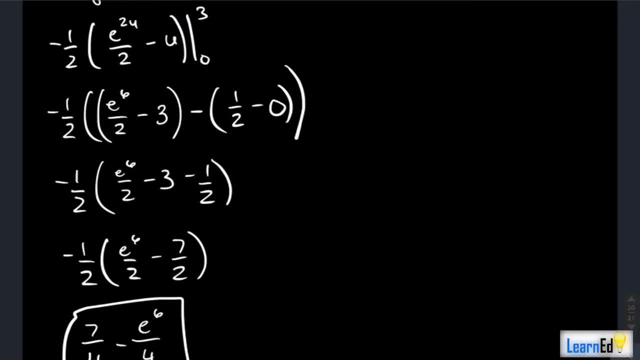 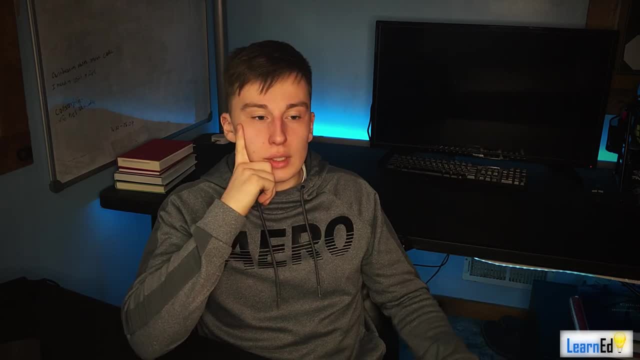 Um, and, and that's really it for multiple integrals. Okay, So you could see, now we're probably at about like an hour hour 10 minutes or something like that. Uh, you know. So I didn't want to add vector calculus to this video. 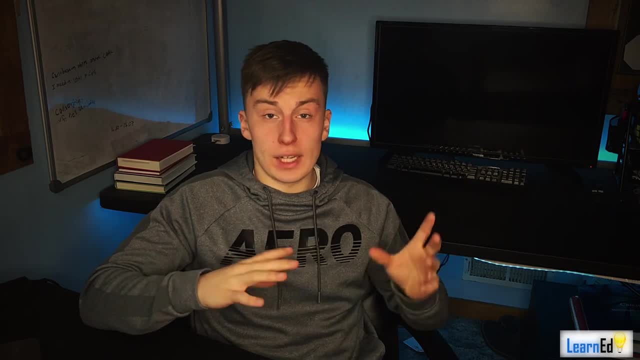 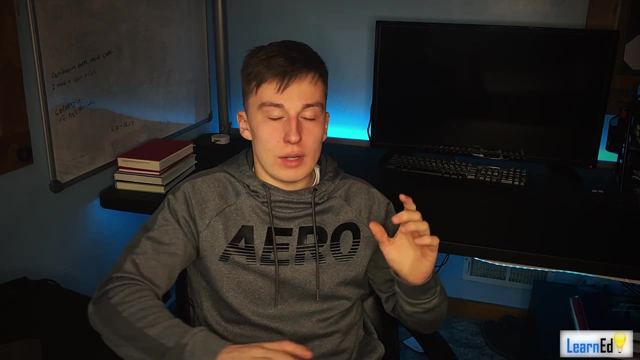 but you know, I hope, you really hope this video really helps you understand multiple integrals and change your variables and all that stuff. because you know double integrals and triple integrals are, You know, not the most straightforward things. You know when you first look at them you know you're like okay.